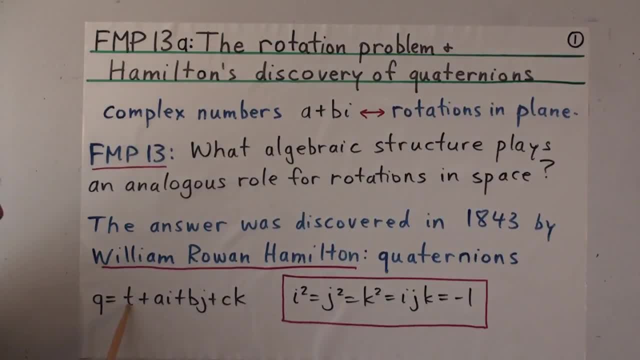 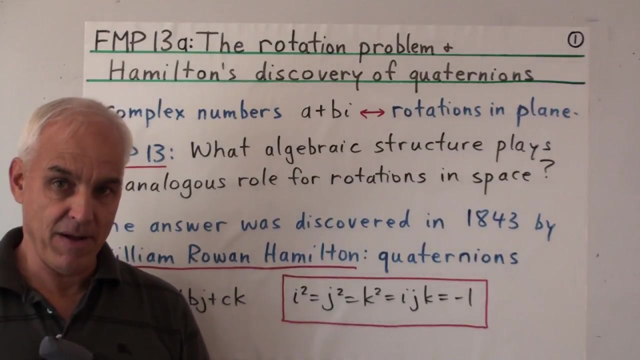 three-dimensional algebra. In other words, he was thinking about vectors of the form t plus ai plus bj- forget the ck for a moment- and trying to find a way of introducing an algebra structure on these three-dimensional vectors, In other words, a way of multiplying them that allowed one to sort of 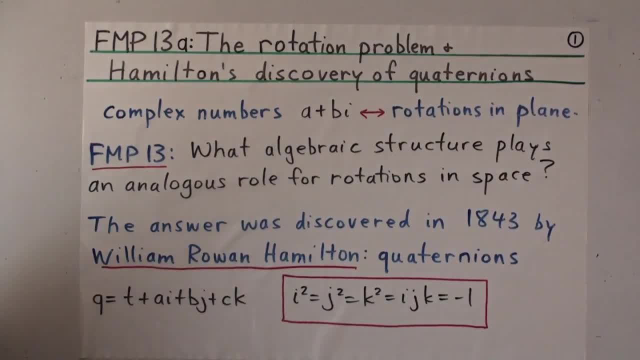 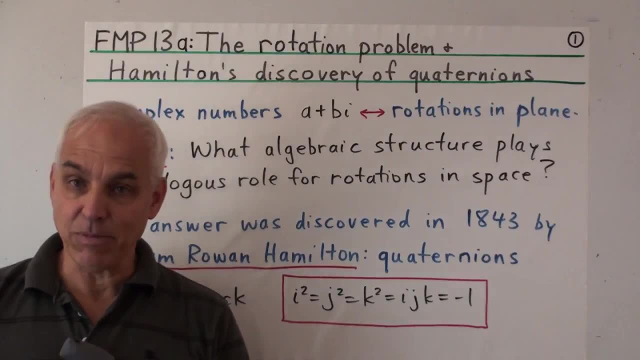 capture the rotational structure of three-dimensional space. And then, on some fateful day in 1843,, he was walking with his wife along a canal in Dublin and was crossing a bridge when this inspiration came to him and he realized that the 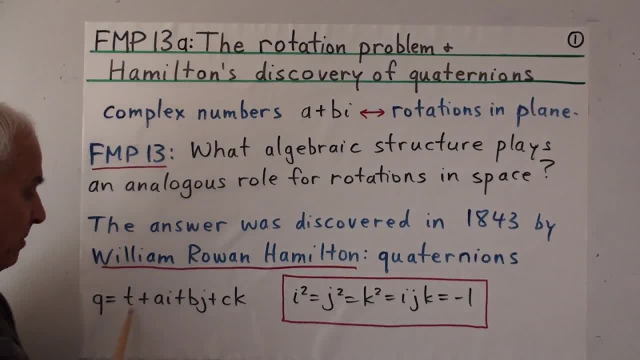 solution was to consider not a three-dimensional space of vectors, but rather a four-dimensional space of vectors, And that the crucial properties satisfied by these new numbers i, j and k- could be captured by these equations. That i squared was equal to minus one. so was j squared. so was k squared. 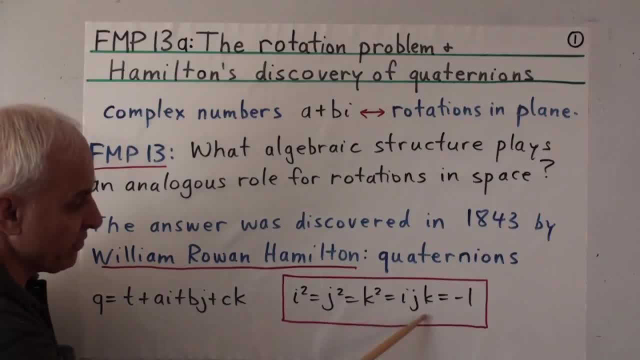 That's much like the complex number situation And in addition, there's a relationship between i, j and k which we can write: i times j times k equals minus one, And he realized this in a flash of insight and a small piece of. 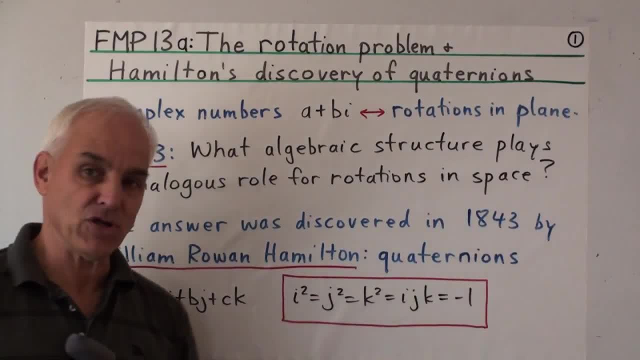 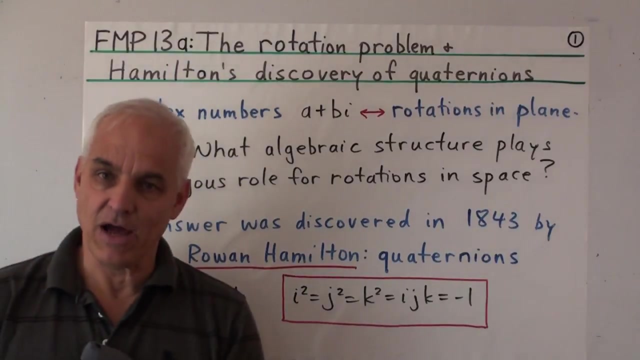 mathematical vandalism carved this equation into the stonework of the bridge. That's a famous mathematical anecdote. a bit of high drama in the world of pure mathematics. William Hamilton was no doubt Ireland's most famous mathematician, a very brilliant fellow who made contributions to 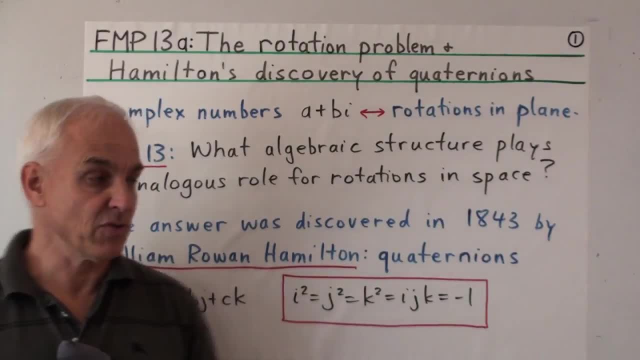 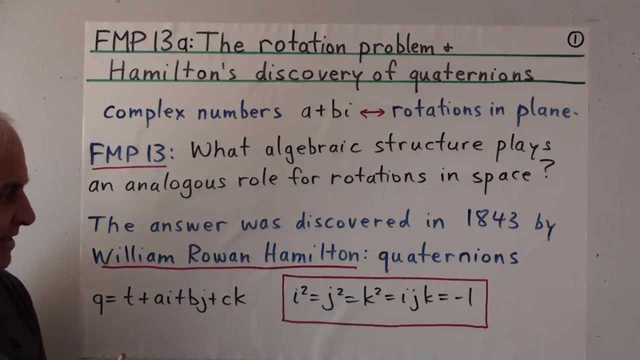 physics, optics and other areas of algebra as well. In addition to his discovery of quaternions, he also built up the theory of quaternions into a very powerful and broad tool for doing physics. That turned out to be coming into conflict with 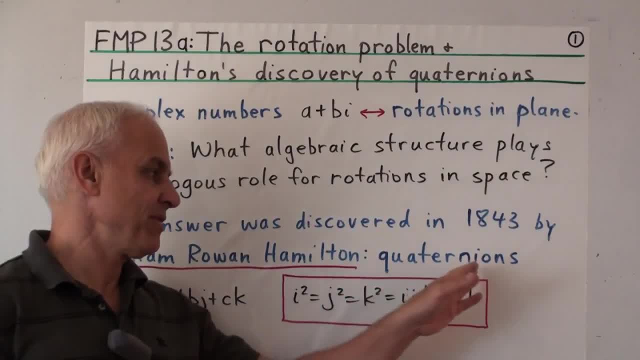 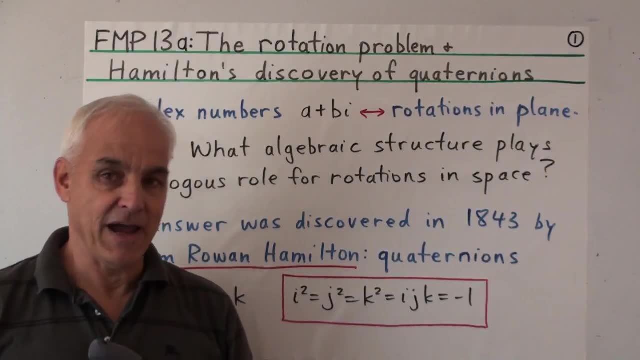 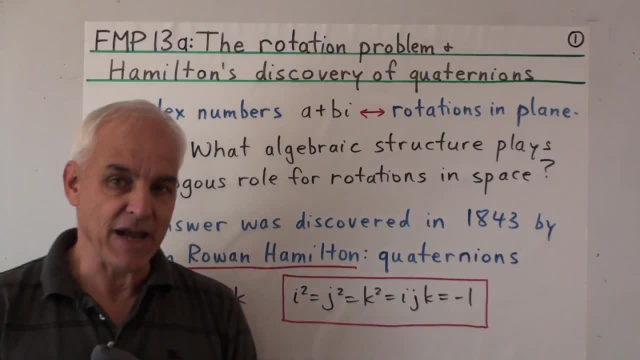 So Hamilton's approach to vectors, and ultimately it lost out to our current approach using dot products and cross products. But as we'll see, they're actually closely connected to quaternions as well. Hamilton was also famous for an important insight into classical mechanics. 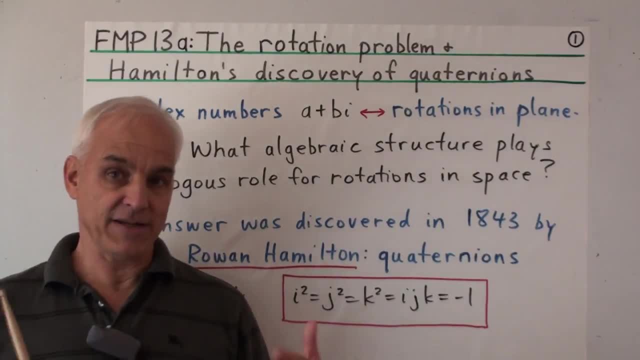 So he took the framework of Lagrange, that Lagrange had established for understanding Newton's laws, and he went back to the and twisted it in an important new direction to give us the so-called Hamiltonian formulation of classical mechanics, which not only brought into being a subject called symplectic geometry, 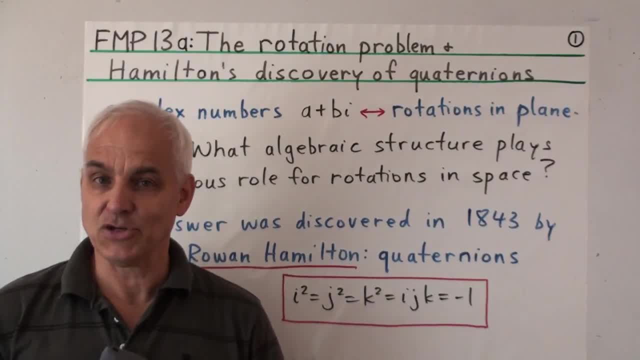 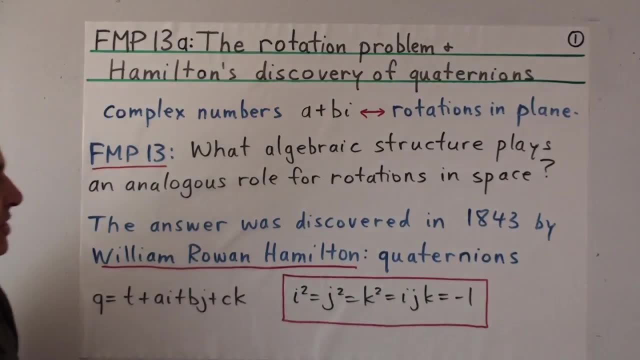 but also was a very important contributor to the 20th century development of quantum mechanics. Alright, so we're going to describe this problem, and it's going to take us probably three lectures to do that. So in today's lecture I want to start by setting the framework. 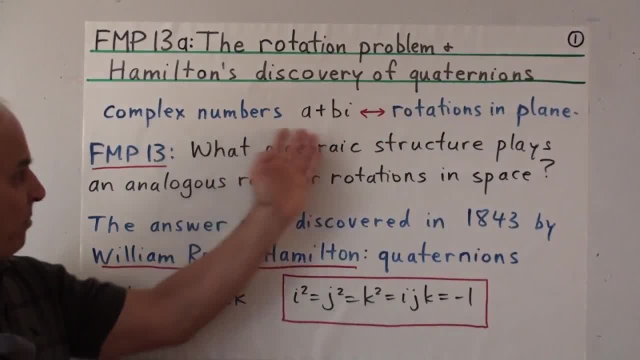 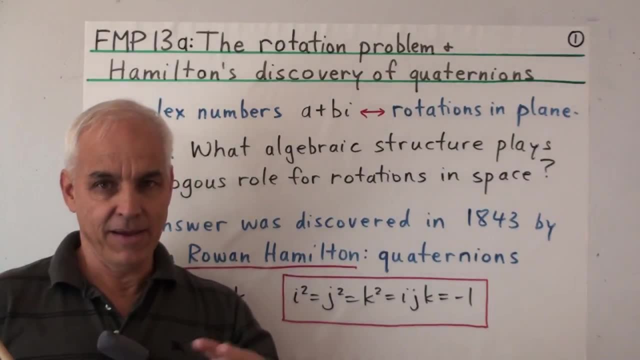 so to speak, by making very clear this connection between complex numbers and rotations in a plane. It turns out that if you look at that subject in the right way, in other words in a rational way, then that makes it much easier to understand what happens with a story. 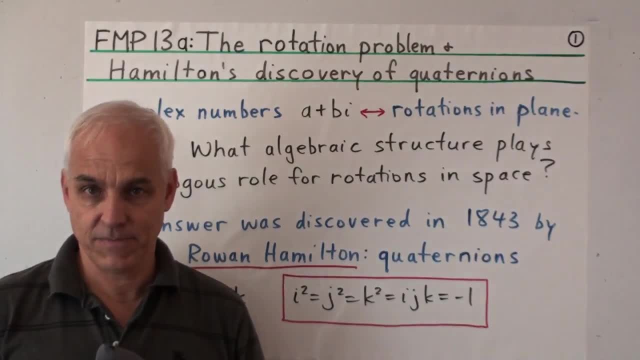 with quaternions and rotations in three-dimensional space. So that's what we're going to do today mostly, and then in the next lecture we're going to talk about rotations And how we think about rotations in three-dimensional space, And then we'll get to the actual quaternion. 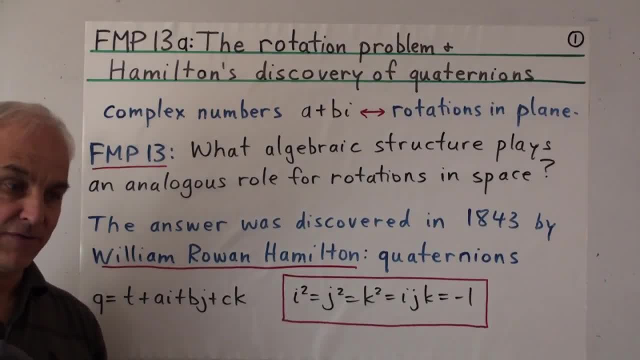 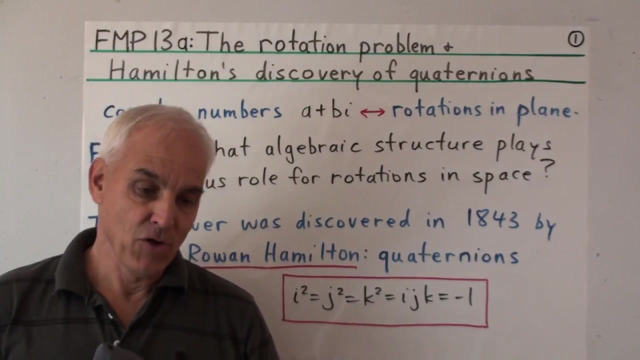 algebra in four dimensions that Hamilton introduced. So we're going to have to go up to four dimensions and understand a little bit of the geometry of four dimensions to get at these quaternions. Now, this is a subject which is quite important these days because working with rotations, 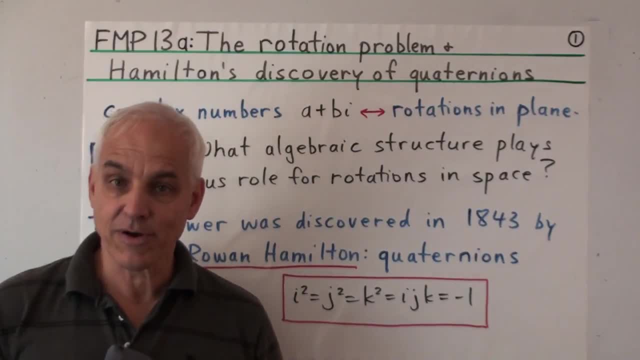 is something that We do a lot in industrial work, in graphics, in computer programming, for example, in video game construction. So there's lots of situations where we want to manipulate rotations effectively And it turns out that quaternions are probably still the best and most efficient way of doing. 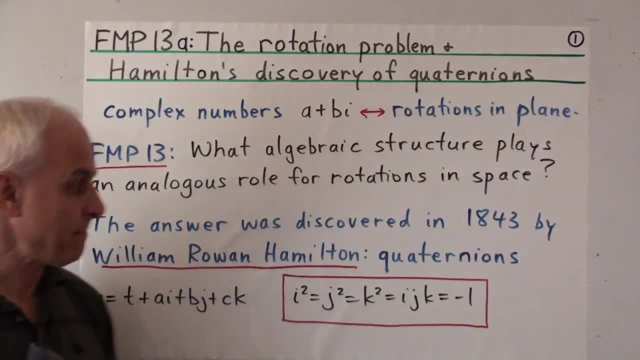 that That's a lovely subject that undergraduates can learn about. So I'm going to give you an introduction to Hamilton's quaternions in these next three lectures, And we're going to start off with this much simpler situation: complex numbers and 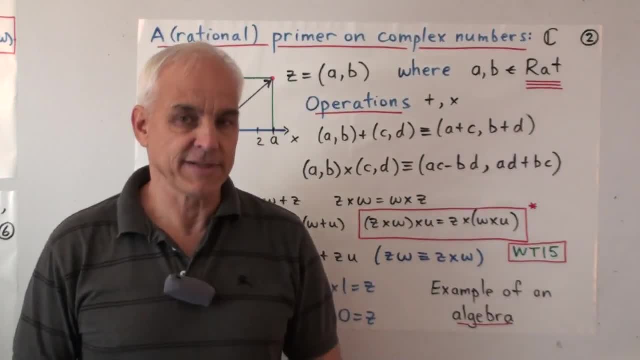 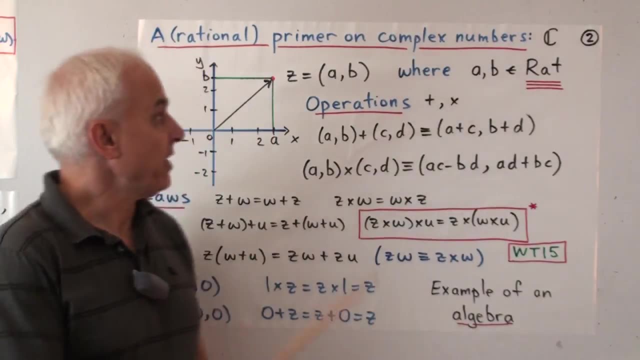 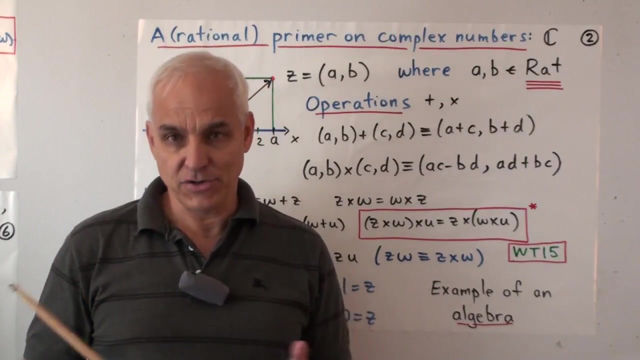 rotations in the plane. There will be a lot of material in this lecture. None of it too sophisticated, But some of it a bit novel, because I have a rational point of view towards things And it turns out that this rational point of view is a very good way of understanding. 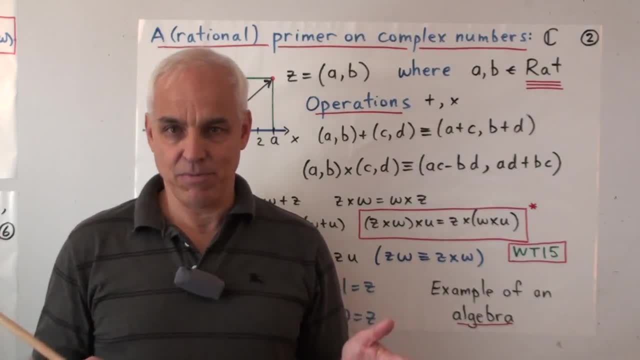 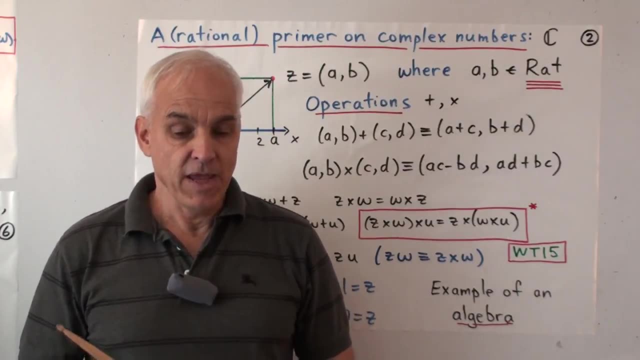 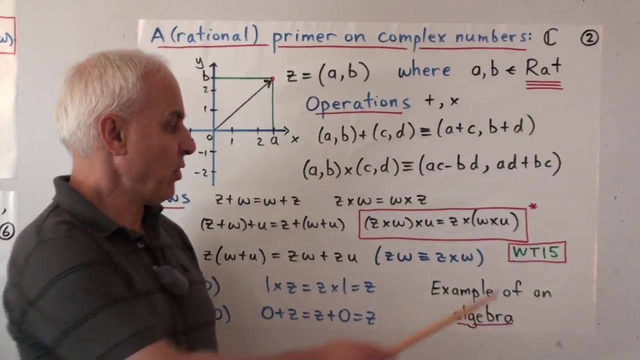 things. It makes a lot of higher geometry much simpler. So even if you're very familiar complex numbers, you are going to learn some important things in today's lecture. If you haven't seen complex numbers before, well, this is probably something of an introduction. You can also have a look at the 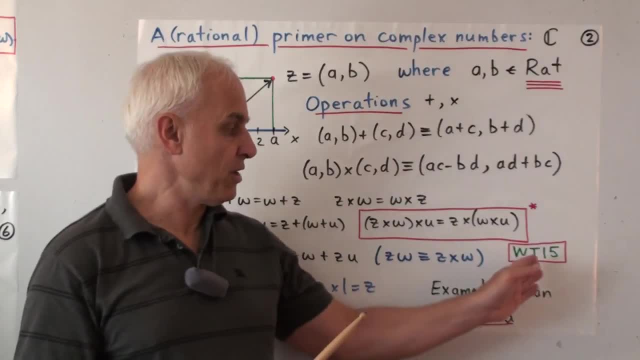 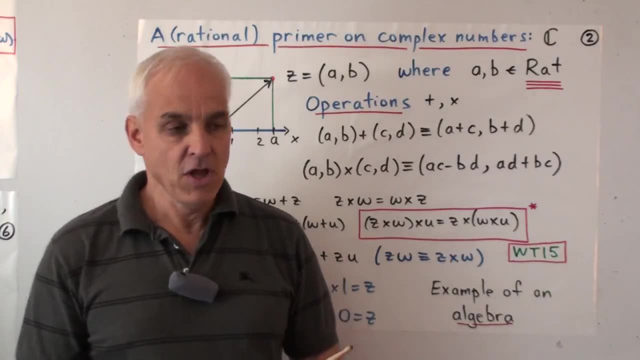 Wild Trig 15 video, which was made quite a few years ago now, but it also has some information on complex numbers. You might want to watch that before you have a look at this. So don't hesitate in stopping the video, going back making sure you understand. 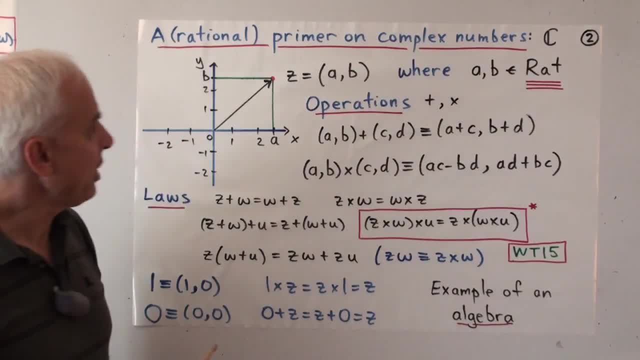 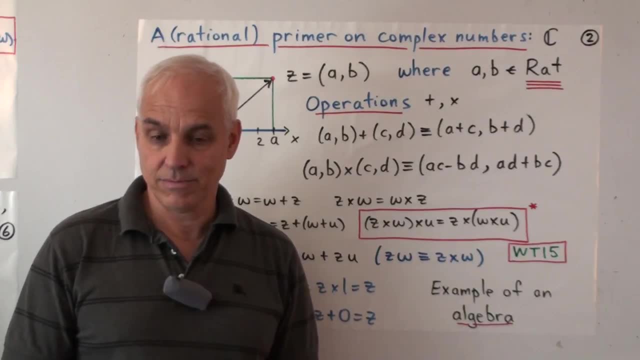 everything that I'm saying here. Alright, we're starting with complex numbers, but I adopt a rational point of view because I don't believe in irrational numbers. It's not a religious position, it's just that I haven't seen any and no one has actually shown me. 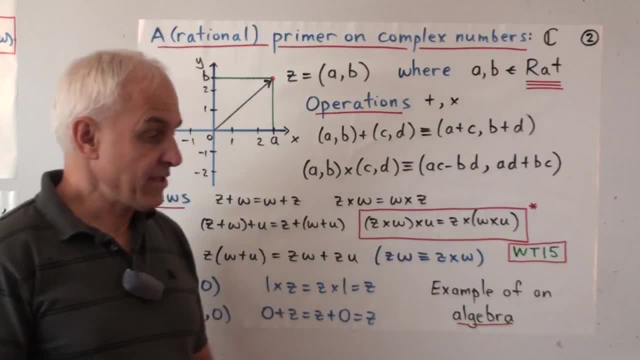 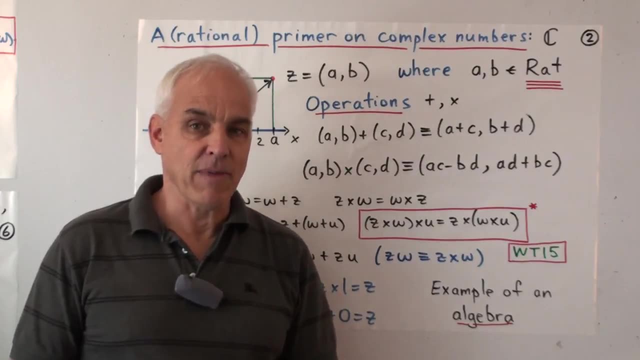 proper irrational numbers, so why should I believe in them? It's a very good position that I encourage you to adopt as well. You might think that it diminishes one's mathematics, but it turns out that it does exactly the opposite: It strengthens one's mathematics because one can then. 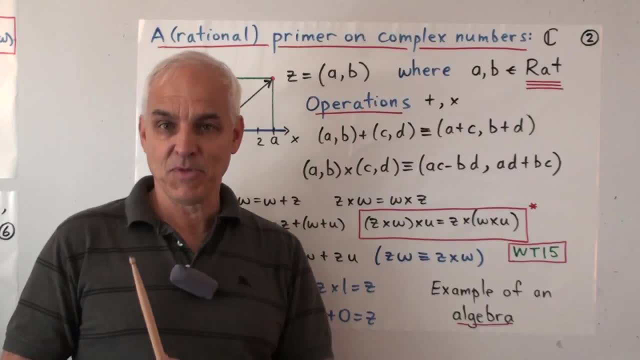 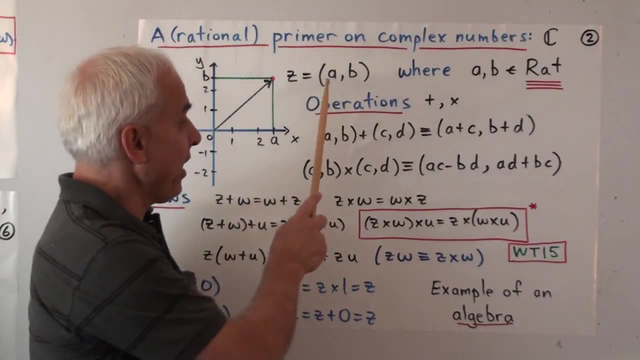 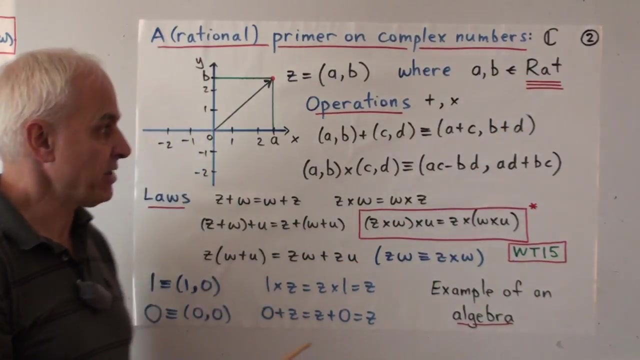 look carefully and clearly and logically at so many things which previously require waffling. So a complex number for us is a pair- a, b- of rational numbers, And this is what I used to denote the type of rational numbers. I prefer not to think in terms of infinite sets. 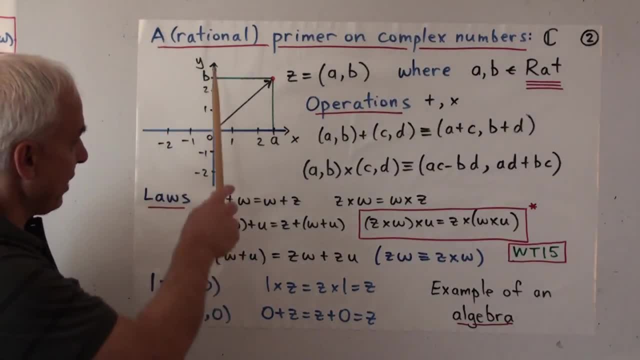 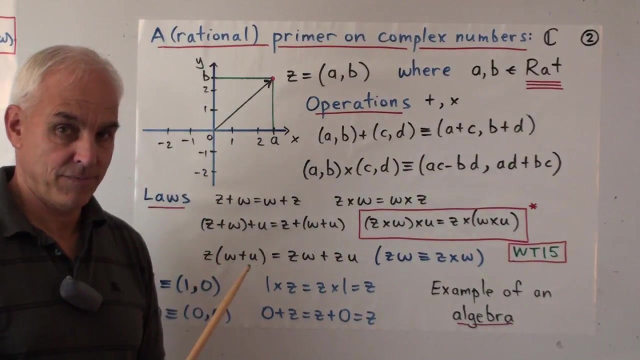 Pictorially we have a xy plane. The pair a- b can be thought of as this point here, with x coordinate a, y coordinate b. Or it can also be thought of as the vector from the origin to this point, And sometimes it's best to think: 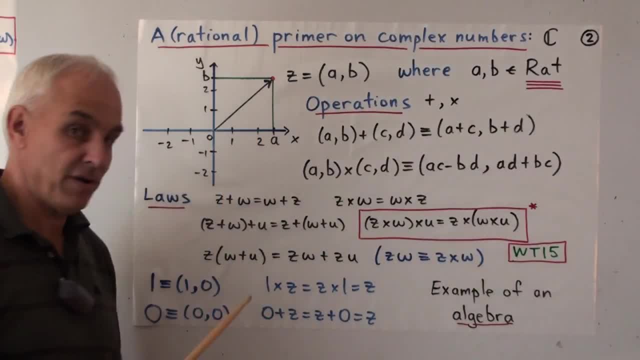 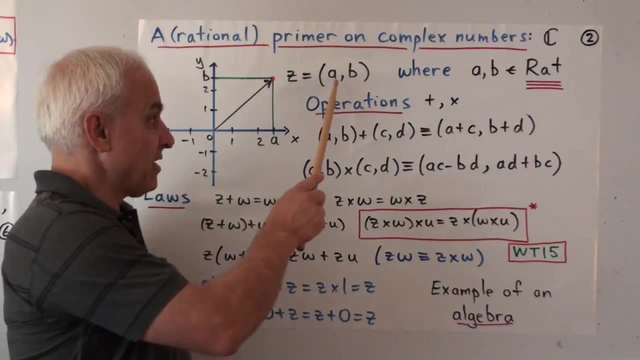 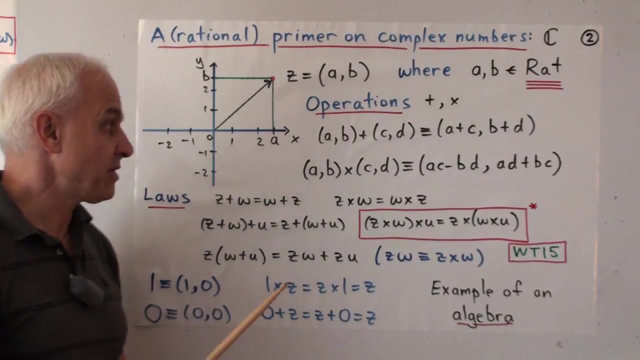 in terms of a point, and sometimes it's better to think in terms of a vector. But in fact, logically speaking, the complex number is neither of those. It's just the pair of rational numbers. Complex numbers support operations. Actually, they support all four operations of addition. 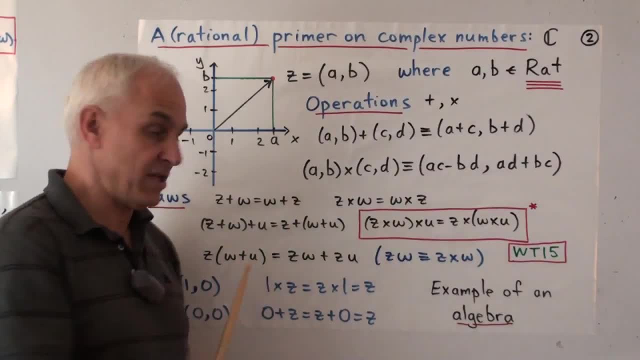 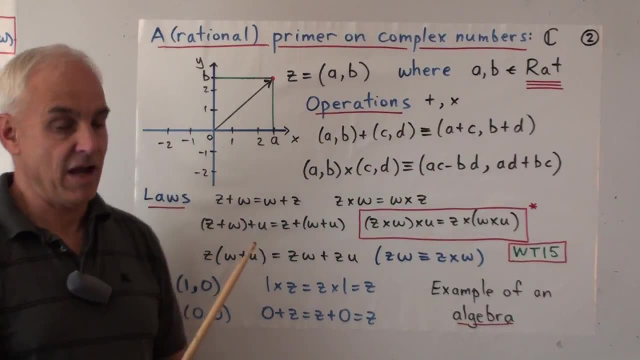 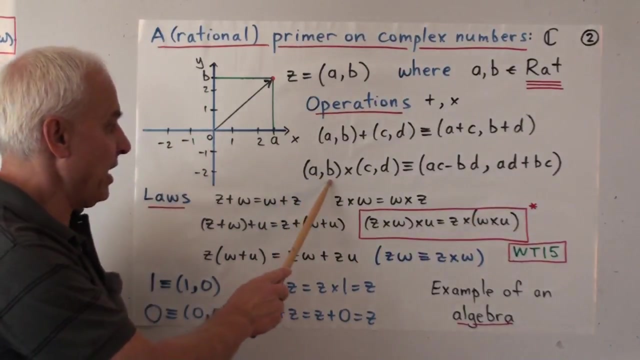 multiplication, subtraction and division. But here are the two main ones of addition and multiplication. Addition is point-wise, corresponding to the usual vector sum of vectors. The multiplication is where all the interest lies. So the formula is that a b times c d is. 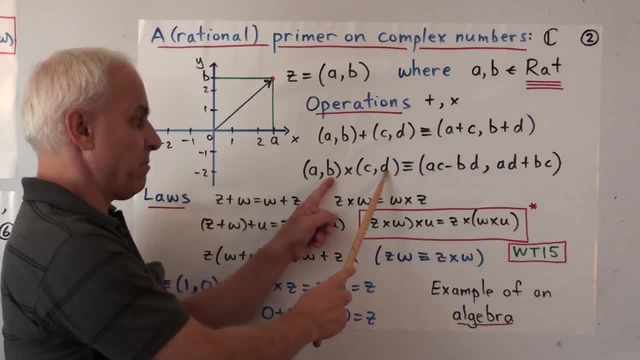 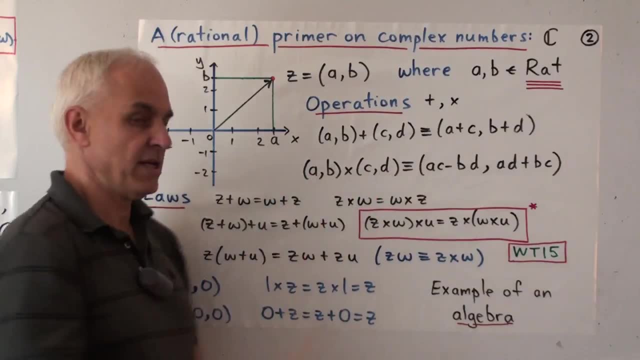 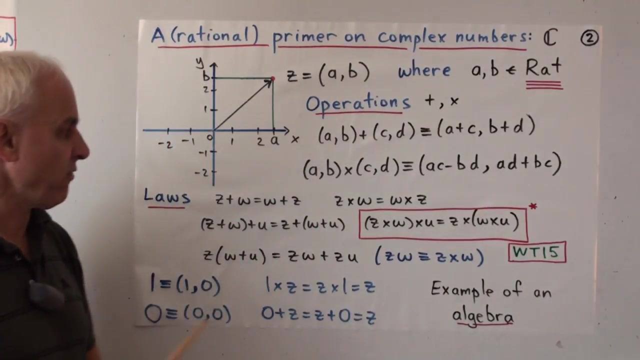 my definition: a times c minus b times d. that's the first entry, And then the second entry is a times d plus b times c. So we make the definition. That's just how we're going to define multiplication of these ordered pairs of rational numbers. 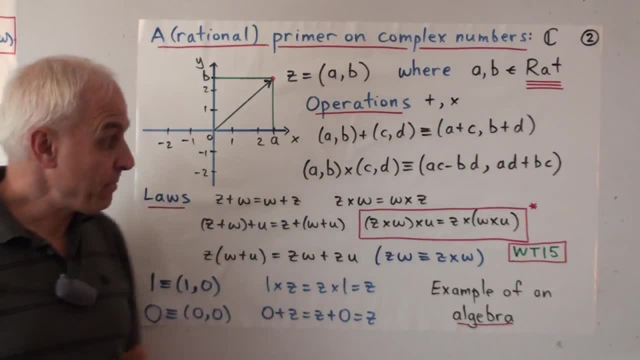 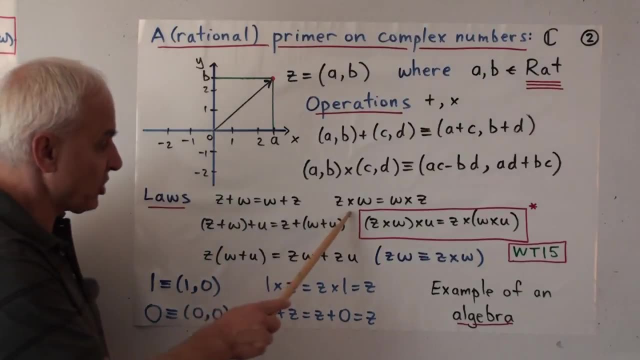 And it turns out that's a very good choice because it has lovely properties. Namely, these operations satisfy the following familiar laws of arithmetic. First of all, the two operations are commutative: z plus w equals w plus z and z times w equals w times z. 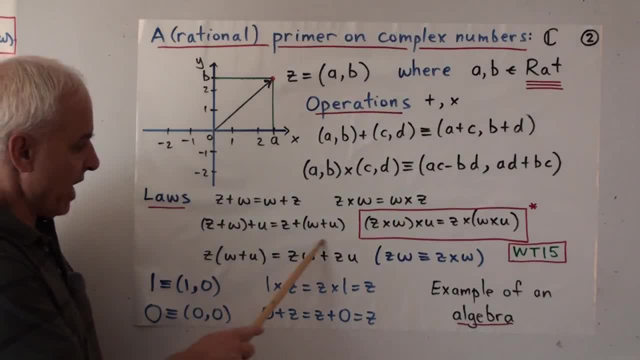 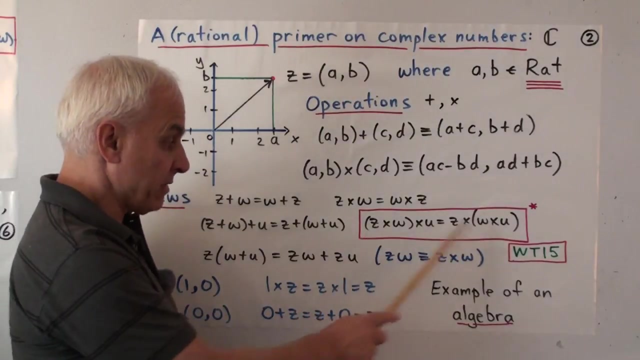 Please check that We have associativity, That is, if you have three complex numbers, it doesn't matter in what order we pair them. So z plus w plus u is the same as z plus w plus u And, more importantly, for multiplication as well, z times w. 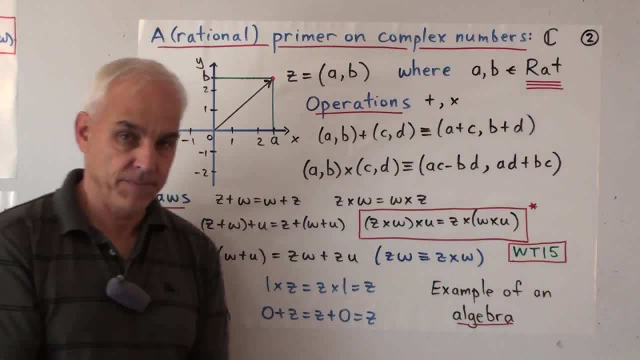 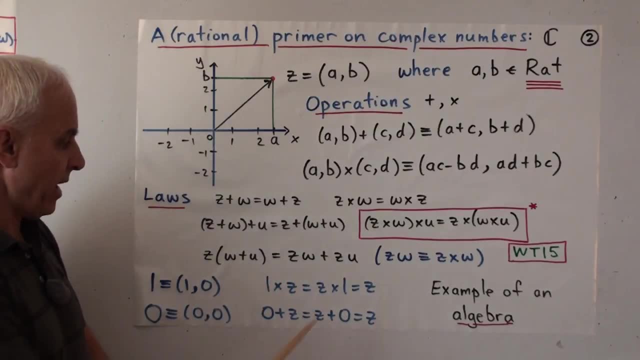 times u is the same as z times w times u. Then there's a distributive law: z times w plus u equals z w plus z u, And here I'm allowing myself the shortcut: z w means z times w. These laws are relatively straightforward to verify, except perhaps for this one. 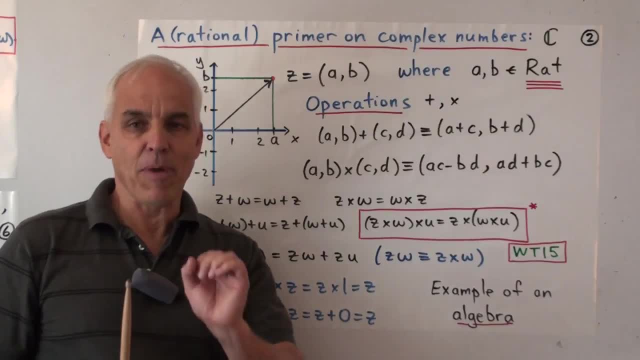 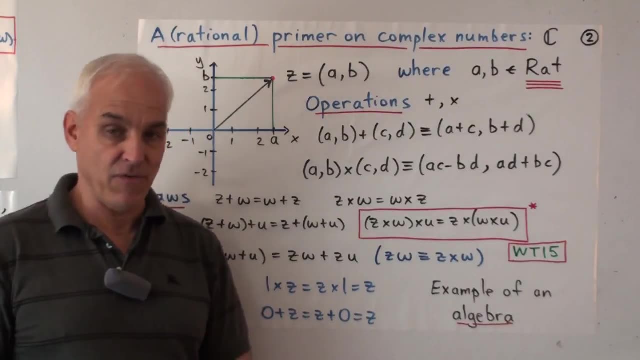 This is the most interesting one: The associativity of the multiplication. That turns out to be somewhat non-trivial. You actually have to make a calculation for that And I please urge you, if you haven't done this in your mathematical career yet, make this. 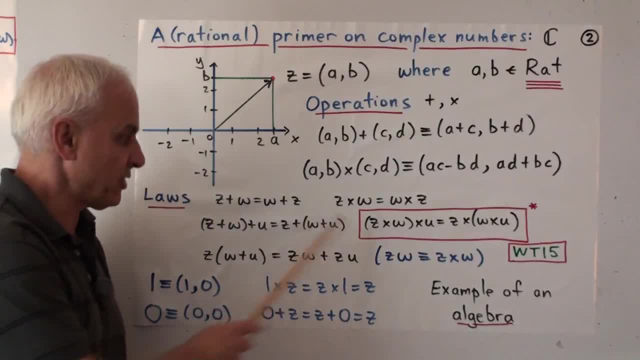 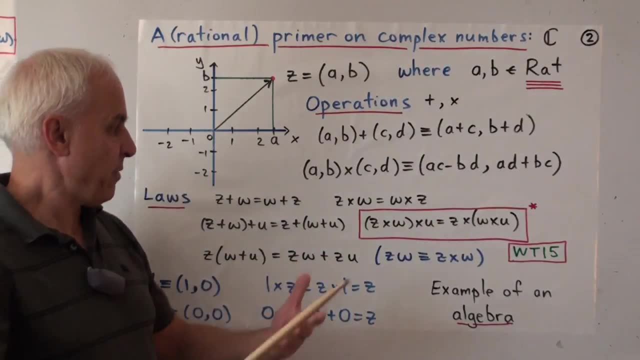 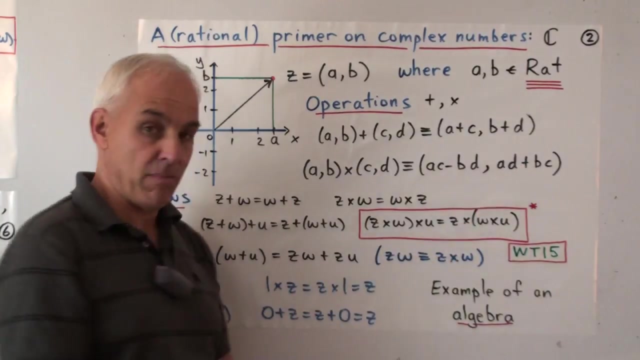 calculation. Check that this is true. And then you might like to think: well, what happens if we modify this definition a little bit? Suppose we decide to make a new multiplication by changing that minus sign to a plus sign, Or maybe that plus sign into a minus sign, Or maybe sticking a factor? 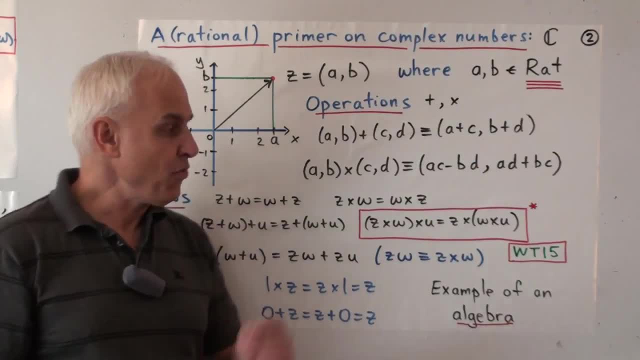 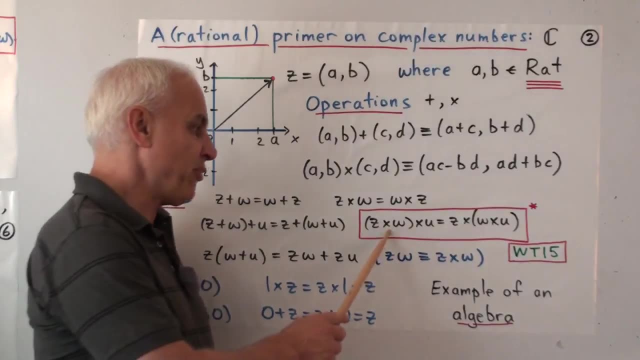 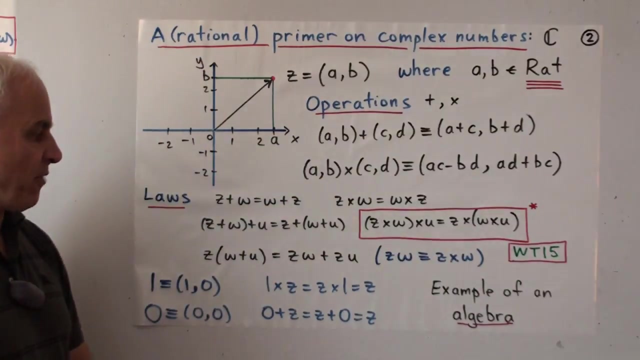 of 2 in front of the ad or some other variant like that. You will find that then this multiplication property here tends to not be satisfied. So you'll get an appreciation for the beauty of this particular definition. It just happens to work for that associative property. 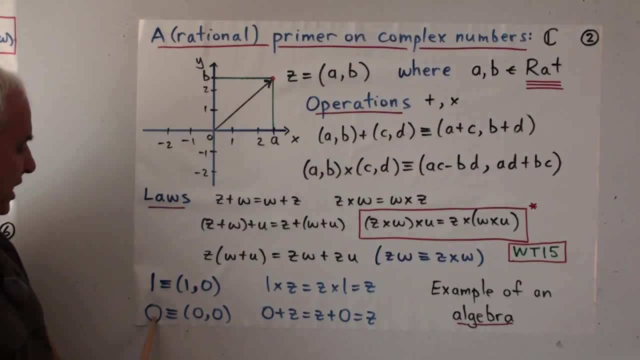 We'll also define a few special complex numbers. So 0 is just the pair 0, 0. And 1 is the pair 1, 0. And then you can check that this 1 has the property that 1 times z is z times 1 is z, So it's the multiplicative identity. 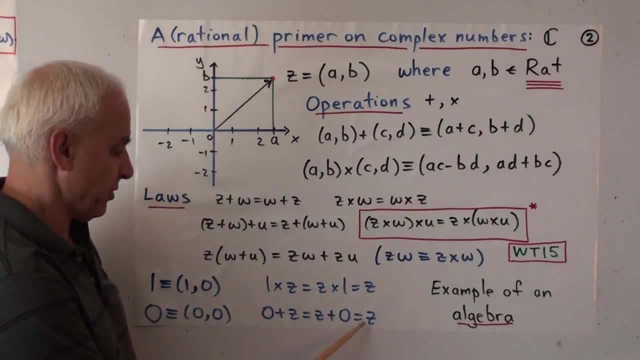 And this 0 has the property that 0 plus z equals z plus 0 equals z. Okay, so we can also define subtraction and division, but I'm not going to do that. This is the essence of the algebraic structure of the complex. 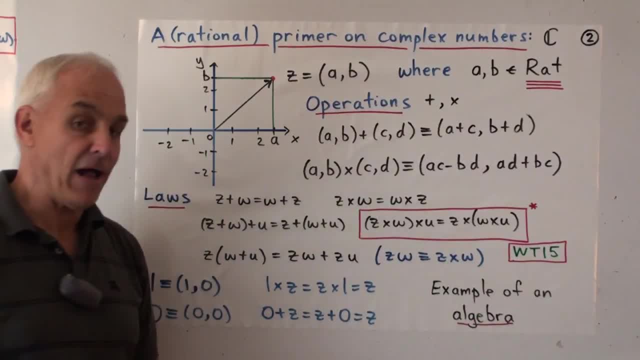 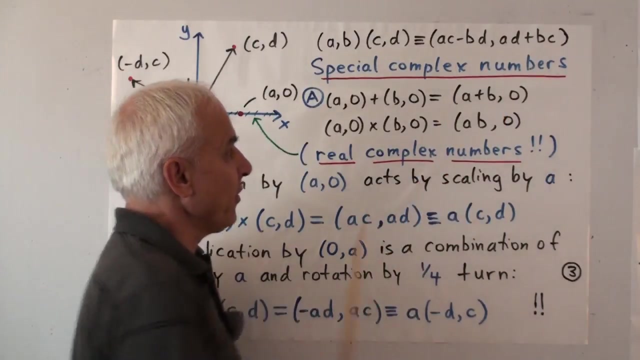 numbers, And this is an example of what is called an algebra in mathematics- A little bit of an unfortunate name because algebra has these different meanings, but anyway, That's the complex numbers. I've now repeated the multiplication here so we can refer to it, And I now want to point out that there are 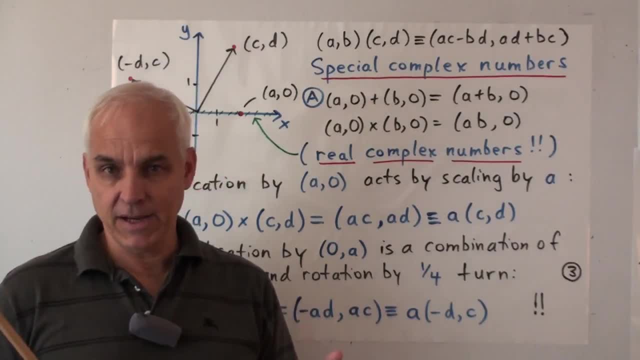 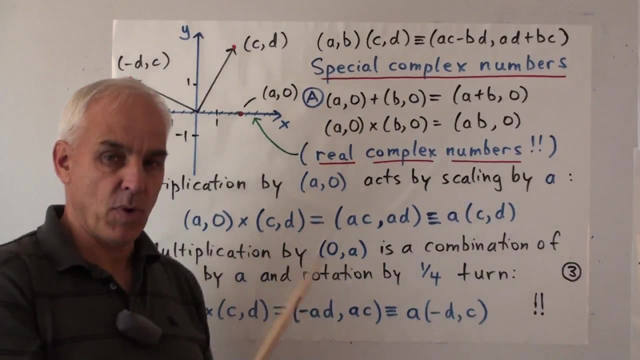 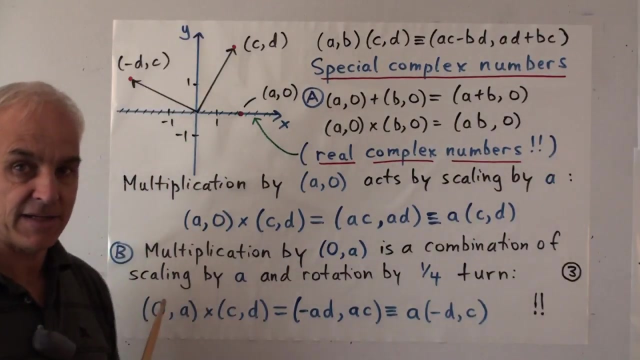 some other sort of special complex numbers that play distinguished roles. First of all, the numbers of the form a comma 0, where the second coefficient is 0. Those numbers correspond to points on the x-axis And their arithmetic is particularly simple. You can check that additively. a 0 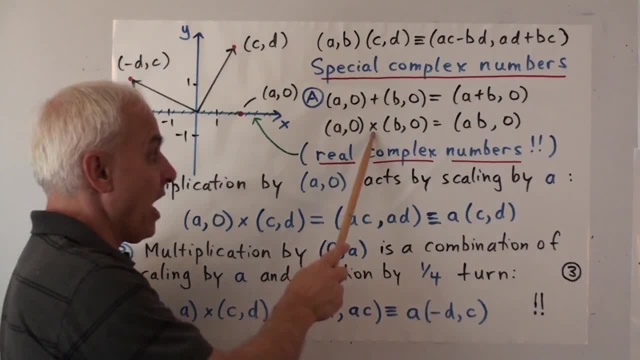 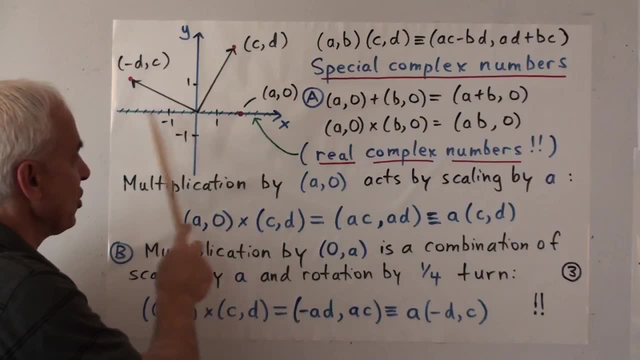 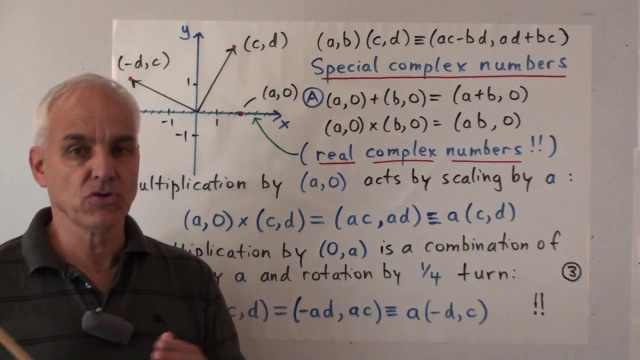 plus b 0 is just a plus b 0. And a 0 times b 0 multiplicatively we get the product a b 0. So that if we restrict our attention to this real axis, then the complex numbers there act just like the usual rational numbers. So we can. 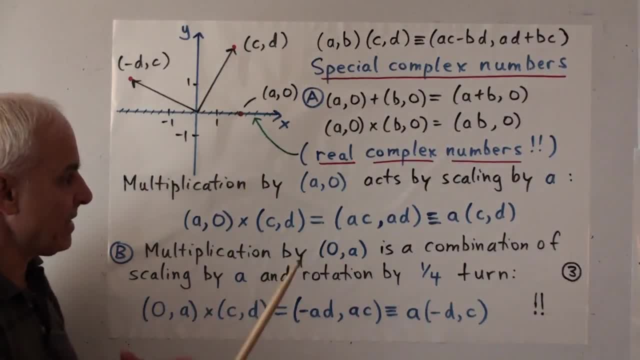 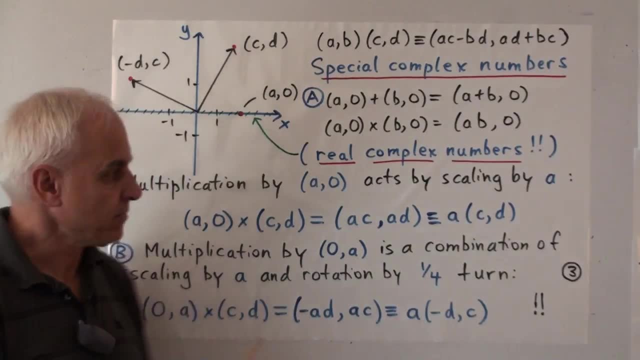 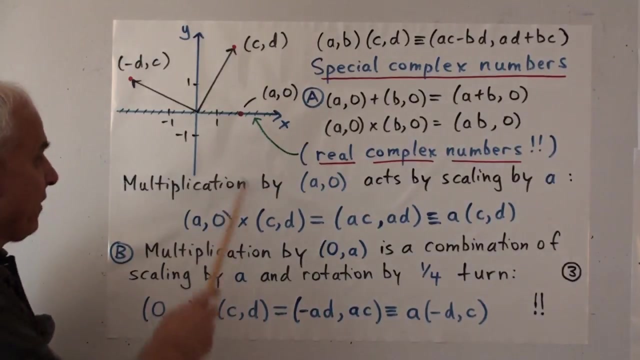 think of the ordinary rational numbers as being embedded in our picture in terms of the points on the x-axis. Now multiplication by such a real complex number. so often these ones are called the real complex numbers, Which is possibly a source of confusion, because I don't believe in real numbers in the usual sense. 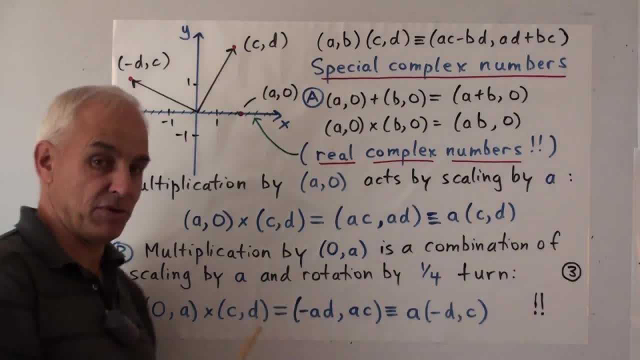 But that shouldn't prevent me from being able to use the adjective real. And so here we're just going to say that any complex number whose second coordinate is 0, we're going to call that a real complex number, even though in fact the entry a is actually a rational number. 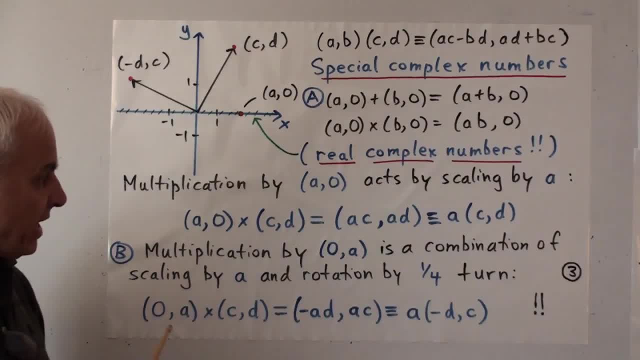 So if we multiply by such a real complex number, a comma 0, then we see that it acts by scaling by a. So let's check: If we multiply a 0 by c- d, the rule is we take a times c minus 0 times d, So that's just a times c. 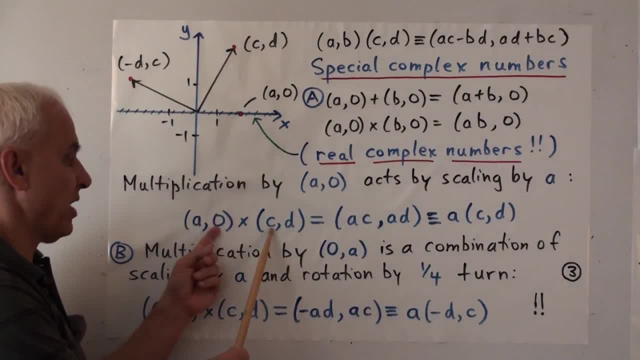 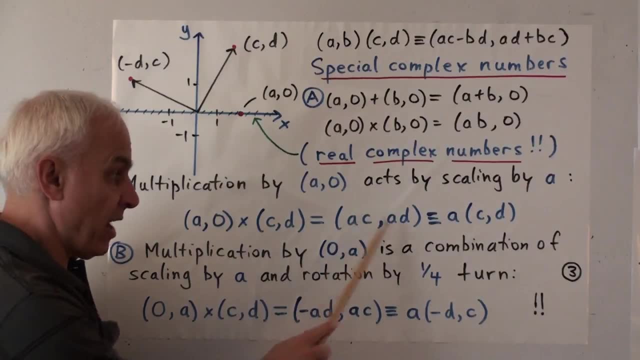 And then we get a times d plus 0 times c, So that's just a times d. So what has happened is that each of these entries has gotten multiplied by a, And a is just an ordinary rational number, And let's agree that we use a sort of vector space. 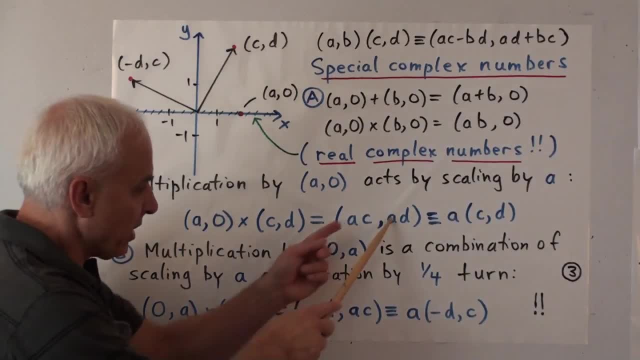 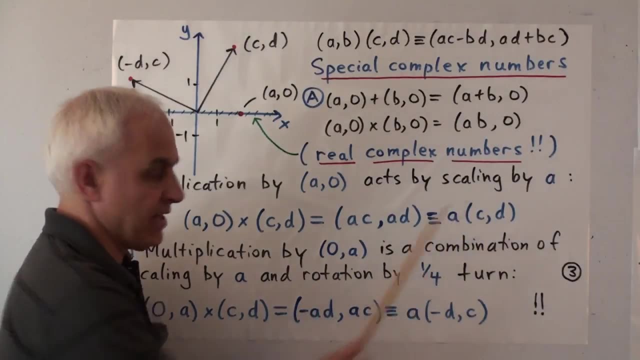 terminology here, or notation, and agree that we can pull that a out front if it's common to both terms, And so we can rewrite this as a times c, d. So here the a is just a rational number. We're just talking about scaling. 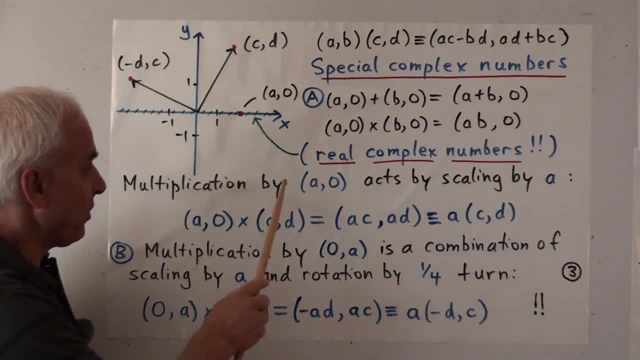 the vector by multiplying by a. So that's what happens when we multiply any complex number by a 0.. For example, if we multiply that complex number by a 0,- a here is somewhere between 1 and 2, say- then it would mean that this vector 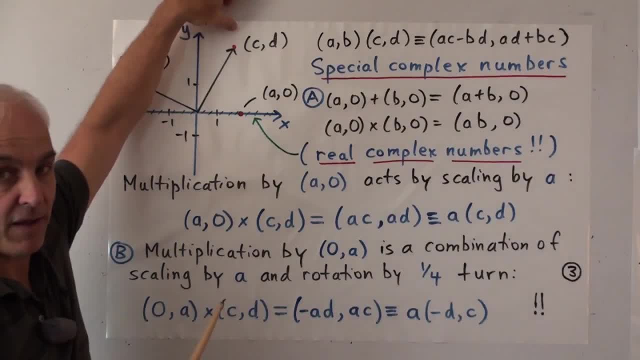 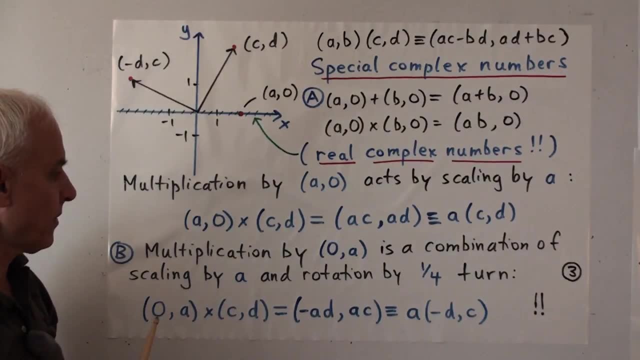 would enlarge by a factor of a, So it would become roughly twice as long. So the product would be up there somewhere. On the other hand, it's also interesting to consider complex numbers which lie on the y-axis. They also have a distinguished role. 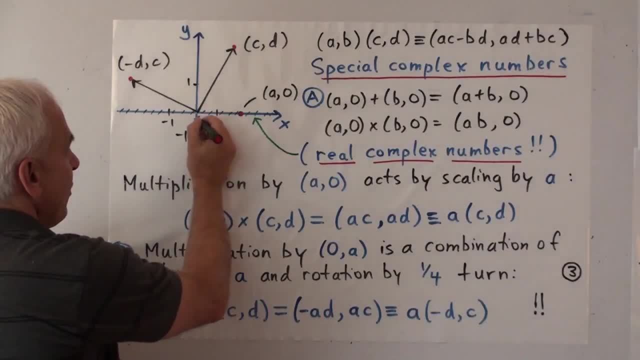 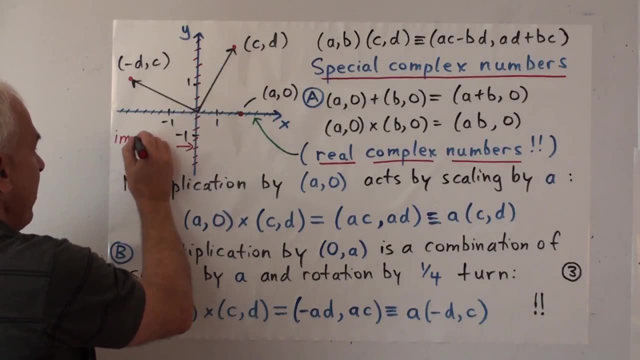 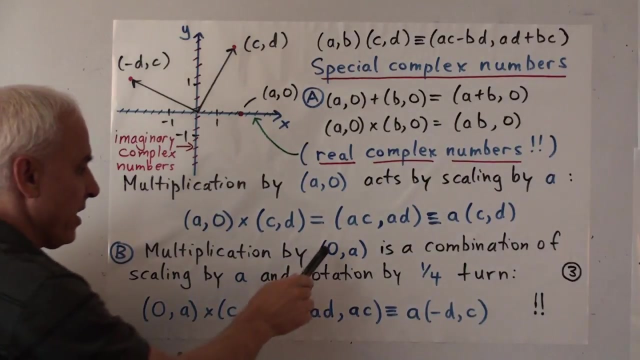 And let's put them in. So these are sometimes called- well, they're called imaginary complex numbers. Imaginary complex numbers, The ones that are lying on the y-axis. They have the form 0, a. So what happens if we multiply by 0, a? Have a look. 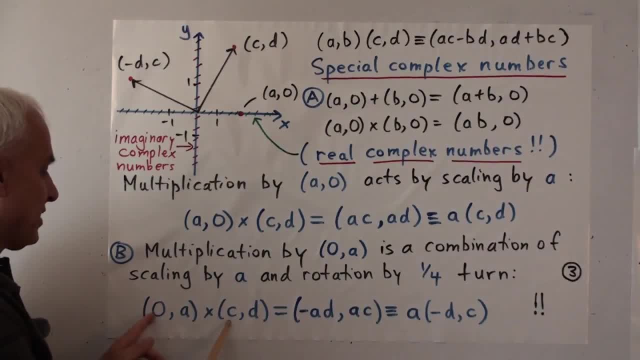 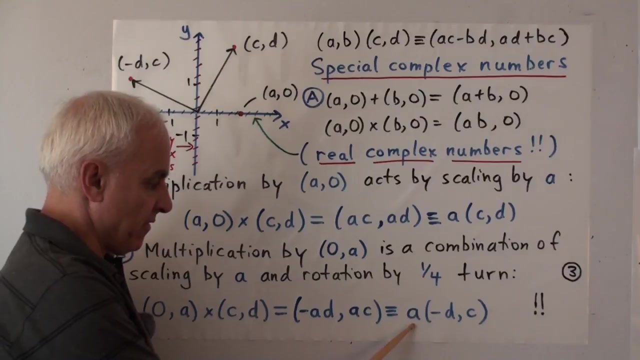 Here's our basic law for multiplication. So we get 0 times c minus a times d for a total of minus a times d. And the second entry is 0 times d plus a times c or ac. If we pull out the common a, as we did before, then this is a times. 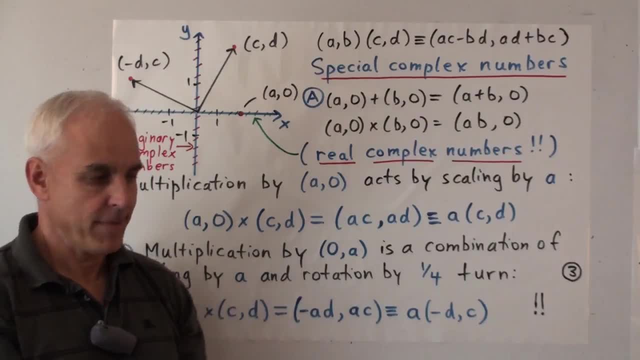 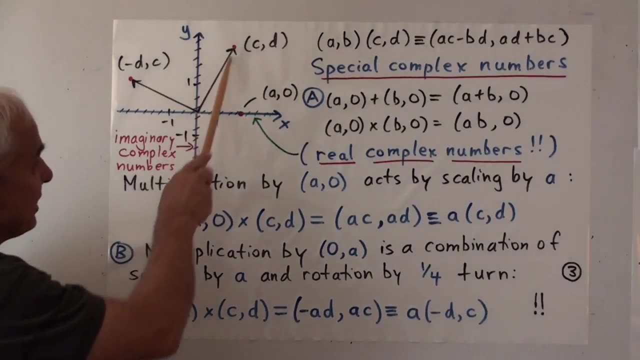 minus d c. So what's the relationship between minus d c and c d? Well, if here is c d, then here is minus d c. It's really the same vector, except that it's been rotated by a quarter turn, So a quarter of the way, all the way around. 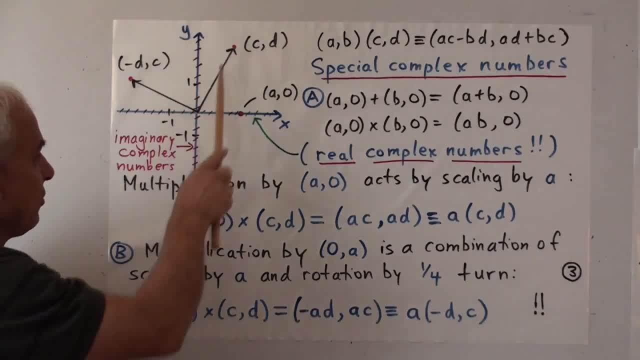 That's a right angle there. These two vectors are c's if we're measuring an angle Spread of 1, if we're measuring with rational trigonometry. So the effect of multiplying by 0, a is to take this vector, multiply it. 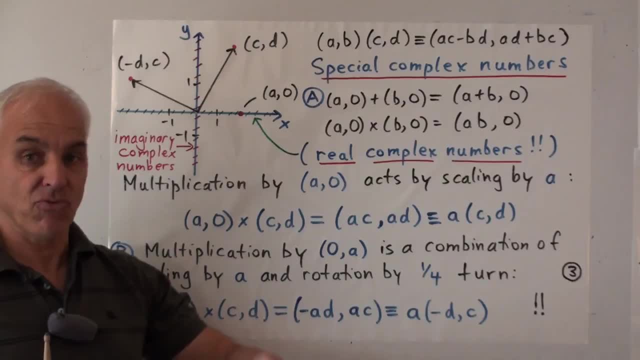 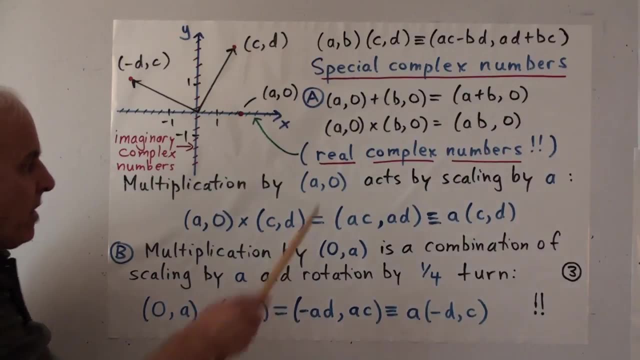 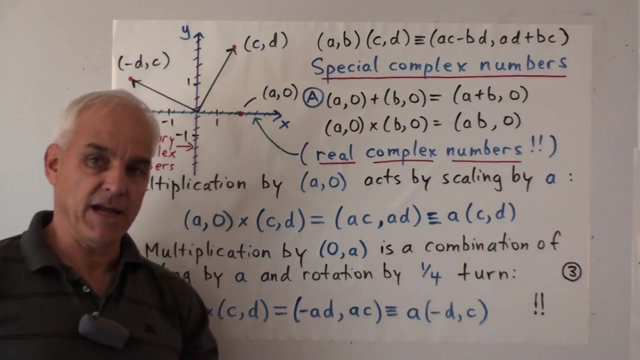 scale it by a and rotate it by a quarter turn. So multiplying by a, 0 just dilates. but multiplying by 0, a dilates and rotates by a quarter turn. So we're already seeing some geometry, some geometrical transformation. 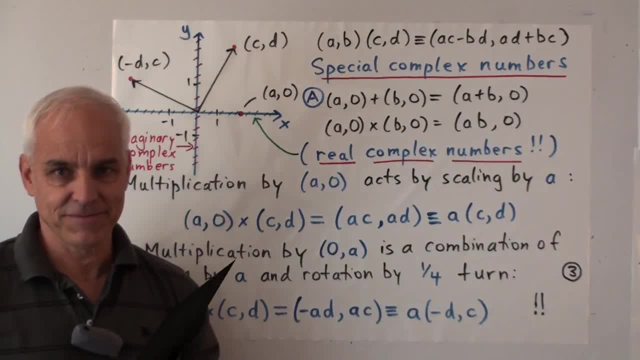 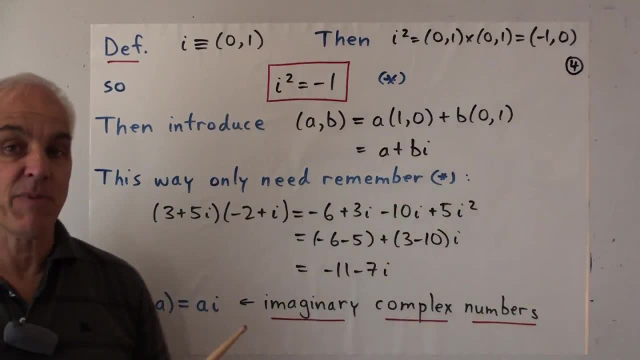 associated to the algebraic structure. So the complex number which is on the y-axis and has coordinate 1, 0, 1, has a special role in the subject And it's usually given a special name. So that's the complex number i. 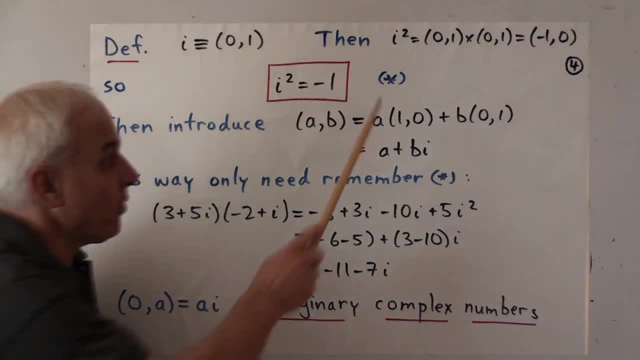 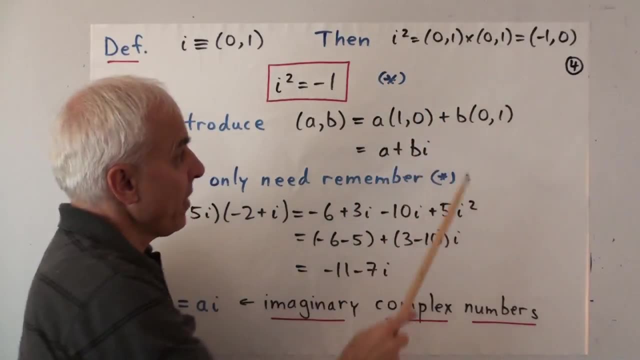 And it's interesting because when we square it, let's see what happens. i squared is equal to 0, 1 times 0, 1.. We're going to get 0 times 0 minus 1 times 1, so that's minus 1.. And we're going to get 0 times. 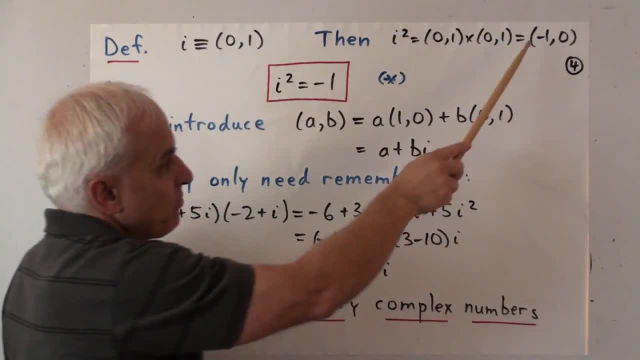 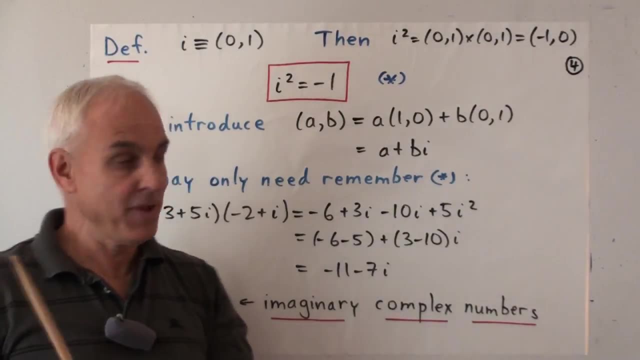 1 plus 1 times 0, so that's 0. So we're getting this number minus 1, 0, which is really like the number, the rational number minus 1.. Because we've said that the numbers ending in 0 are really acting like the rational. 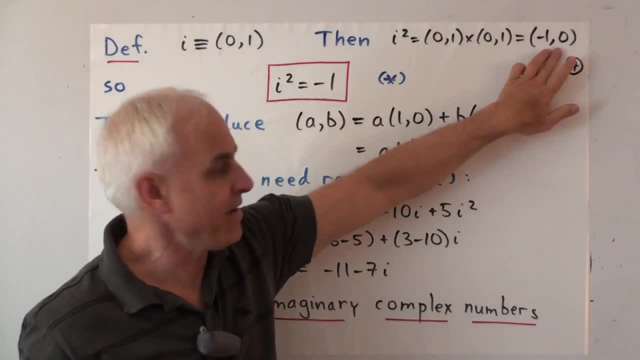 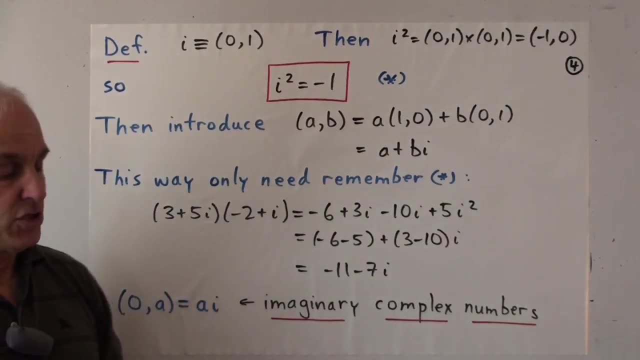 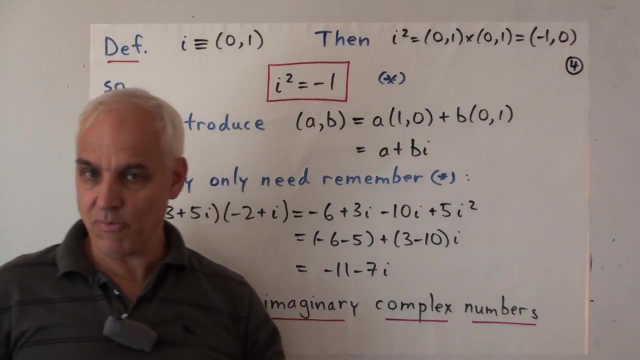 numbers. So we can agree that we're going to call this number just minus 1.. In that case i squared is equal to minus 1.. So we have this algebraic system now, where we have this new number called i, which has this remarkable property that no rational number does. 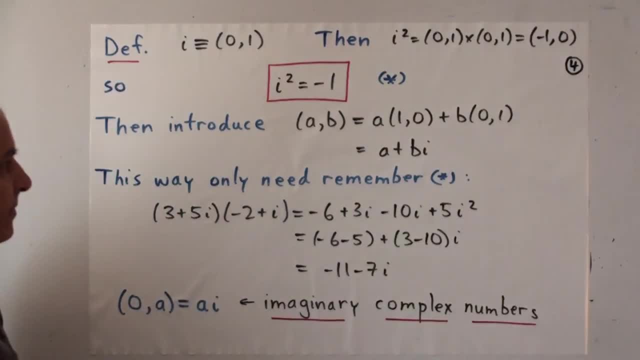 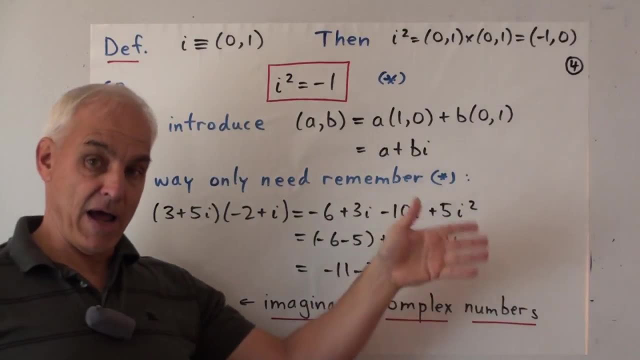 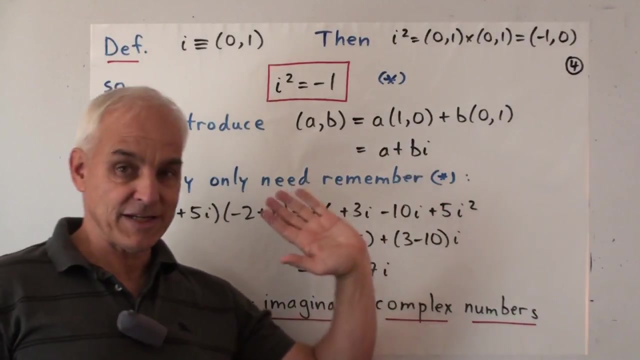 Namely its square is minus 1.. And we can see that, geometrically, from what we were just saying, in terms of rotation, if we multiply by i, well then we just rotate by 90 degrees or a quarter turn. And so if we do that twice, if we multiply by i, squared. 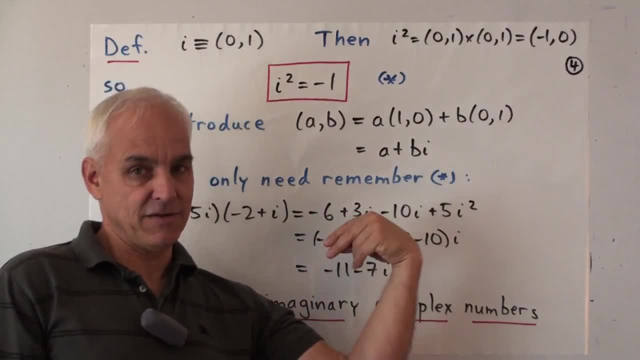 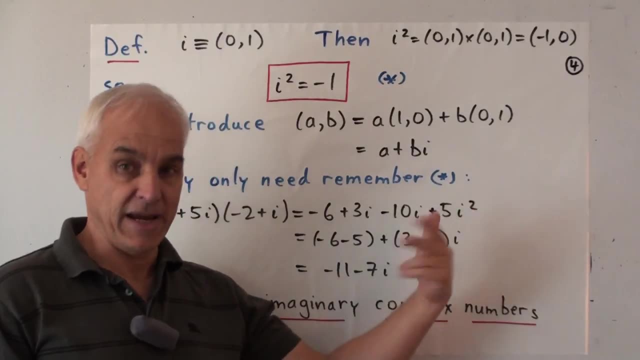 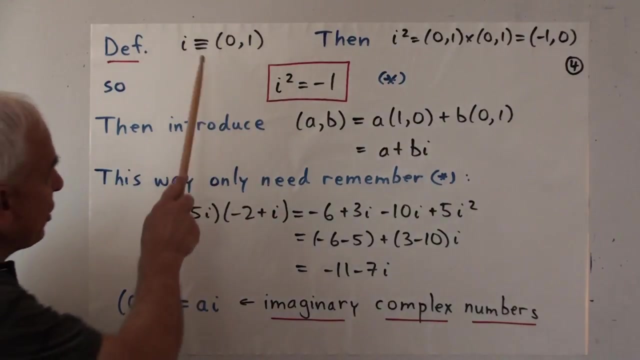 we're taking every vector and changing it to its negative, So we're rotating essentially by 180 degrees or a half turn, which is essentially to negate any vector. It's a geometrical interpretation of this equation, And now we're going to use this particular complex number. 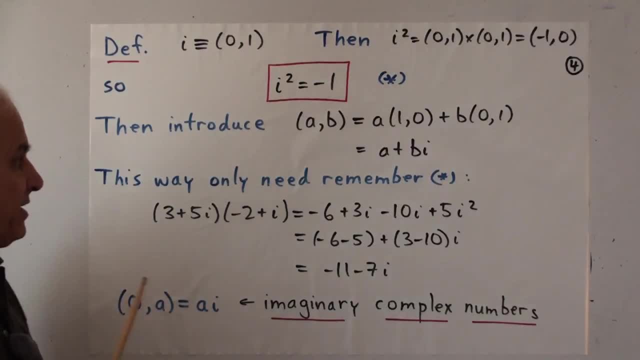 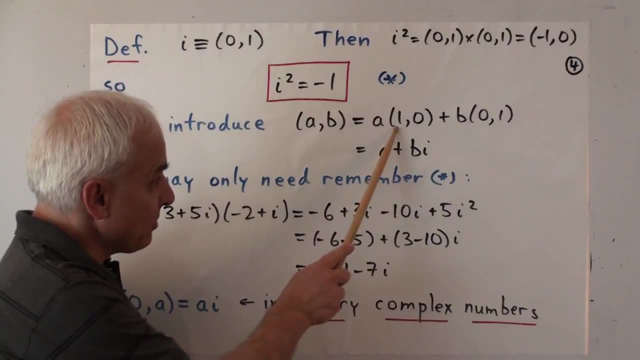 to simplify or give an alternate form for complex numbers. So instead of writing the pair a- b, we'll think of this as being a times 1, 0 plus b times 0, 1.. And this 1, 0. 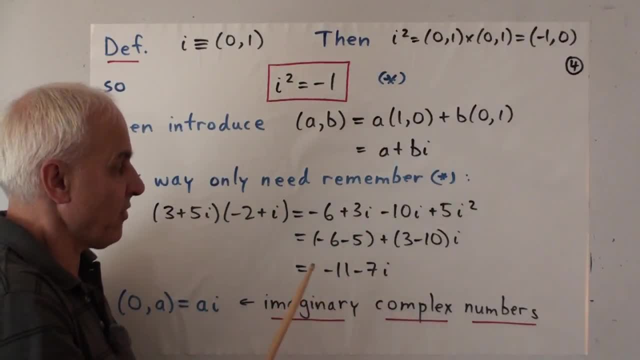 is really the number 1, which we don't need to write, And this 0, 1 is this new number i, So we can write this expression as a plus b i. That's an alternate form for complex numbers, which is the one that we're going to probably use in practice most. 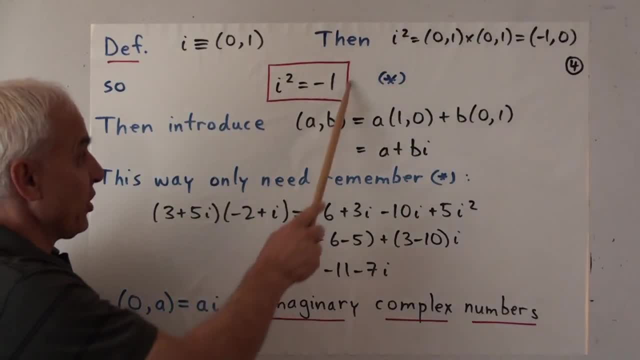 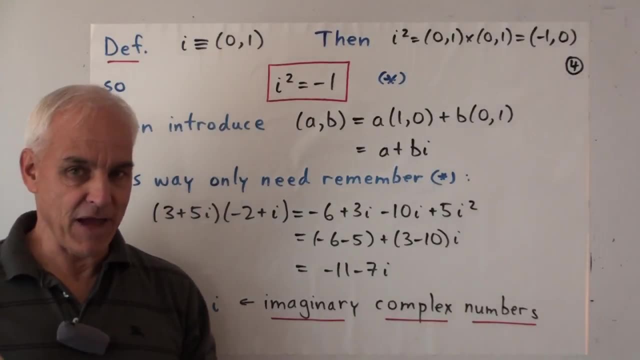 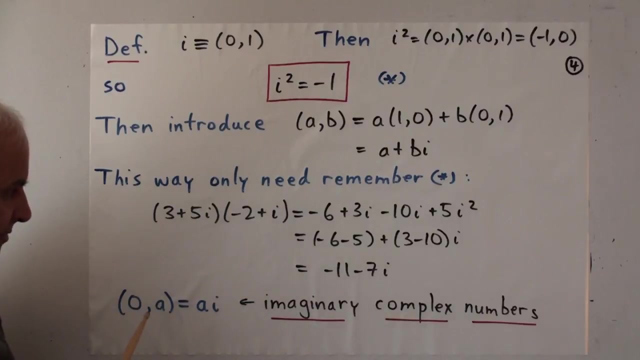 With this notation, this particular equation is really the only thing that we have to remember when we're multiplying. We can forget almost about that original rule as illustrated here. Suppose we want to multiply 3 plus 5i with minus 2 plus i, Then if we're just going to do this, 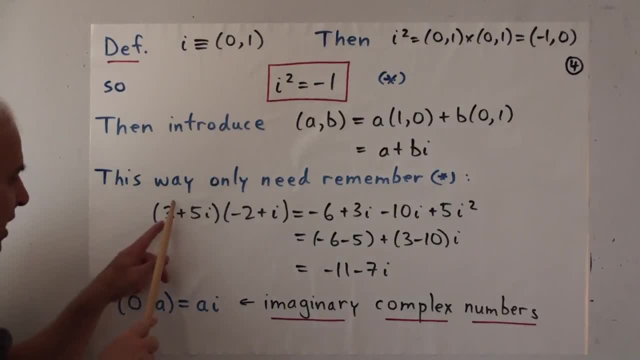 using the distributive law we get: 3 times minus 2 is minus 6,. 3 times i is plus 3i. 5i times minus 2 is minus 10i and 5i times i is 5i squared. 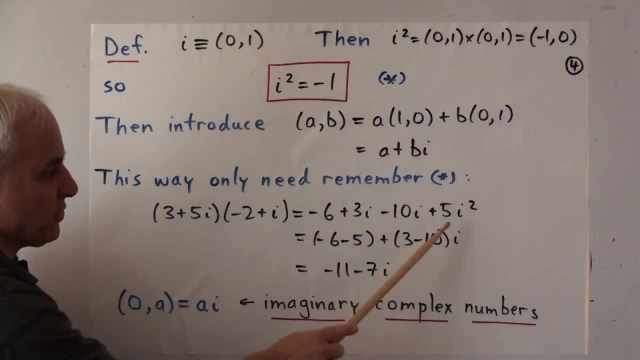 Well, if i squared is equal to minus 1, then we should replace this thing with a minus 1 to give us minus 6 minus 5.. And then the i's combine as 3 minus 10i, giving us all together minus 11. 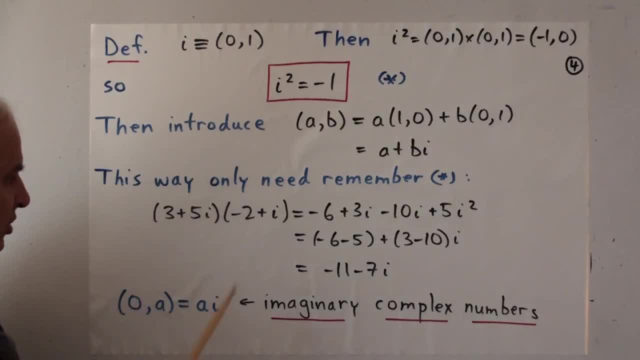 minus 7i, And you can check that. this is the same thing that you would get if you did the original multiplication in terms of this times this minus, this times this And this times this plus, this times this. It's that the advantage is that we don't actually have to remember the formula for multiplication, we only 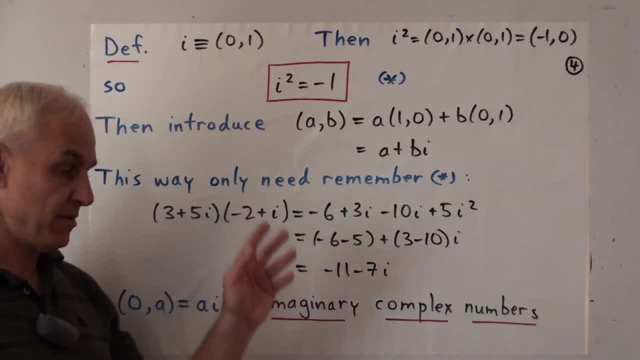 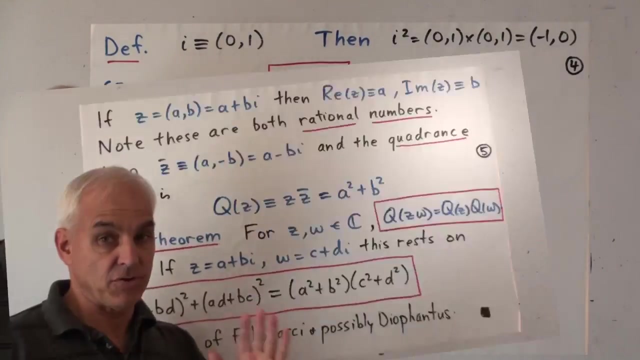 have to remember this very simple law and use natural distributivity, Alright. and then numbers like this, 0a, can be just written as a times i. so these are the imaginary, complex numbers that lie on the y-axis. Alright, now let's introduce a little bit more terminology. and then 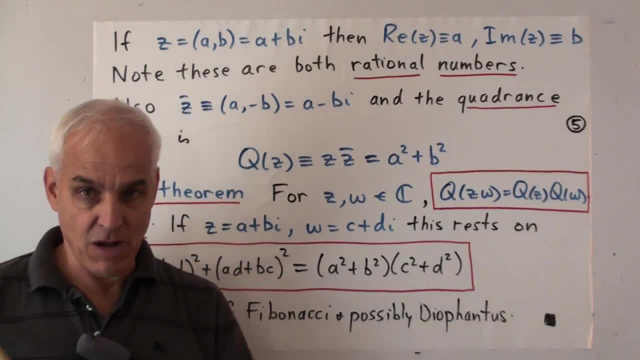 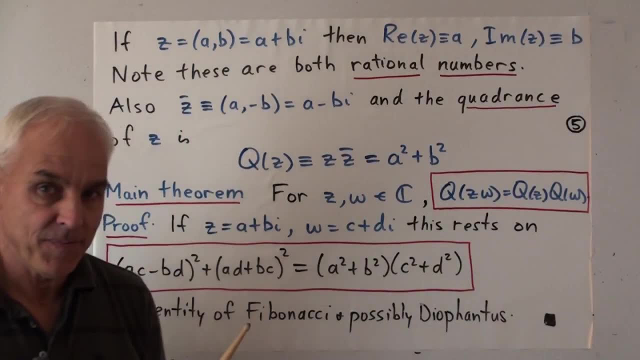 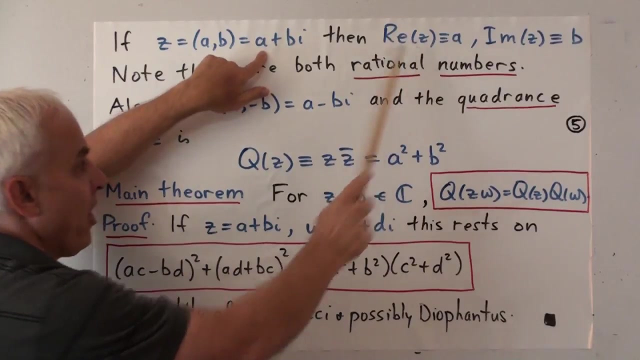 the main theorem, the most important fact about complex numbers. So if z is equal to ab or, in our new notation, a plus bi, then let's give a name to these numbers: a and b. Let's call a the real part of. 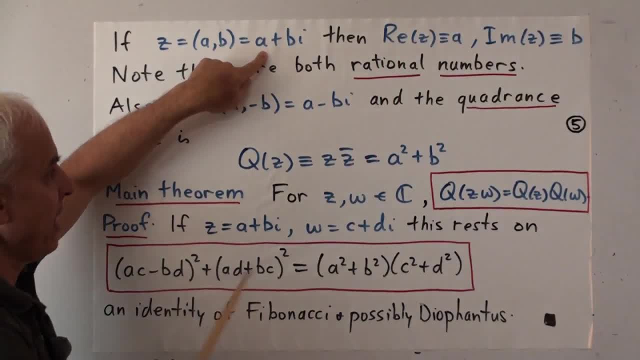 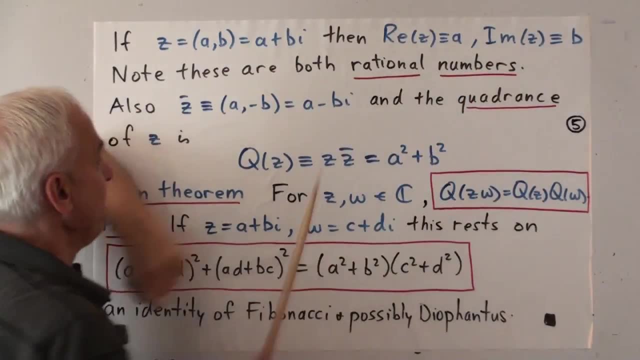 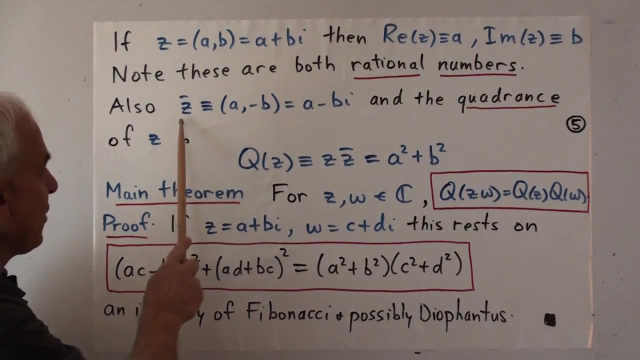 z and denoted by this re of z. And let's denote the rational number b as the imaginary part of z and denoted by im of z. Note that these are both rational numbers. Let's define the complex conjugate. So, if we take 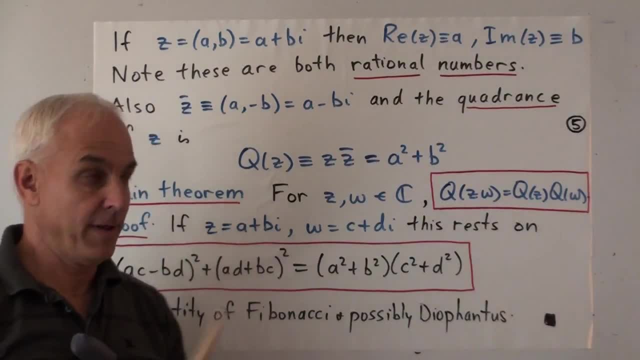 the complex number z and we put a little bar over it. that means complex conjugate, and what you're going to do is you're going to take the pair and you're going to negate the second coefficient In terms of a plus bi. that. 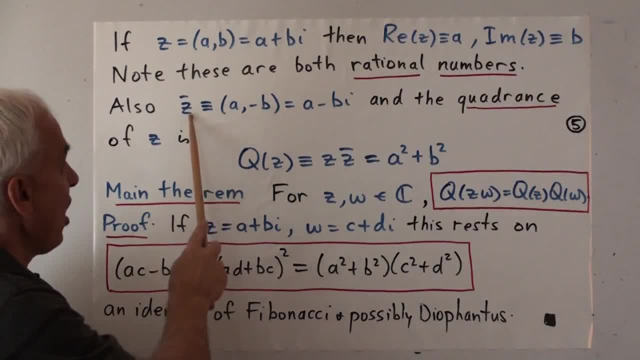 changes to a minus bi. So that's the complex conjugate of z. That's an important idea in complex numbers and we're going to use that to define the quadrants of the complex number. So the quadrants of the complex number z is q of z. It's, by definition, z times z. 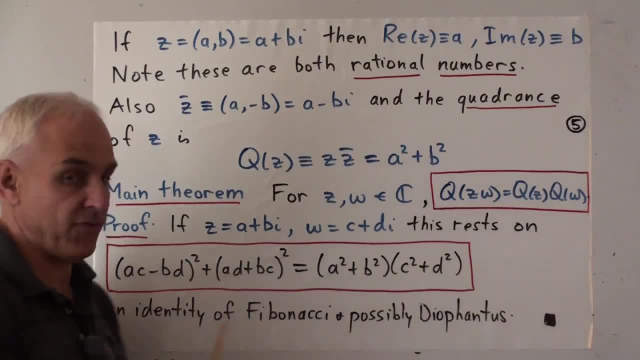 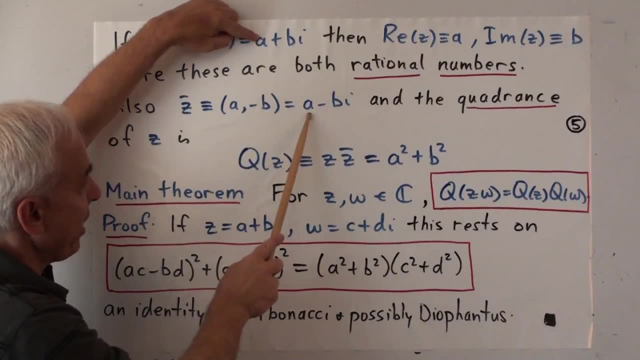 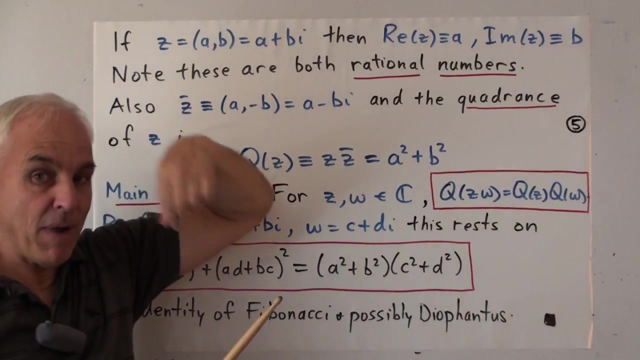 bar. It's what you get when you multiply this times this. Now, that's a difference of squares. So if you multiply a plus bi times a minus bi, you're going to get a squared minus bi squared, But i squared being minus one, that amounts to a squared. 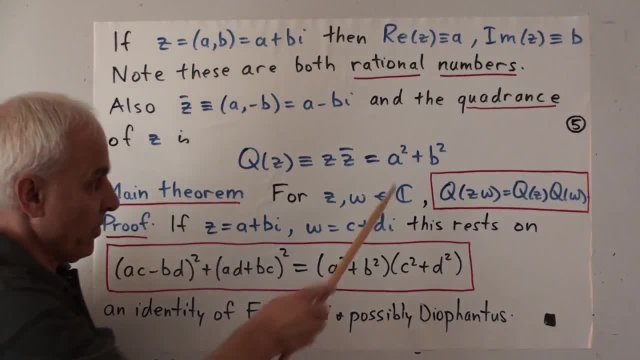 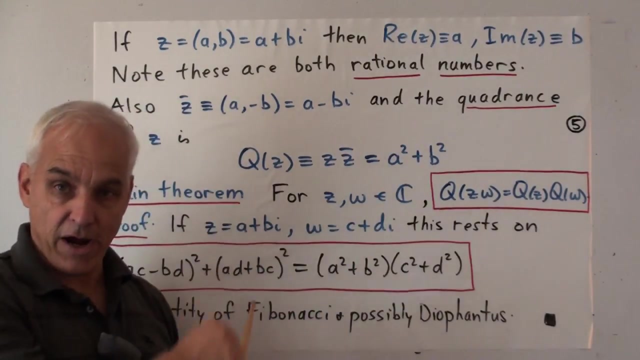 plus b squared. So what we're getting is the sum of the squares of the coefficients of the complex number z. If you think in terms of a diagram and Pythagoras' theorem, this represents the area of the square that Euclid would have built on. 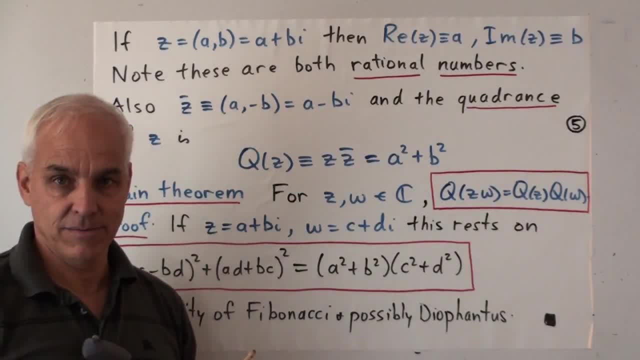 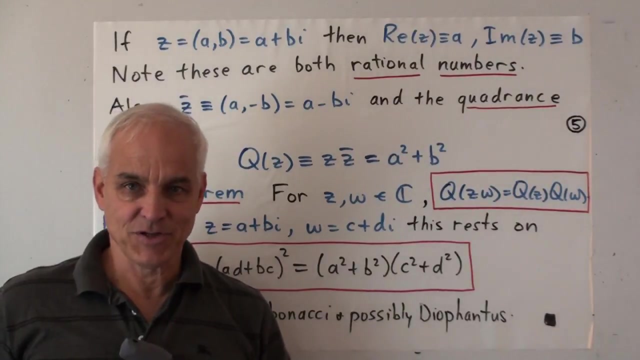 the segment from zero to the point z. It's the quantity that appears as the hypotenuse area in Pythagoras' theorem. Now, an important point. In ordinary texts one then uses this. in fact, one doesn't give this thing a name, One goes directly to what's considered more fundamental. 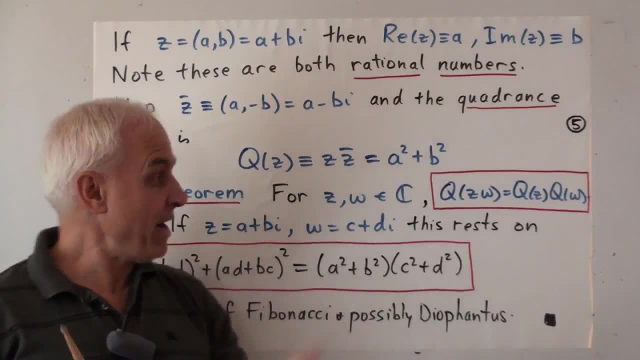 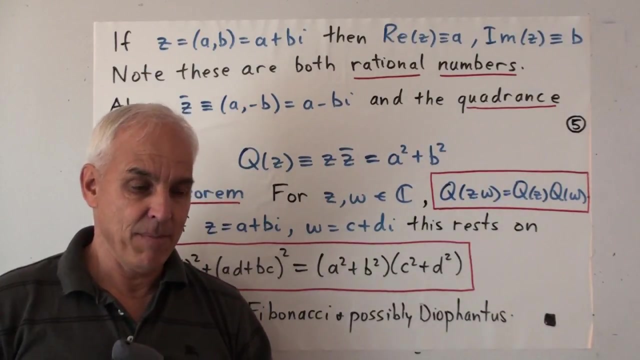 namely the length of the complex number z, By taking a square root of this. we do not want to do that. We do not want to use square roots if we can avoid it. Square roots properly. take us outside of pure mathematics, because the square root is actually very 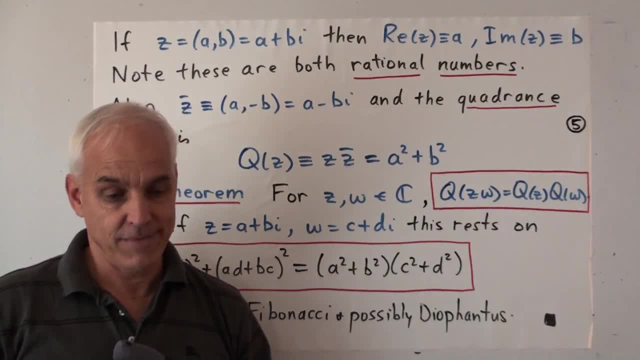 subtle, problematic construction, As evidenced by the fact that if I ask you what square root of 13 is, you can't give me a precise answer. Your calculator will spit out a certain number of digits, but you don't actually have a number whose square 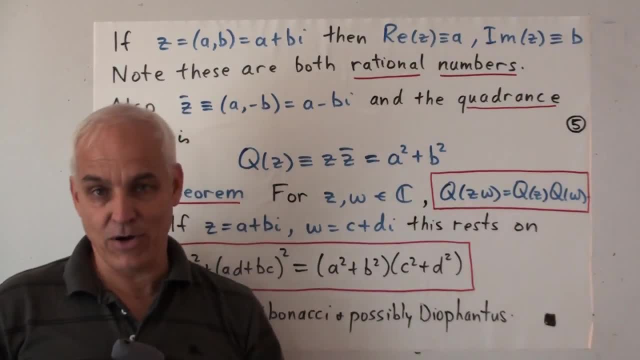 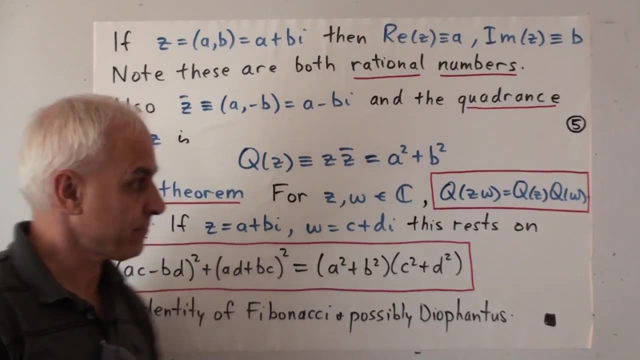 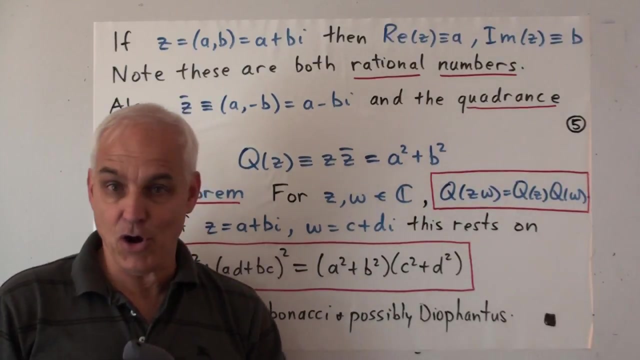 is 13.. In fact, the existence of square root of 13, as I argue in my Math Foundations series, is highly suspect. So we're going to avoid that. We're not going to mention length of vectors or moduli of complex numbers. 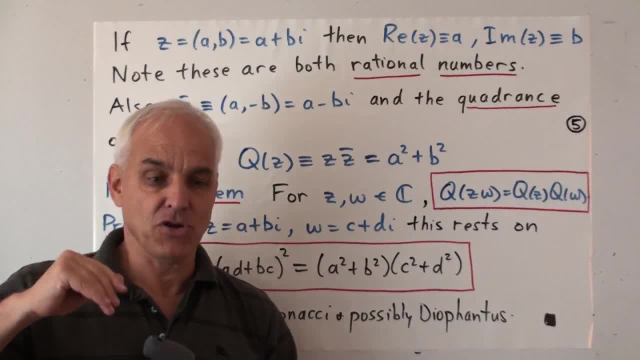 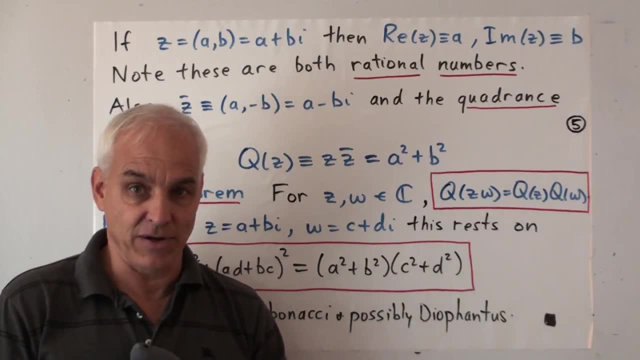 This is a big step up conceptually actually. So not using that means that we have to make everything algebraic. We're forced essentially in the right direction in terms of our thinking. So I know this is a little bit novel to many of you, but 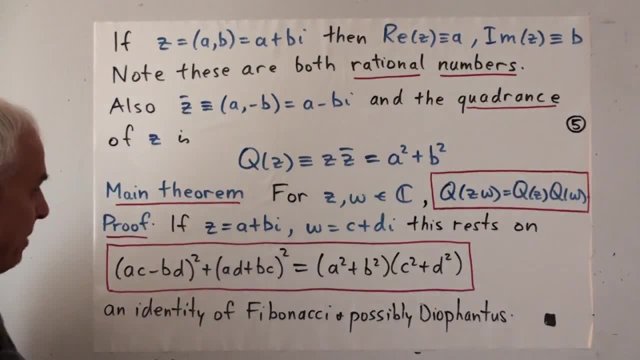 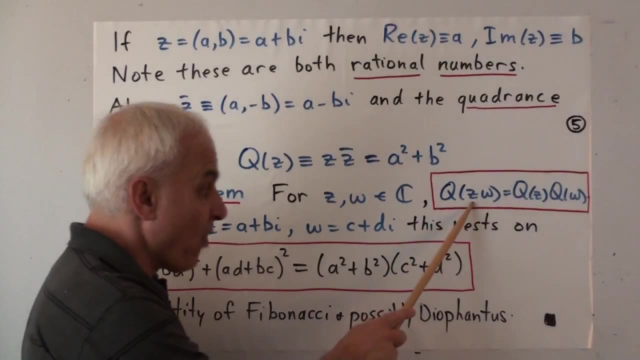 believe me, there's much to be said for it. In particular, we have this main theorem, which looms as an absolute pillar of the subject, which is that if you have two complex numbers, z and w, then the quadrants of the product z times w. 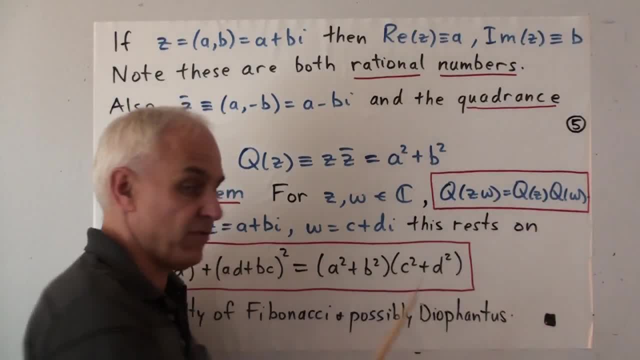 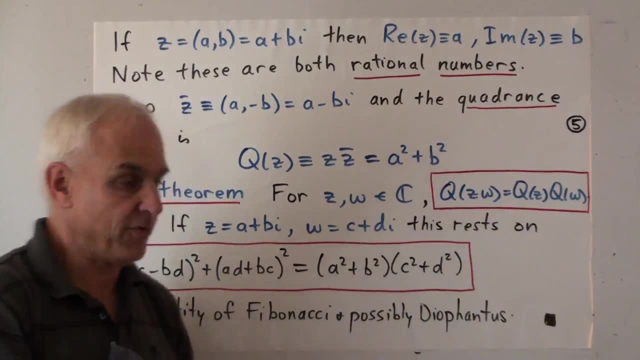 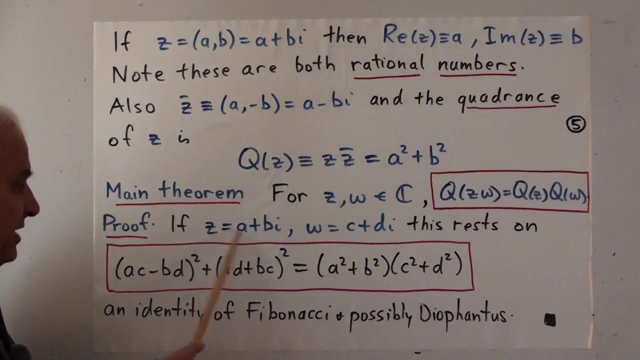 is the product of quadrants of z times quadrants of w. So the quadrants of a product is the product of the quadrants. So let's prove it. Let's say that z is equal to a plus bi and w equals c plus di. Then the 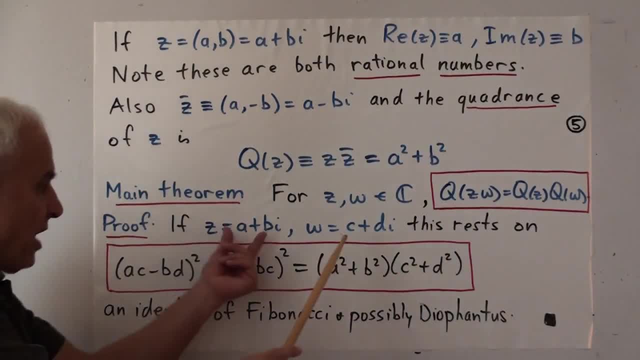 left-hand side. what does it look like? Well, we have to multiply z and w, and then there'll be two coefficients and we have to take the first coefficient squared plus the second coefficient squared. That's what the quadrants of z times w is. So here, I hope you recognize. 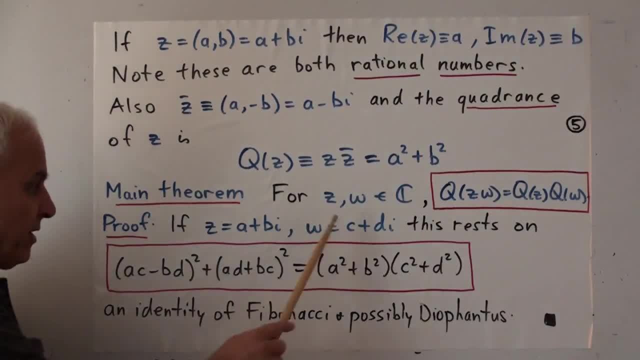 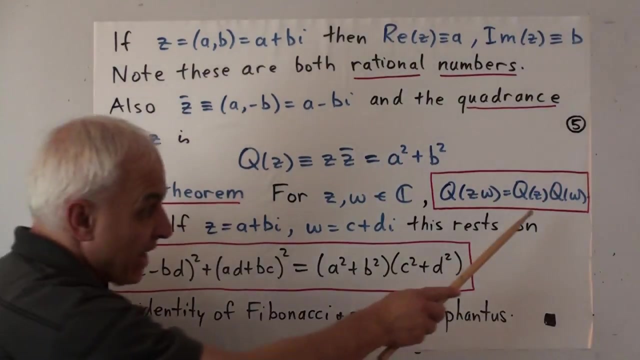 this is the real part of the product- ac minus bd, And the imaginary part of the product is ad plus bc. So we have to take this squared plus this squared. That's the left-hand side. The right-hand side is the quadrants of z. that's a squared. 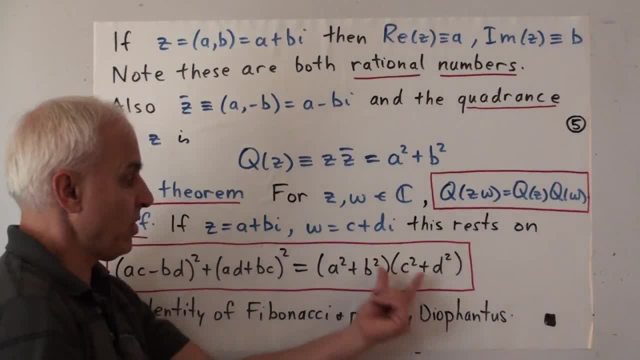 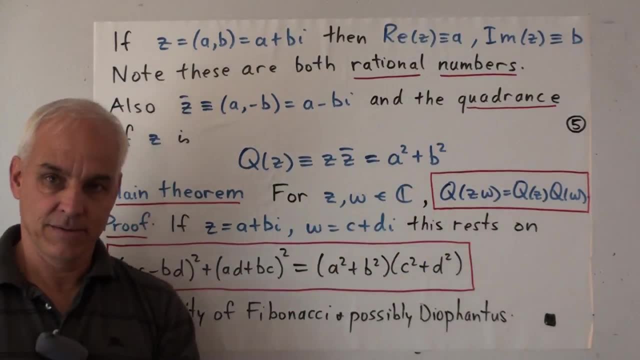 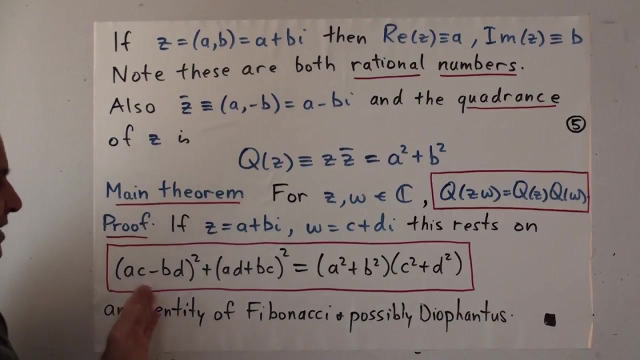 plus b squared, times the quadrants of w, which is c squared plus d squared. So the assertion is that this equals this For any rational numbers: a, b, c and d. And this is an identity of Fibonacci, Leonardo of Pisa. 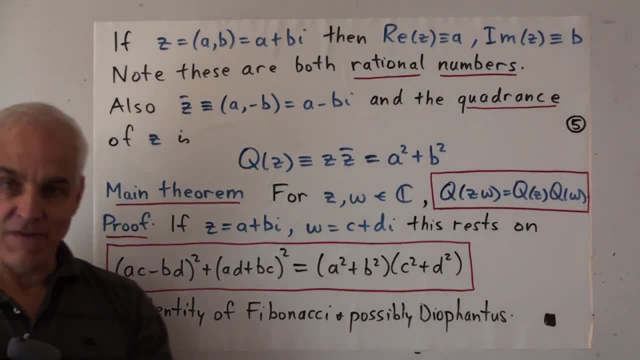 And in fact possibly it goes back to Diophantus 300 years after Christ. Let's check why it's true. If we square this, we're going to get ac squared, which is this term here plus bd squared, which is this term minus twice the product. 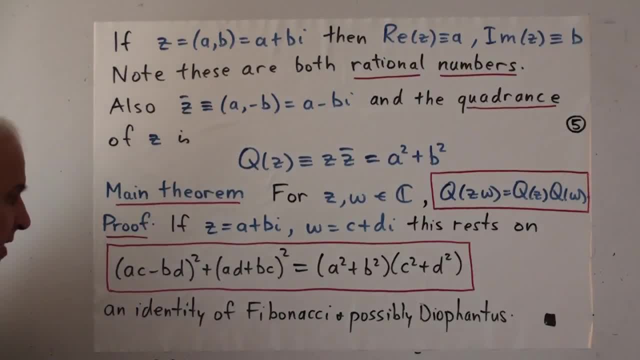 Let's forget about minus twice the product temporarily. When we square this thing, we're going to get ad squared which is: this times this plus bc squared, this times this plus twice the product. Alright, so minus twice the product. over here is minus 2 times a times c, times b. 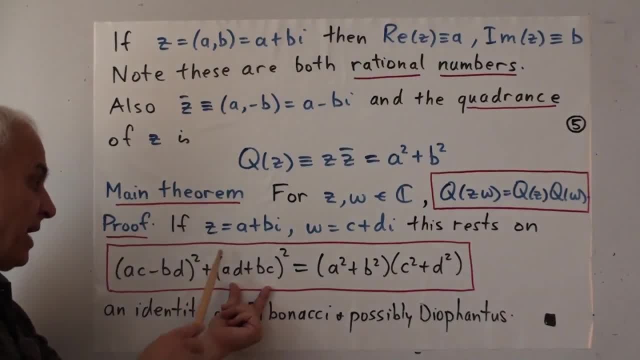 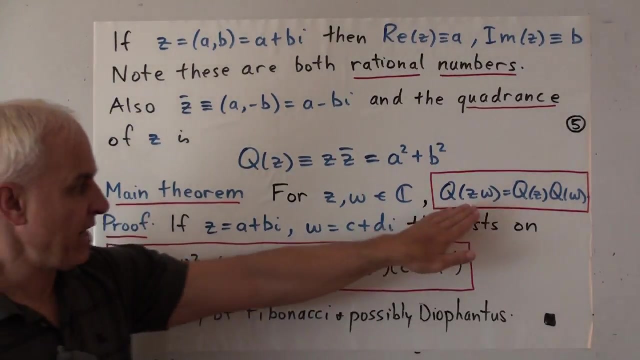 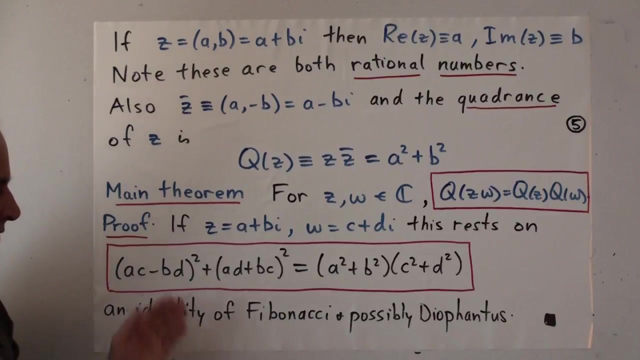 times d and plus twice. the product here is 2 times a times d times b times c. Those two terms are conveniently exactly the same with opposite signs, so they cancel and the equality is obvious. This drives this basic result Very important, crucial: identity, that's. 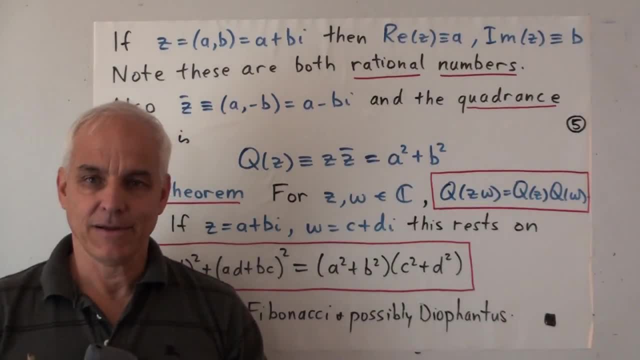 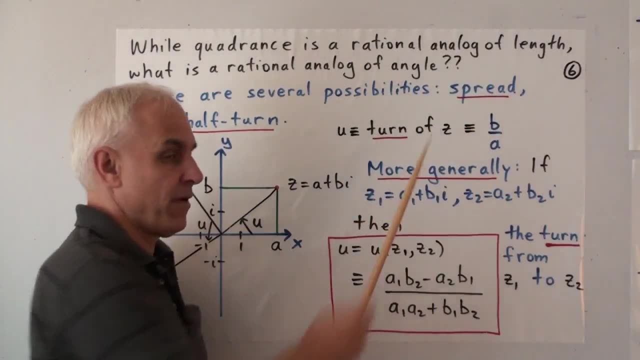 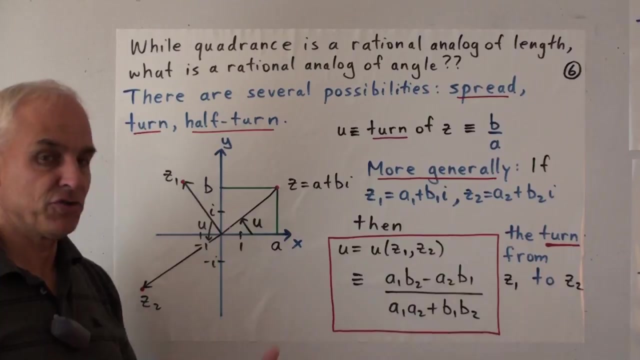 somehow at the heart of the beauty and usefulness of complex numbers in terms of rotations. So, while quadrants is a rational analog of length or distance, what is a rational analog of angle? Traditional treatments of complex numbers rely heavily on the notion of length. 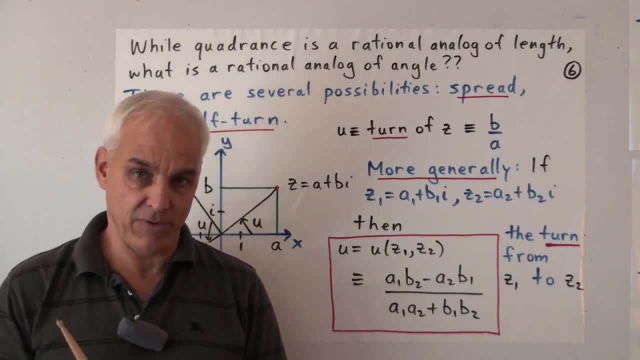 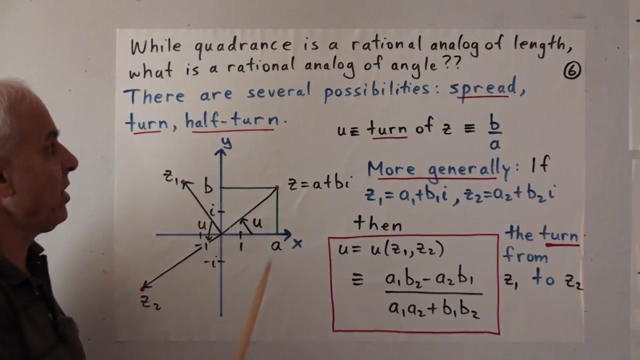 and angle for polar coordinates for complex numbers. Maybe it's inconceivable to you that you could study the subject without those two concepts if you're very familiar with complex numbers. But in fact you can. There are rational analogs of angle and there are a number. 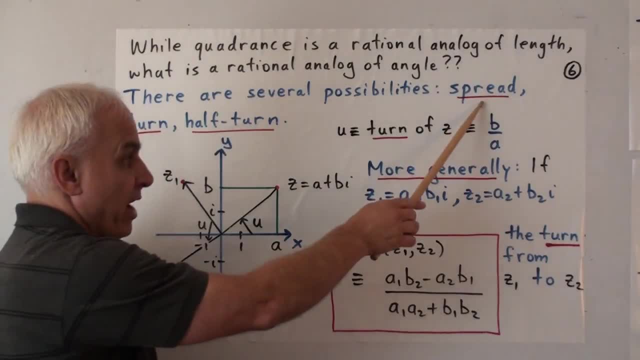 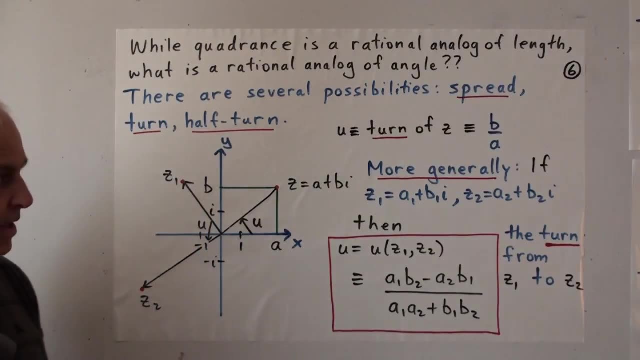 of different possibilities. One of them is the spread from rational trigonometry, or the turn or the half turn. The turn is also described in my book. The half turn I'm going to talk about in the Math Foundations or the Wild Trig series. It's 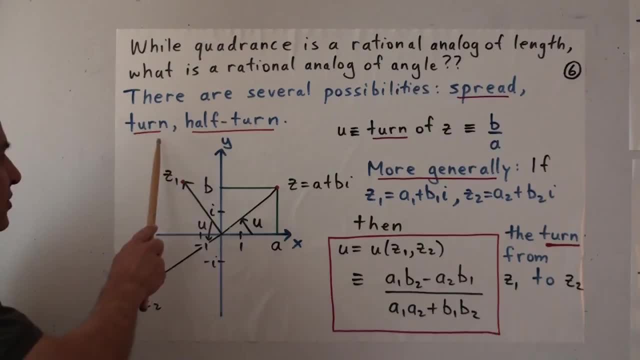 something else that's also very interesting. Today I'm going to tell you about the turn, which is a very natural idea that's closely connected with the geometry of lines in the xy plane. So here is a number: z equals a plus bi. x coordinate a, y coordinate b. 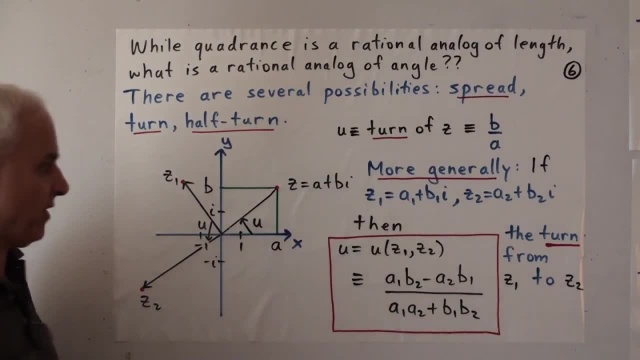 and here's a vector joining the origin to z. We're going to define the turn of z to be the slope of this line. The slope is, by definition, the change in the y coordinate divided by the change in the x coordinate, So the y coordinate. 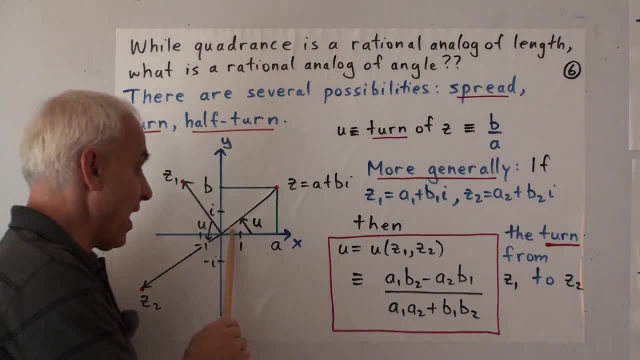 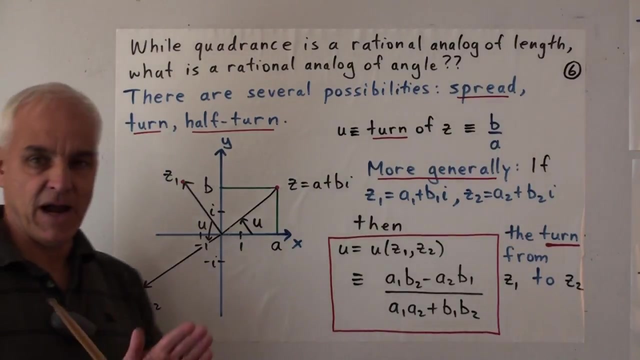 is b, the x coordinate is a, and that's how we're going to define the turn of this complex number. So, geometrically, we're going to relate it to a slope of a line. Now, more generally, what we really want to do is to define the turn between two vectors. 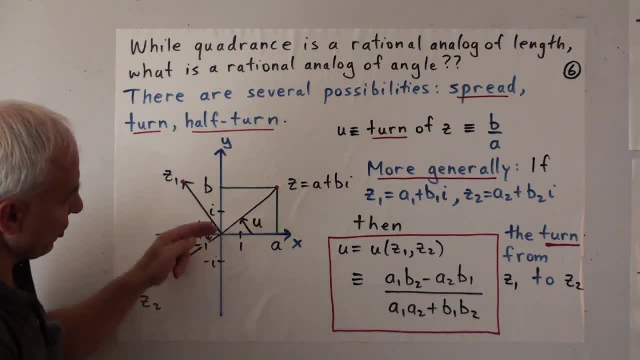 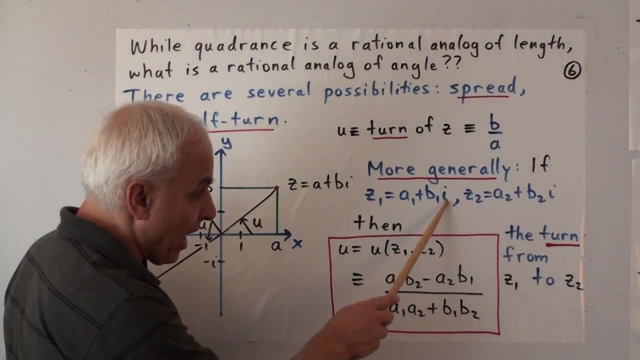 So this would be the turn between the vector 1,, 0, and z. But more generally, if we have z1 is a1 plus b1i and z2 is a2 plus b2i, then it turns out that 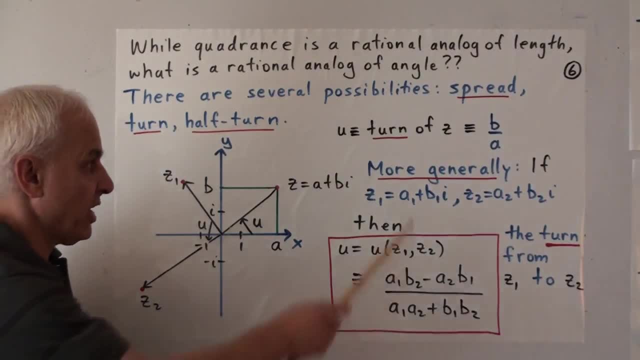 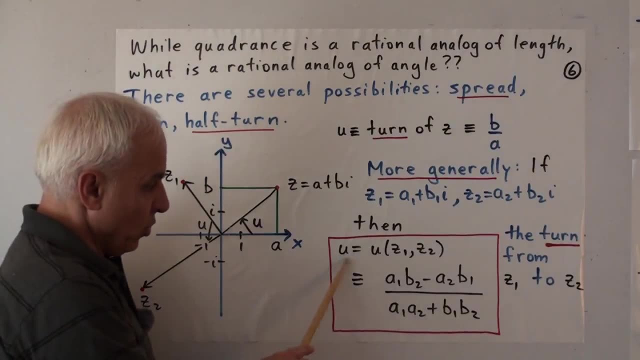 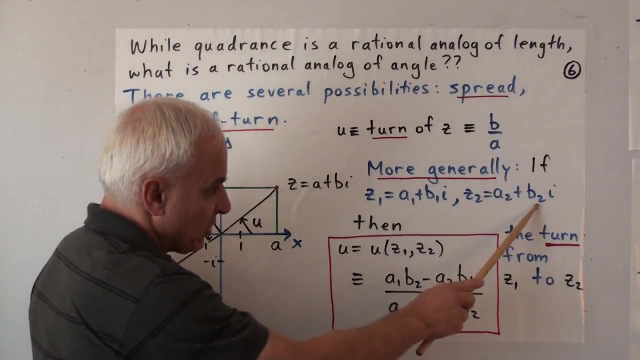 this is the formula for the turn, which is a generalization of this slope of line. What is it So? u? the turn from z1 to z2, is, by definition, a1b2 minus a2b1 in the numerator and the denominator. 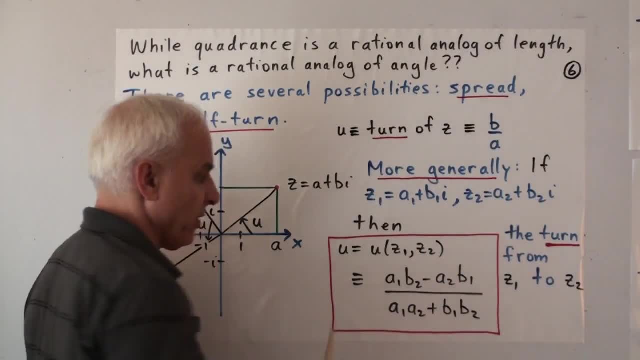 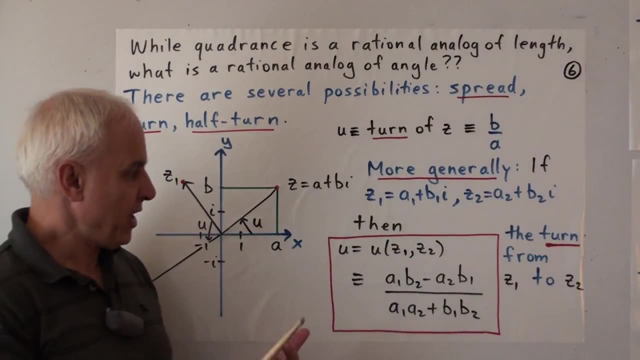 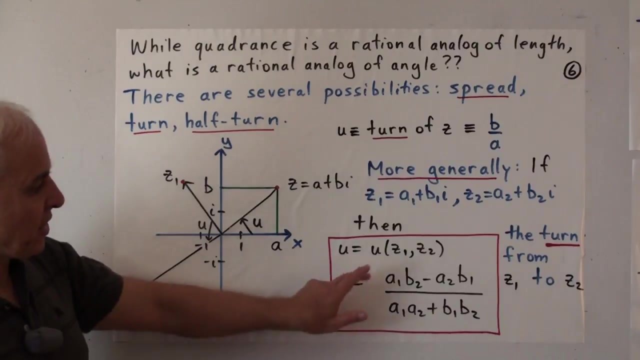 a1a2 plus b1b2.. Now these two expressions look a lot like the coefficients of the products of z1 and z2.. And if you think about it actually for a little while, you see that these are the complementary expressions. 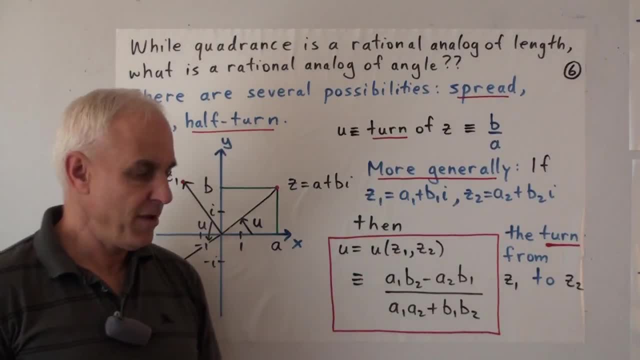 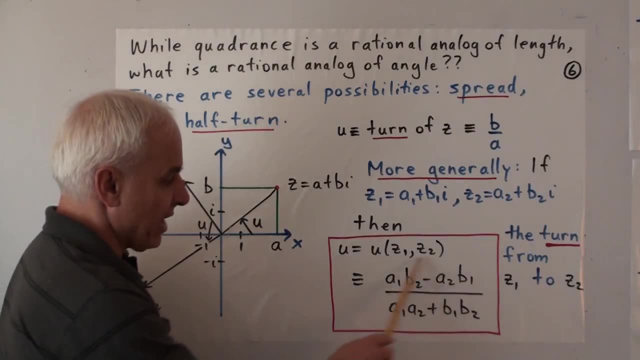 that are linear in the various variables, complementary to the two expressions that are used in the product. This you may also recognize as a determinant. Essentially, it's an area of a parallelogram formed by the two vectors And this here you recognize as a dot product. 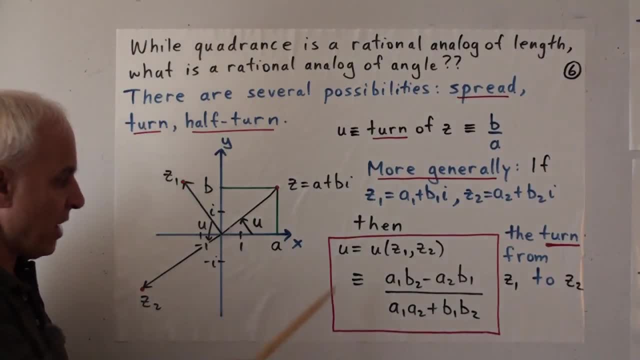 between the two vectors. Now, this particular expression is very nice. It's the definition of the turn from z1 to z2.. And in the special case when the first vector is say, then you can check that this thing reduces to. 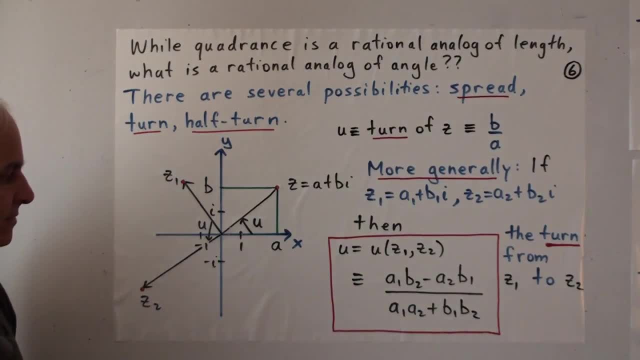 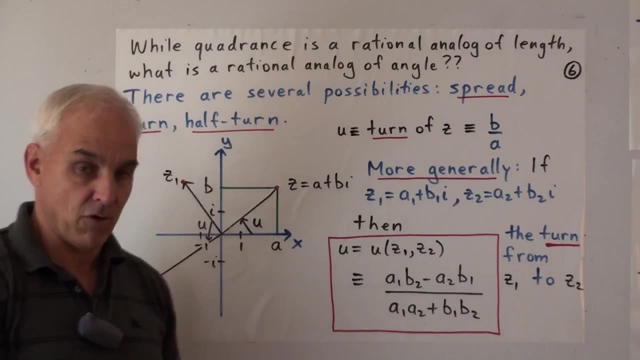 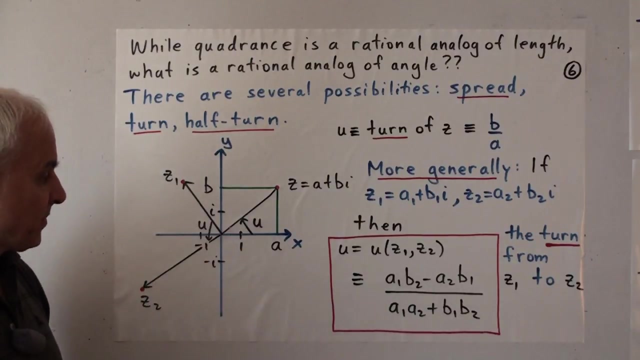 this one here. There's one more thing to be said that there's a slight problem with this definition if a is 0. In other words, if the complex number is perpendicular to the x-axis or 90 degrees, then the turn is: 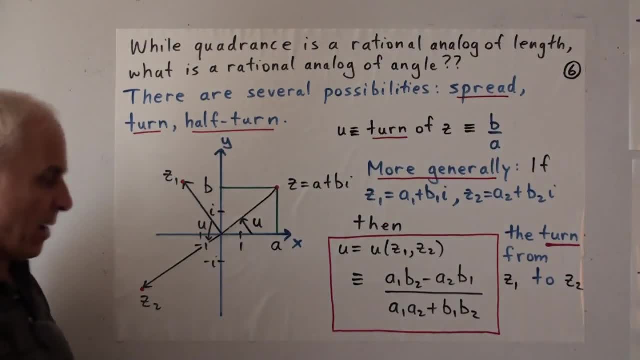 either undefined or infinite, And that will also happen here. in this more general case, If the two vectors are perpendicular, say z1 and z2 are perpendicular, then the turn will be undefined. By the way, here is the terminology that I like to use. 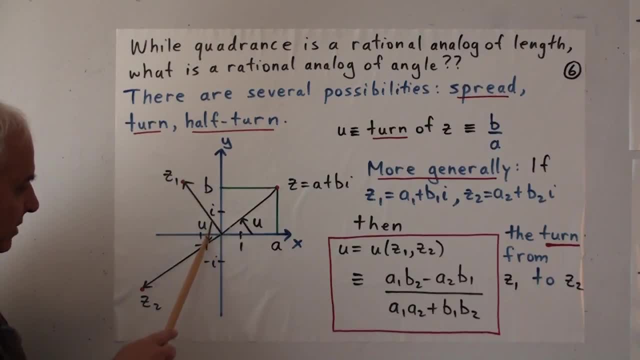 So it's given by this little straight line with a little arrow, and there's the u. The arrow here denotes that the object has an orientation. It depends on which complex number is first and which one is second. You can check that. if you change the order, then the turn. 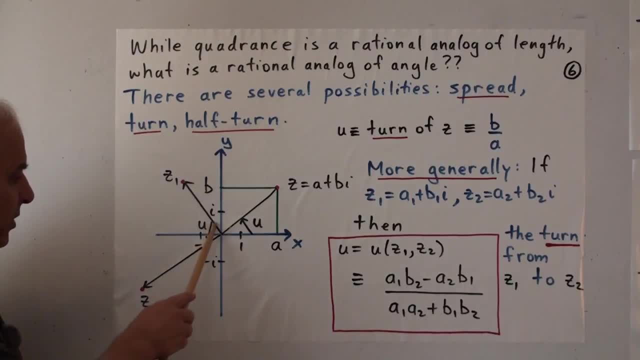 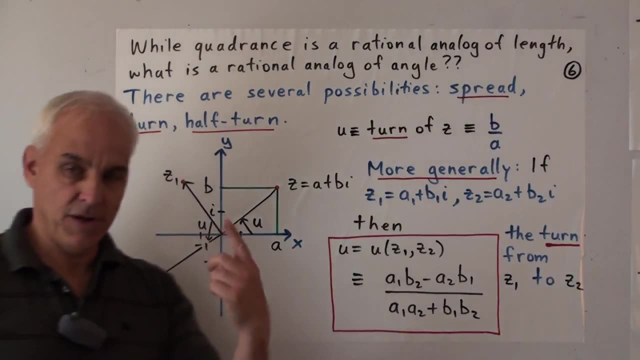 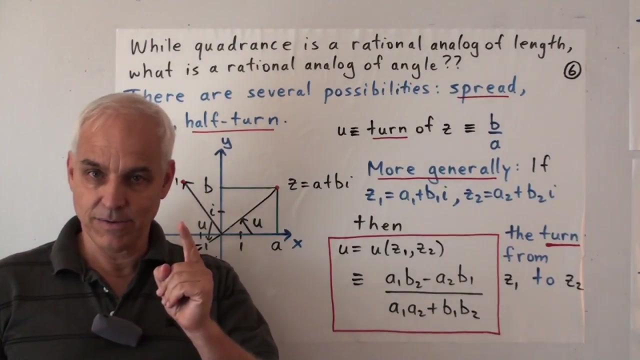 negates. Alright, so this is how we're going to express the turn from z1 to z2.. It's a number associated to the two complex numbers that measures somehow how far apart they are. It's a replacement for angle, But it's a rational replacement, No transcendental. 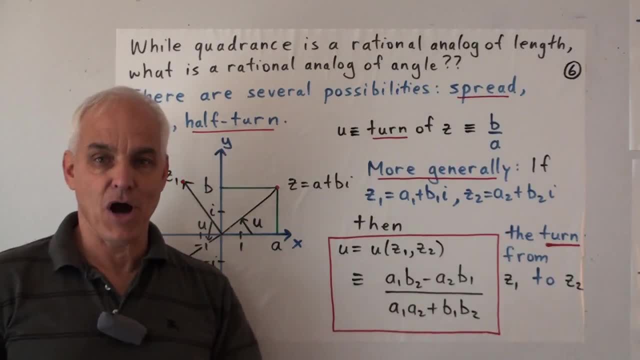 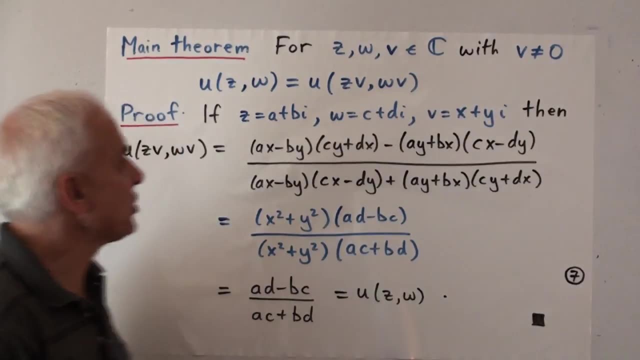 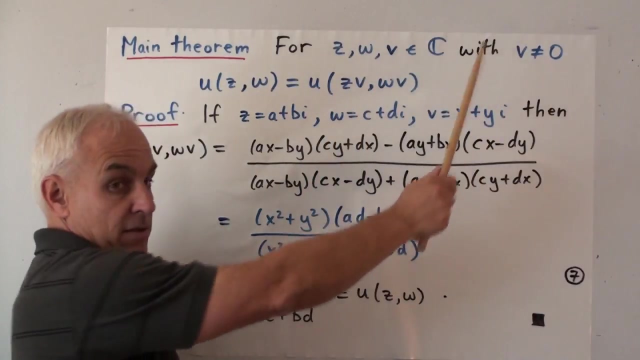 functions or definitions are required. And here's the main theorem for turns, The theorem that asserts that if we have three complex numbers- z, w and v- with v not zero, then the turn from z to w is the same as the. 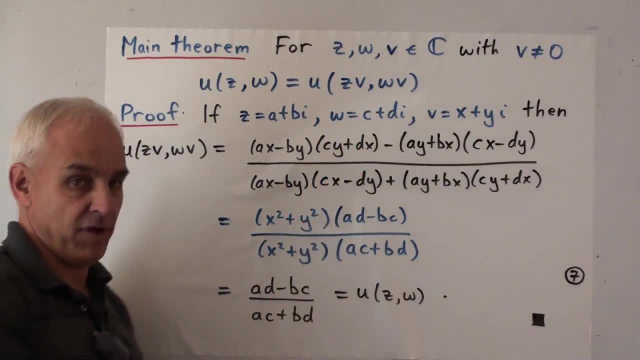 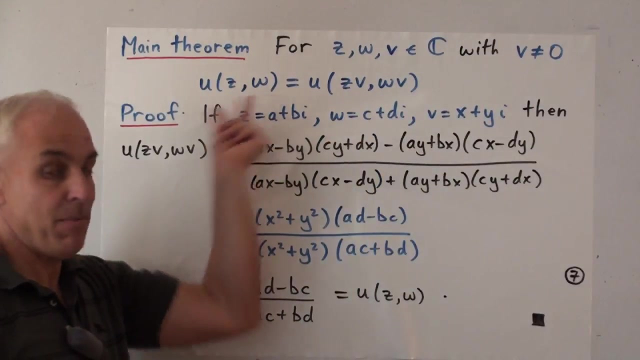 turn from z times v to w times v. In other words, when we multiply both z and w by the same complex number, we get two new complex numbers, zv and wv. The turn between them is the same as the turn between the original z and w. 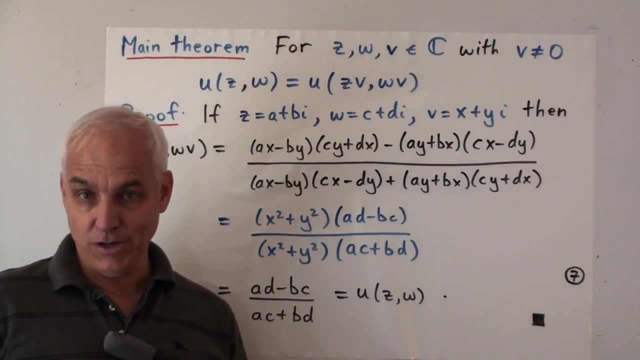 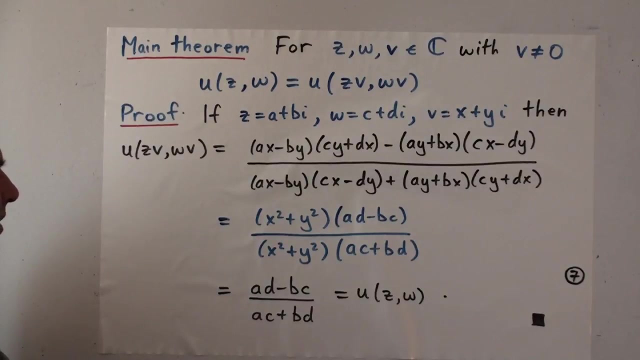 So this is a rational analog to the statement that when we multiply by a complex number, the angles between two complex numbers don't change Alright. so what's the proof? z, let's say, is a plus bi, w is c plus di, and let's suppose that v is. 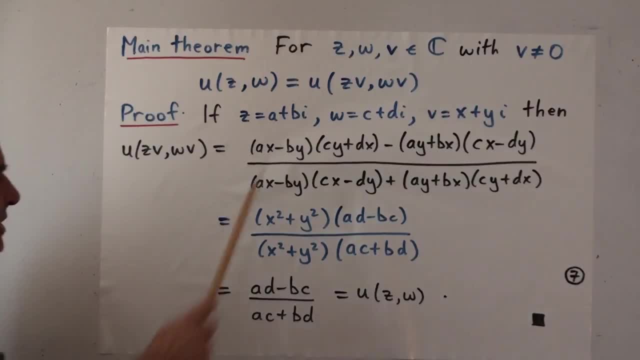 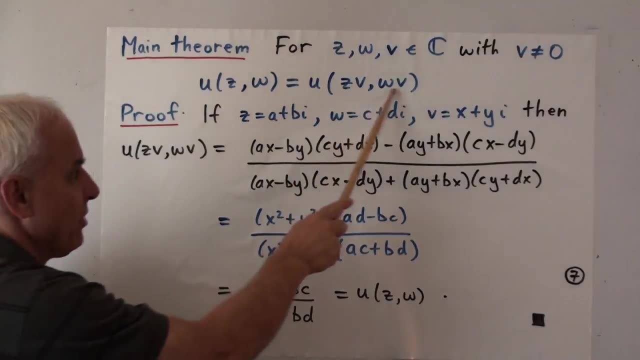 x plus yi. So let's calculate this thing here. Alright, so we have to calculate z times v and w times v, and then we have to apply the formula for the turn on the previous page. Alright, so z times v is going to be. well, there's going to be an ax. 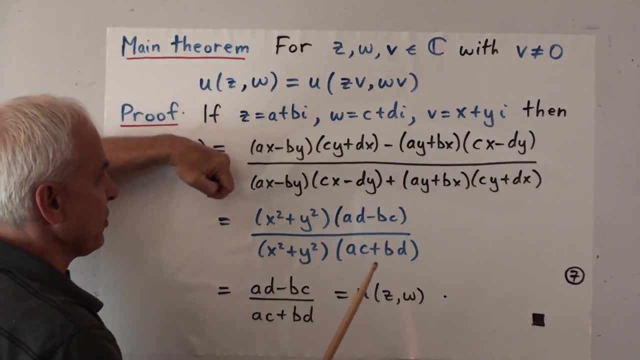 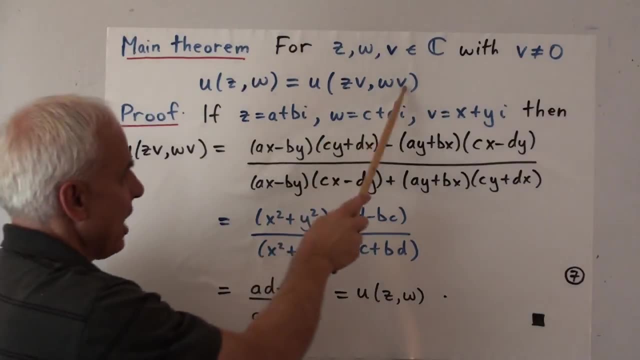 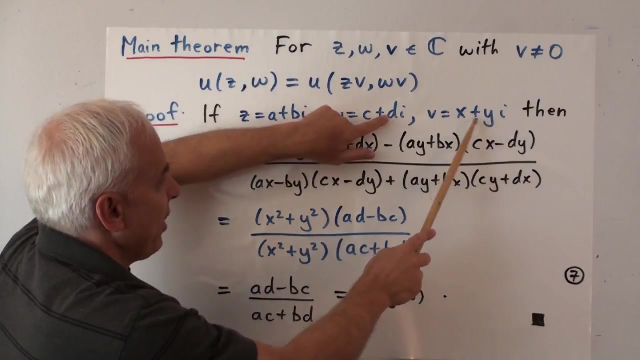 minus by. that's going to be the first term, and then there's going to be an ay plus bx And the w times v is going to have terms cx minus yd and the next one cy plus dx, And then you can check that. this numerator here is the determinant formed. 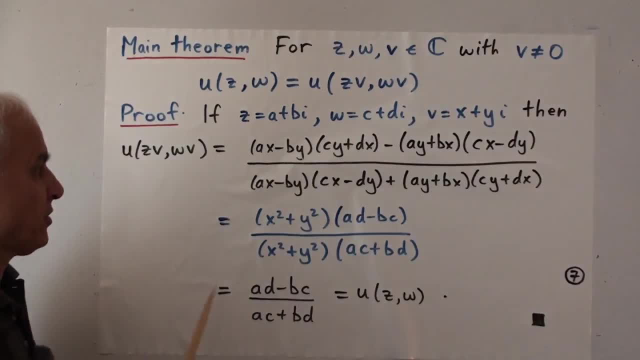 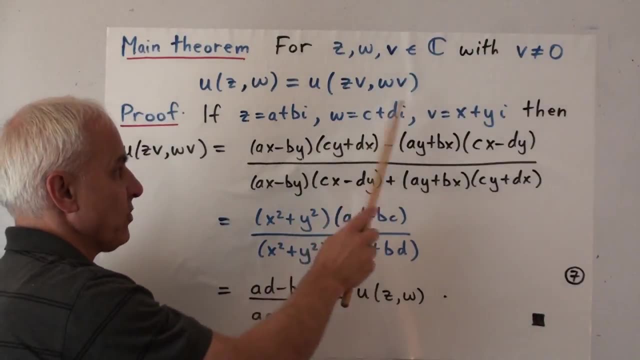 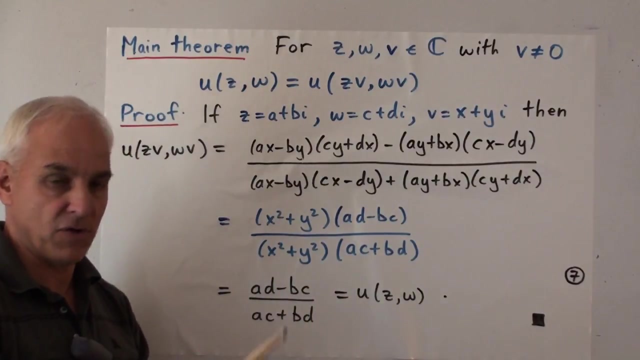 by those two vectors that we just mentioned. So the first coefficient of zv times the second coefficient of this one, minus the first coefficient of this, one times the second coefficient of that one. And here in the bottom is the dot product or inner product of those two vectors, The products of the two. 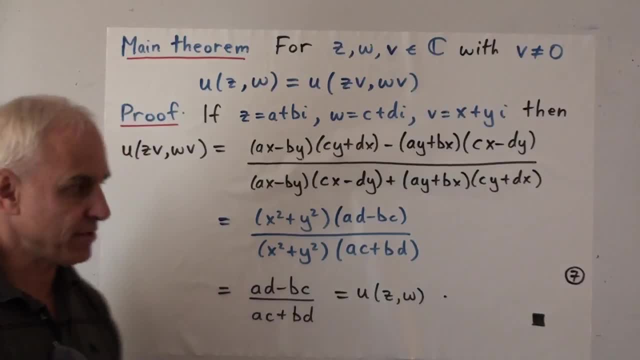 first coefficients plus the products of the two second coefficients, And now you have to expand this, Alright. so please do this. It's a good algebraic exercise. Expand the numerator, expand the denominator and stare at them both individually and convince yourself that they both. 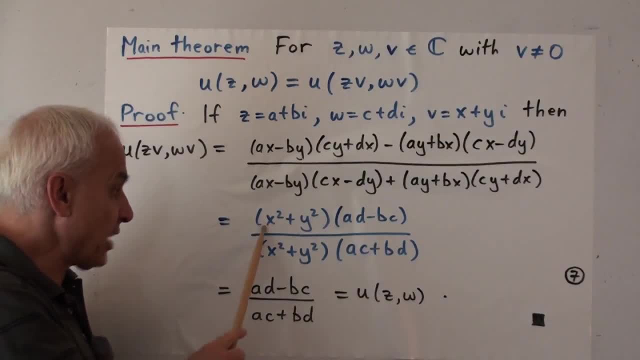 factor, The numerator factors as x squared plus y squared times ad minus bc, and the denominator factors as x squared plus y squared times ac plus bd. And since we're assuming this v is non-zero, the x squared plus y squared has to be: 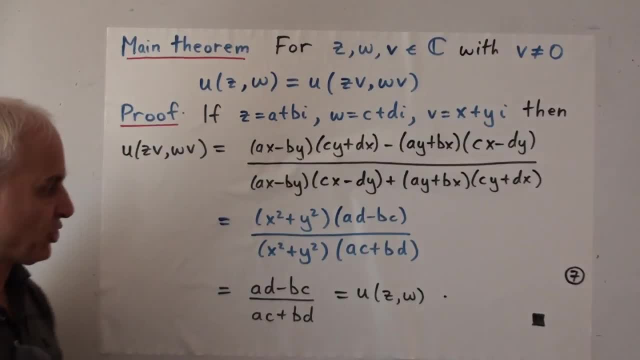 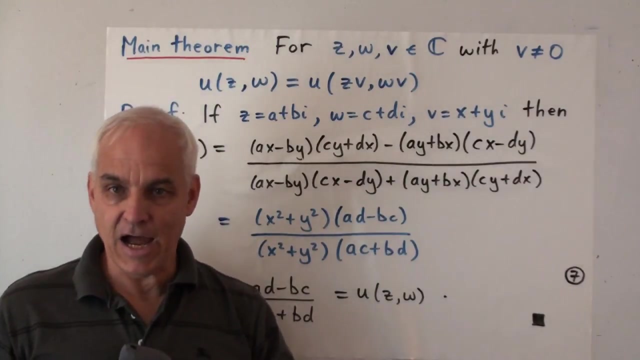 non-zero. We're talking about rational numbers here, And so conveniently these two terms cancel and we're left with the term between z and w. It's a lovely calculation that replaces the usual fuddling around with cosines and sines and formulas for cos and so on. 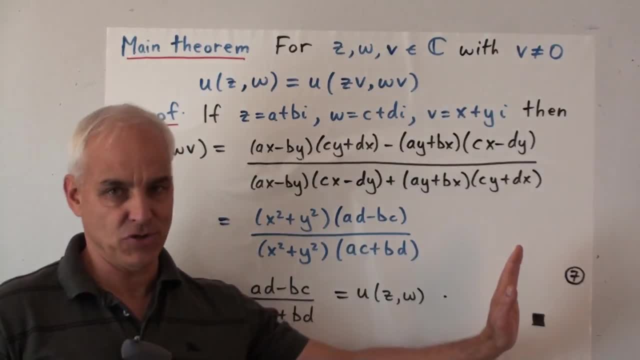 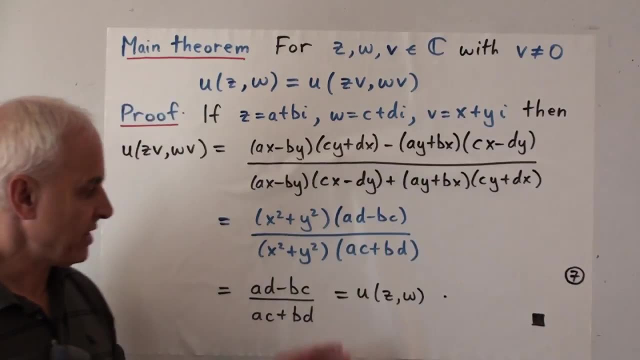 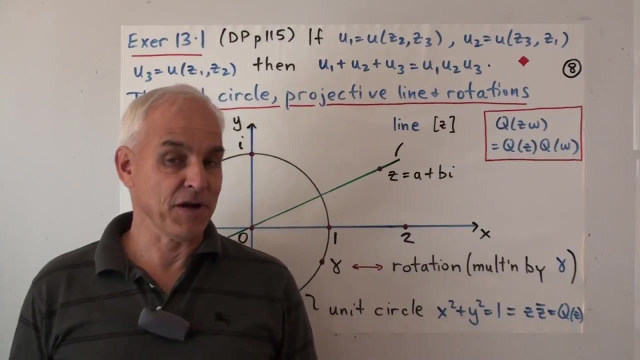 This is without any transcendental notions. That's a big step up, in fact, So it's something that's well worth thinking about. So the invariance of turn under multiplication Mathematics is a very conservative subject, especially pure mathematics, And many mathematicians have said to me: 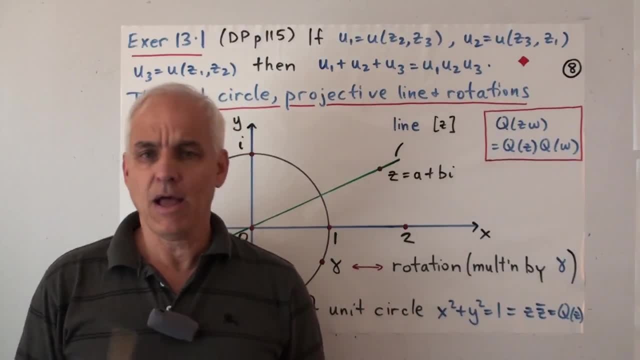 yes, Norman, that's all very good. a rational approach probably very interesting. but what about just the additivity of angles With angles? we can add them An angle of 3 degrees plus an angle of 4 degrees, you get an angle. 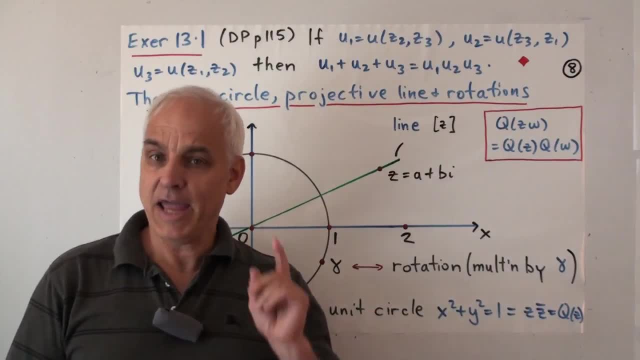 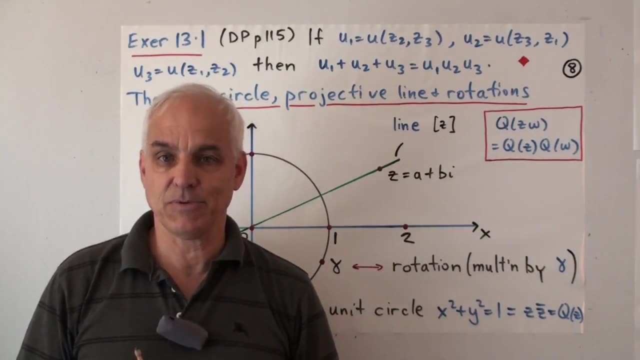 of 7 degrees. Well, that's true, but it's a very heavy price to pay The machinery and the transcendental business that you have to put into the subject in order to try to get at that linearity. It's an attempt to force linearity. 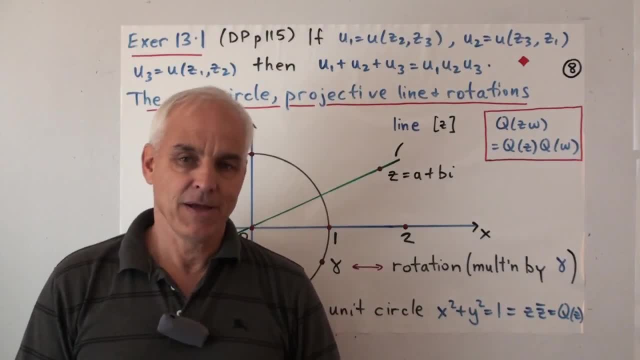 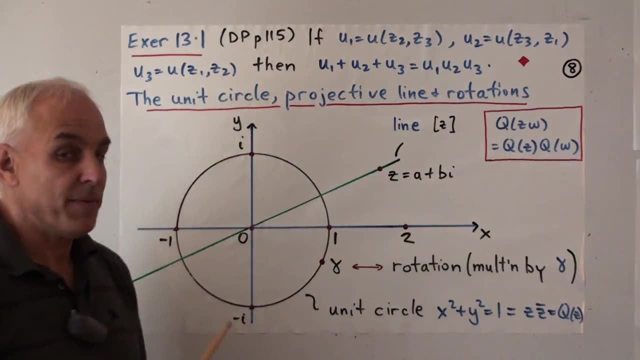 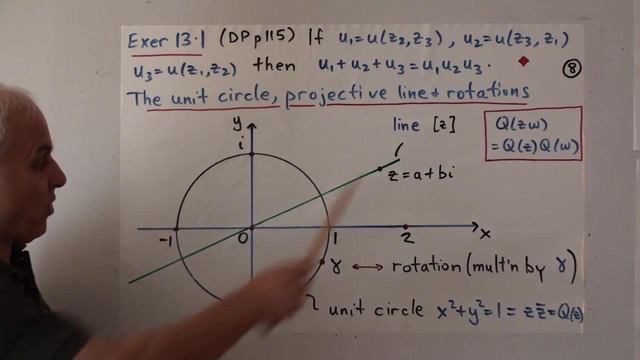 on the circular structure, which doesn't really want to go from a theoretical point of view, This exercise here gives you a rational analog to this additive structure. Suppose that you have three complex numbers- z1,, z2, z3, and we measure. 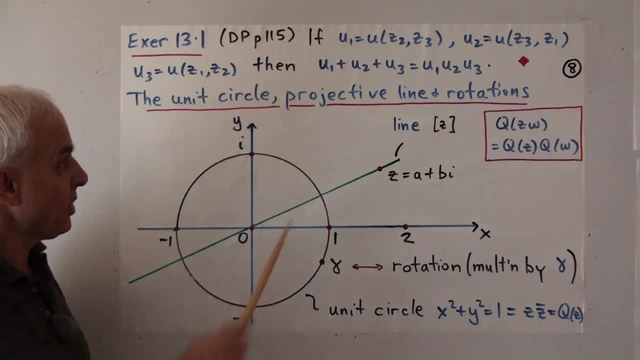 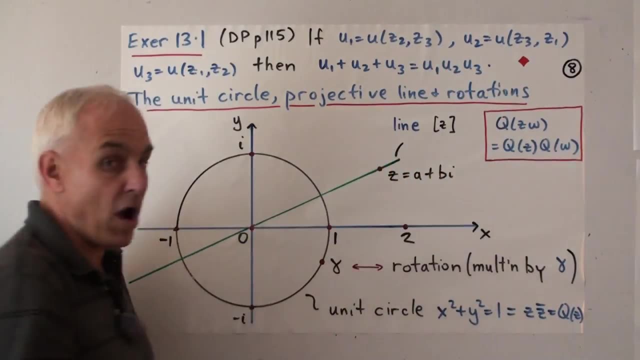 the turns between all three pairs. So let's say u1 is the turn between z2 and z3,, u2 is the turn between z3 and z1, and u3 is the turn between z1 and z2.. Remember the order. 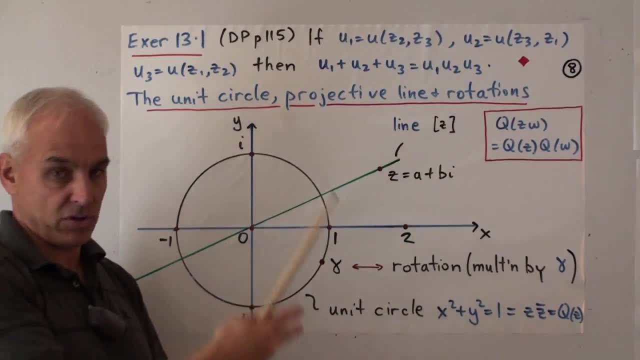 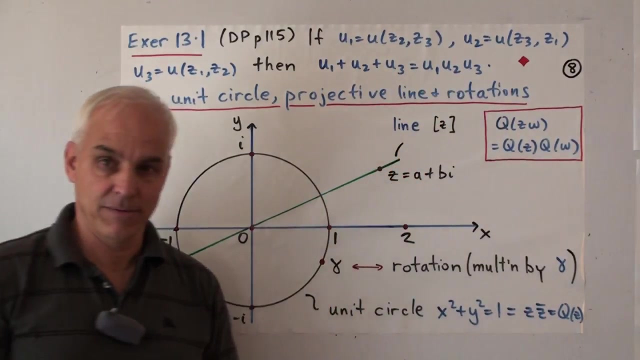 matters. so I'm kind of doing this in a cyclical order. so it's all symmetrical, Okay, so great exercise. Prove then that these three turns satisfy the following: pleasant relation: u1 plus u2 plus u3 equals u1, u2, u3.. And please do it. 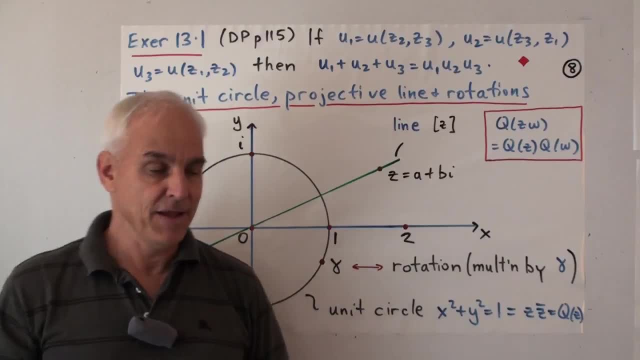 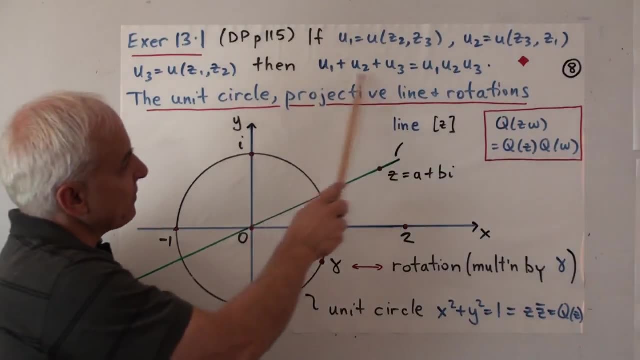 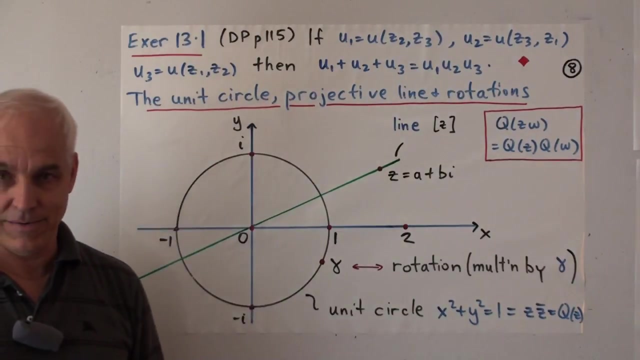 without any reference to tans of angles. This is a purely rational result. It deserves a purely rational proof. Notice that it means in particular that if you know two of those turns, then you have a linear equation for the third one. So, while it's not quite as 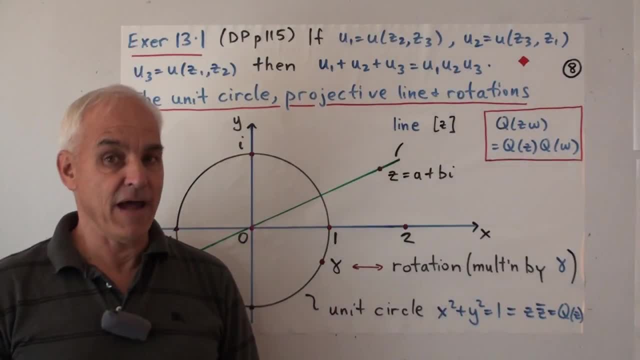 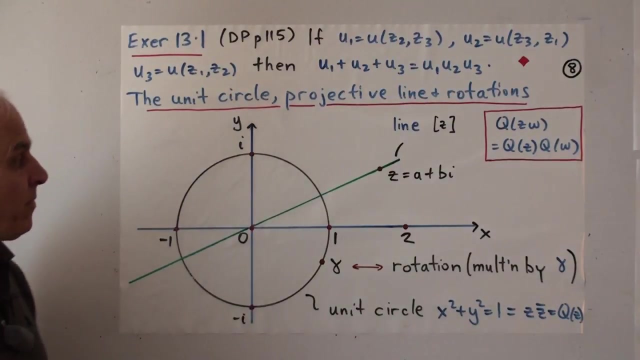 simple as just adding the two turns. it's not that much more complicated. Alright, now let's have a look at a very interesting circle of ideas. I want to connect the unit circle in the complex plane, which plays a very important role, to the projective line. 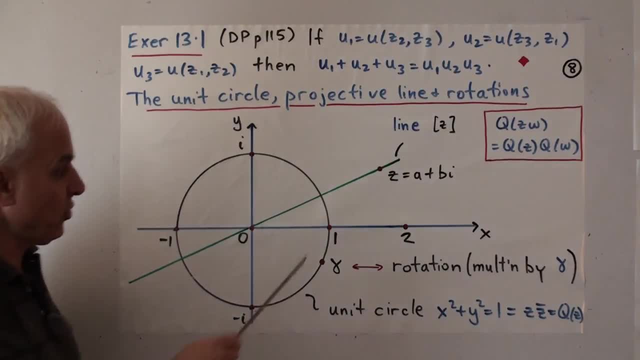 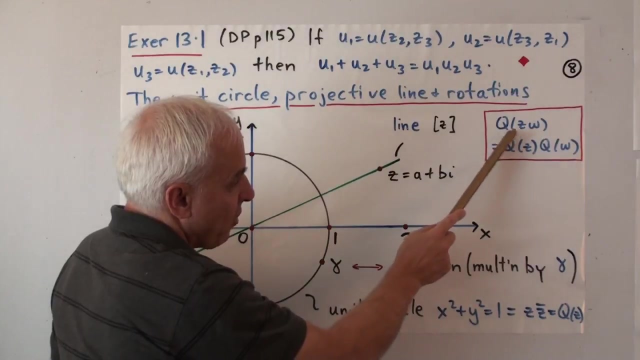 of lines through the origin, to the idea of rotations of the plane centered at zero. So these three subjects are all intimately connected. So these three subjects are all intimately connected. Now I'm going to remind you of our main theorem with quadrants, that 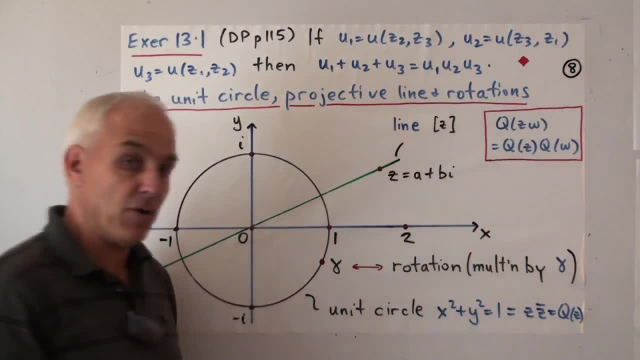 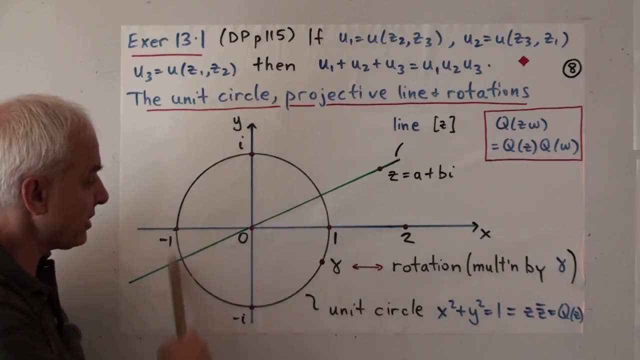 quadrants of z times w is quadrants of z times quadrants of w And in particular, if you have a point gamma which lies on this unit circle, so the unit circle has equation: x squared plus y squared equals one in xy coordinates In terms of complex. 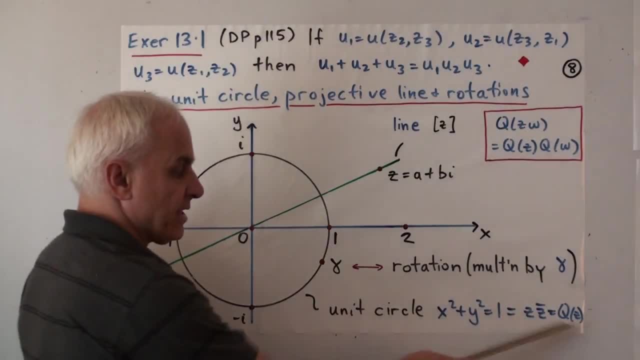 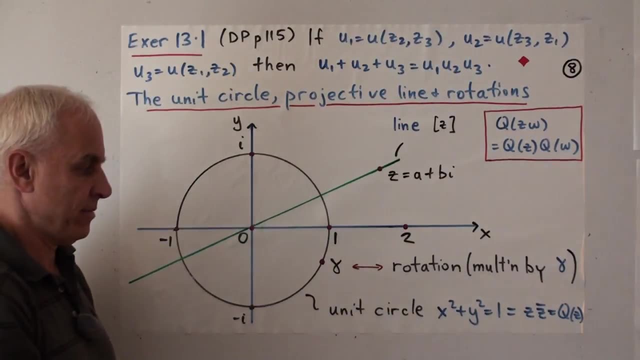 numbers. well, it's those complex numbers whose quadrants is equal to one, Or, if you like, z times z. bar equals one- Three different ways of writing down the equation of the unit circle. So suppose that gamma is on the unit circle and we consider: 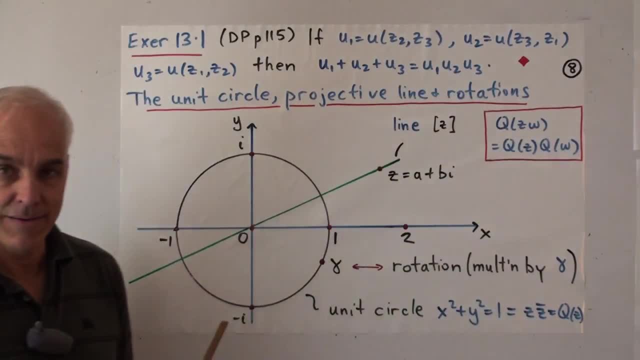 what happens if we multiply, say, w by gamma? w is out here somewhere. If we multiply by gamma, then we get the quadrants of gamma times the quadrants of w, But the quadrants of gamma is one and that tells us that the quadrants of gamma. 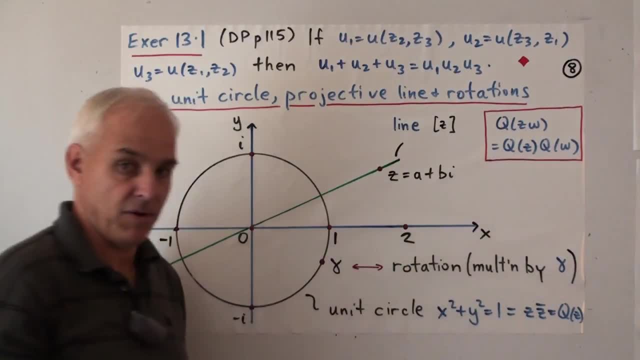 times w is the same as the quadrants of w. In other words, multiplying by gamma does not change the quadrants of a vector. So if you have a w out here and you multiply by gamma, what's going to happen is that 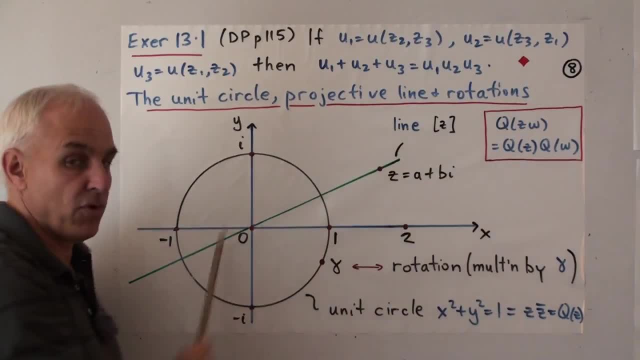 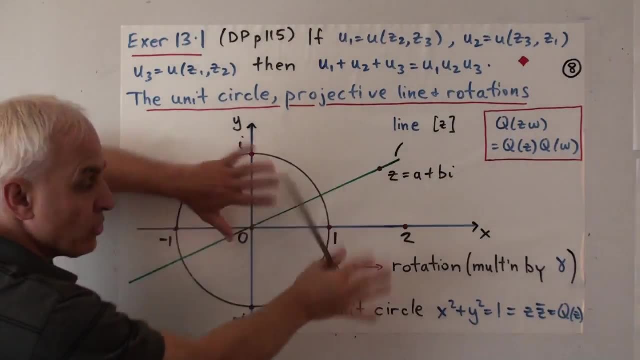 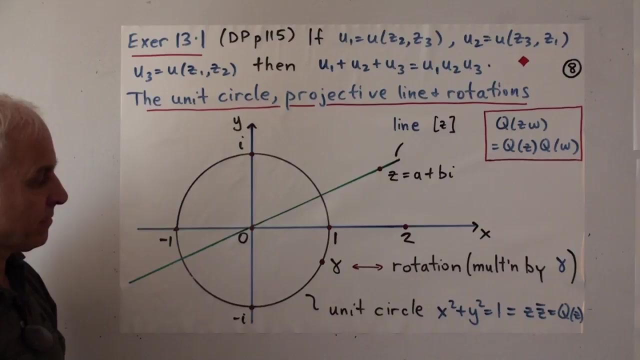 you're going to stay on the big circle through w. You're going to rotate along that circle. So multiplication by gamma is a rotation of the entire plane. So there's an intimate connection between rotations and points on the unit circle. Because, after all, if we have 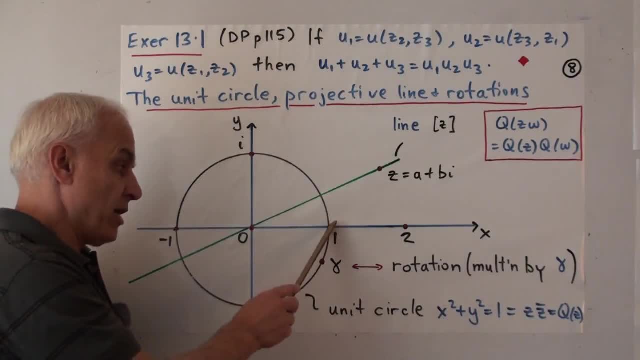 any rotation centered at zero, then this number one is going to get sent to another point on the unit circle and the rotation is determined by that point that we get. So the moral is that rotations of the plane at least centered at zero and points. 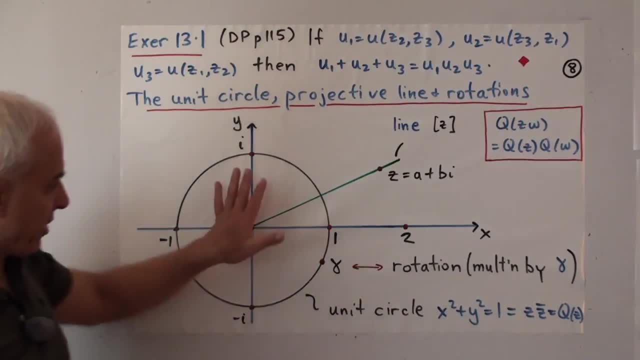 on the unit circle are intimately connected: For every rotation, there's a point on the unit circle, and for every point on the unit circle there's a rotation. Now, what's more interesting now is that we're going to throw in a third aspect: the projective. 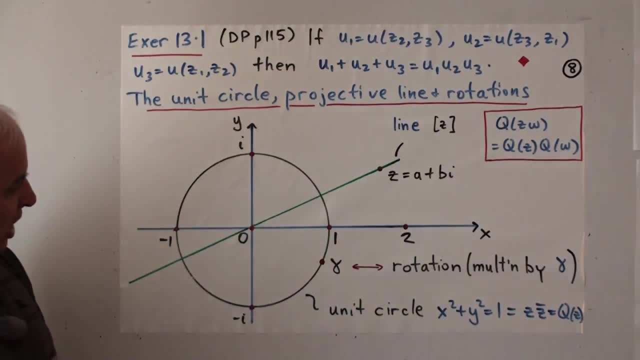 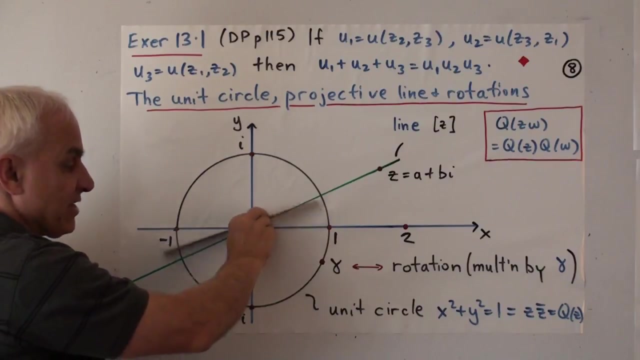 line. Alright. so in projective geometry the projective line in this kind of situation is obtained by looking at lines through the origin, That one there as an example. Or we can take any line through the origin. That space of lines is what's called the projective. 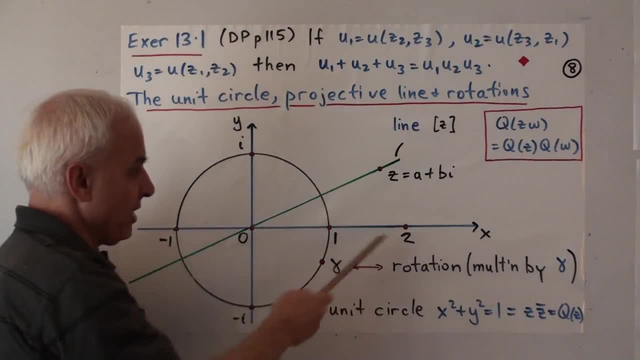 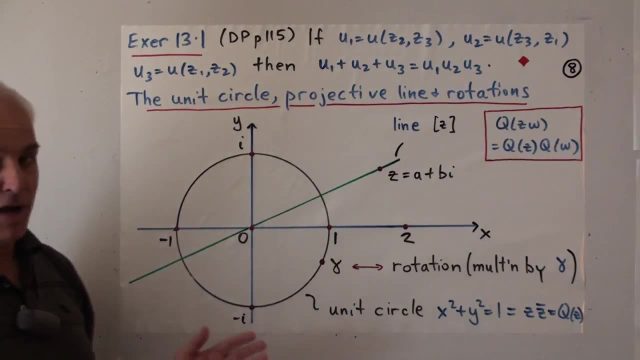 line. So here's a typical line. Let's say it goes through the point. Say that point is z, And I remind you again that all numbers are rational numbers. So a and b are rational numbers. We're only considering lines that go through the origin and a rational point. 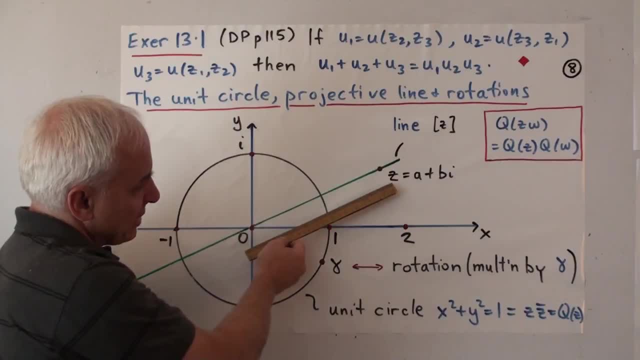 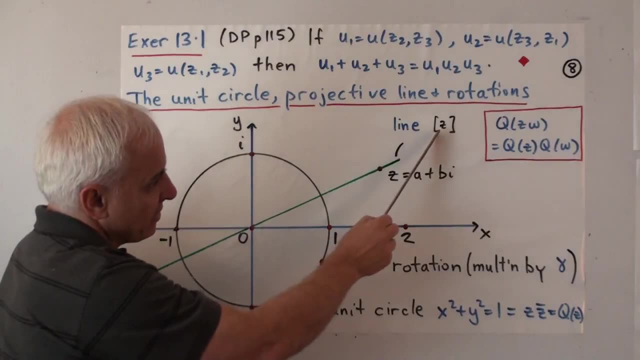 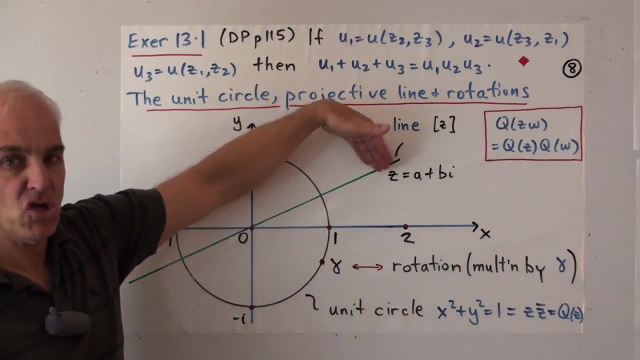 Now this line is determined by z, but it's also determined by any non-zero multiple of z. So we sometimes write square brackets of z to denote the line, meaning that we can multiply z by any non-zero rational number, and it's the same line. 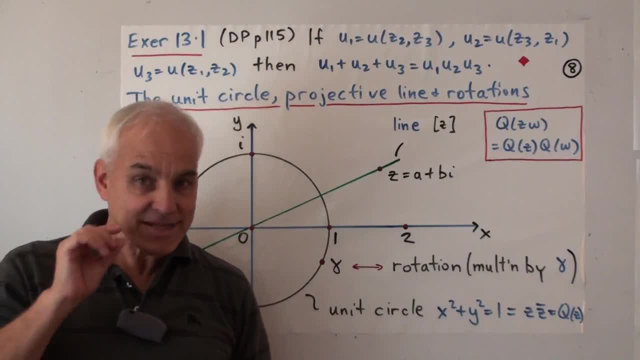 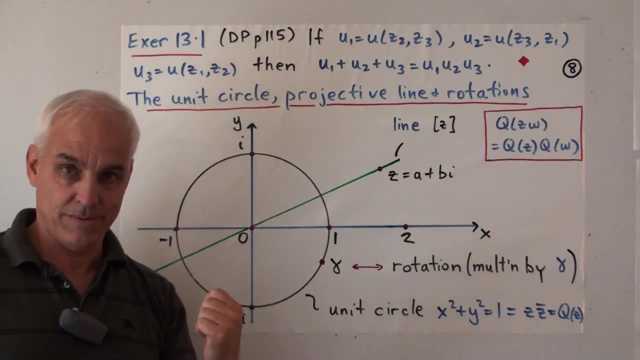 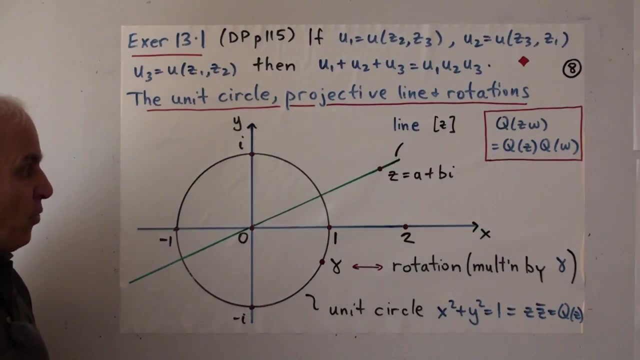 Alright. so there's a very important but somewhat subtle connection between the projective line and the unit circle. And what is it? Well, if you've been classically trained, you probably think that what you do is you take z and you divide by its. 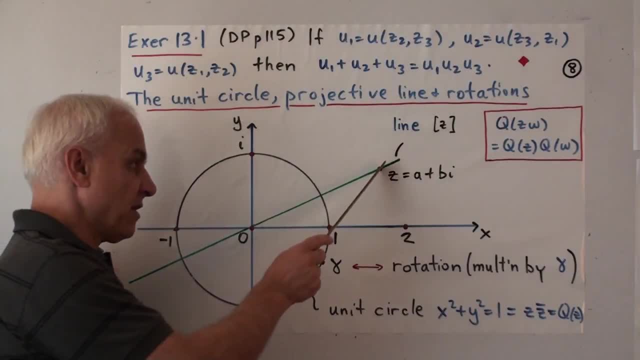 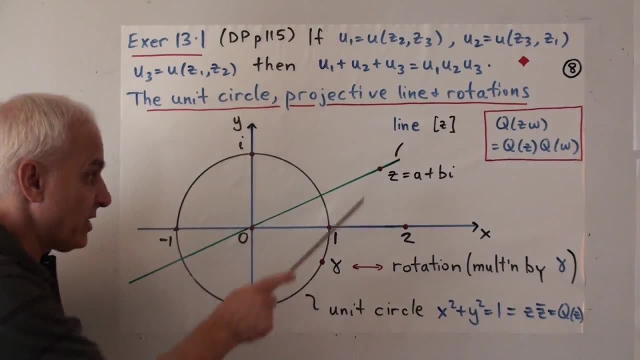 modulus. This is the standard way of getting a unit vector or a unit complex number from a general complex number. You divide by the modulus. So that means we take this and we have to divide by the square root of a squared plus b squared. 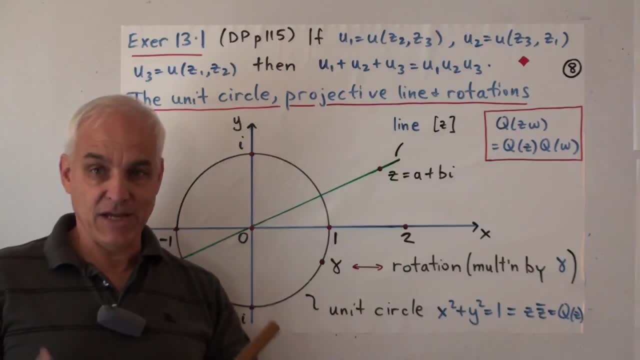 But, as I've tried to explain, the square root of a squared plus b squared is a highly problematic concept And if we're working rationally as we are here, it doesn't figure in our picture. So that's not an option for us. 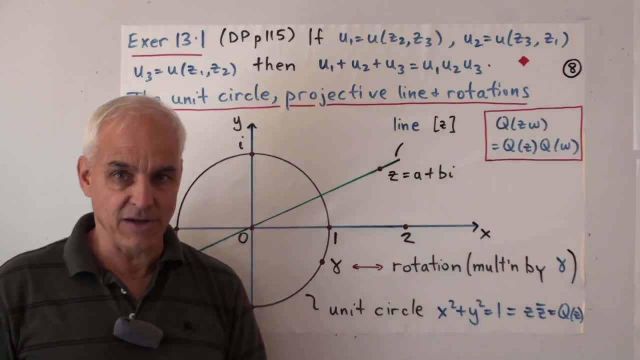 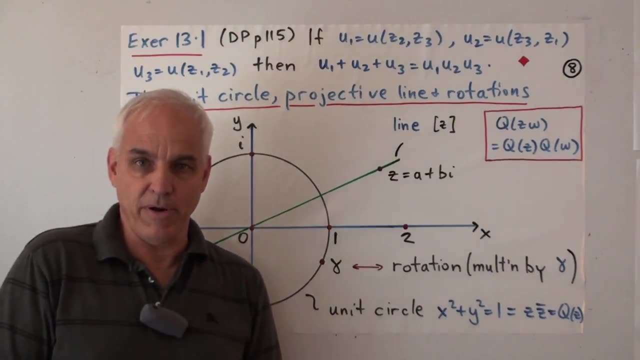 This is a very familiar construction in standard complex analysis, but it's not available to us. thinking rationally, Now you might say: well, that's a problem for you, Norman. I mean, we can do something that you can't. Well, whether you can. 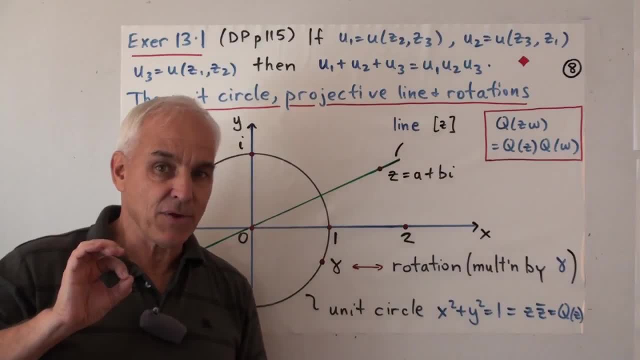 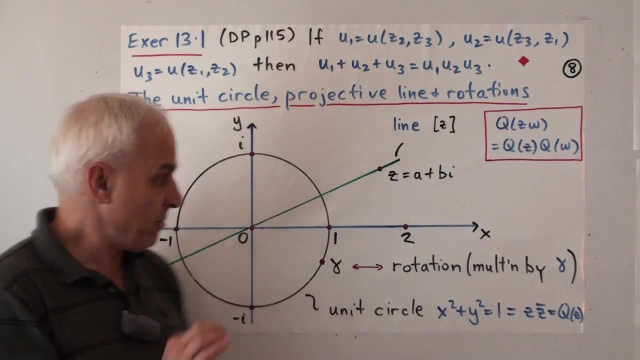 actually do it or just talk about it is a question, But the point is that there is something better that we can do to replace this idea, And it's going to be very important for us to understand what that is. It's a replacement. 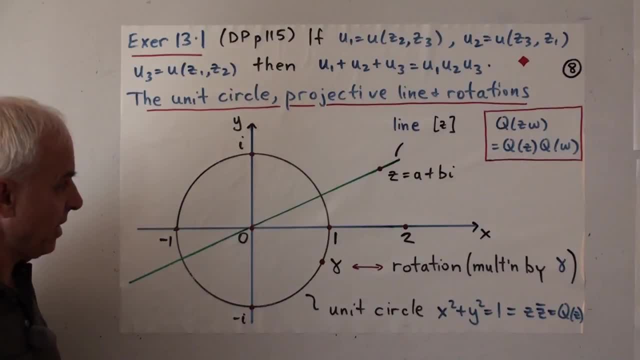 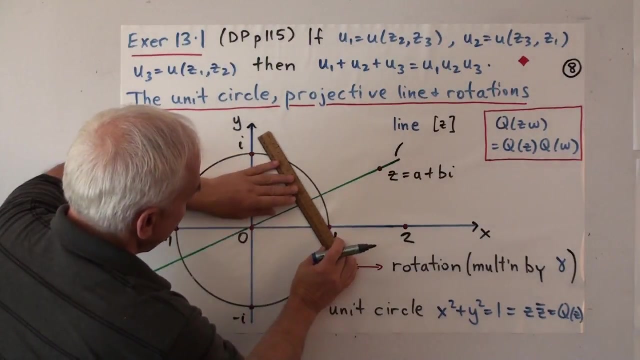 Okay. so here's what we're going to do. We are going to take this line and we're going to take the point one And we're going to reflect the point one in this line. So it's like a reflection. So how do we do a reflection? Well, we take a line through here. 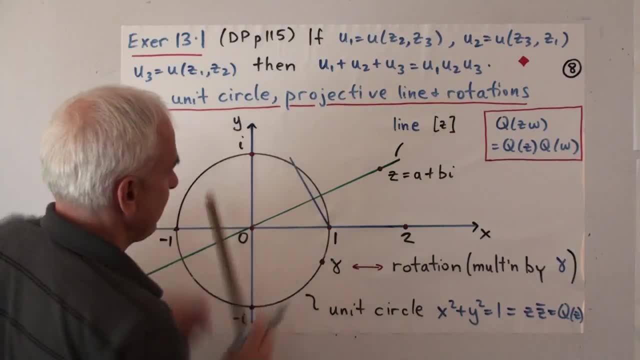 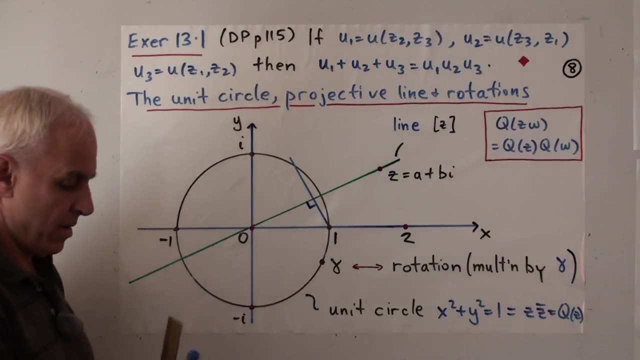 which is perpendicular, Something like that. That's perpendicular, And then we go up to here. It's going to meet the circle in the second point here, And this point here is the reflection of one in this line, And notice that it's unique. 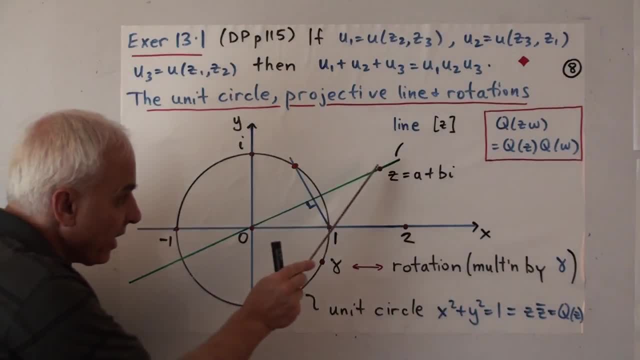 That's quite different from the idea of taking this thing and dividing by its modulus to finding a unit vector which is on this line. In rational geometry, a line through the origin does not have to meet the circle. So the existence of this point and this point, 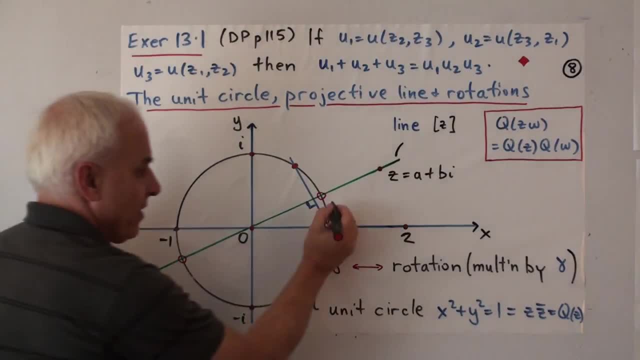 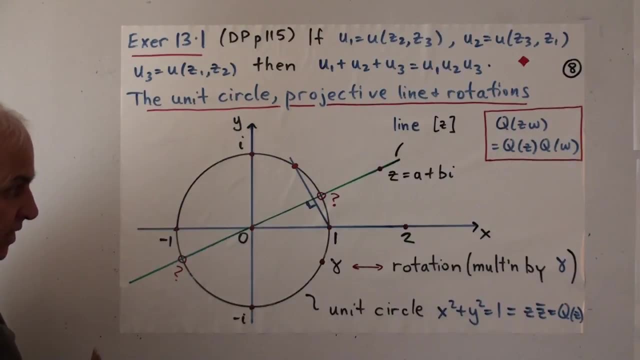 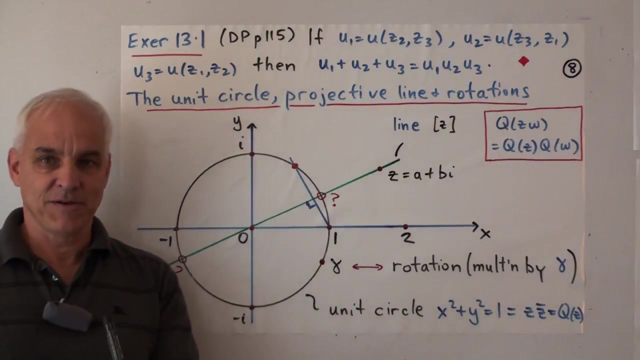 this intersection between the line and circle is problematic. Maybe it exists and maybe it doesn't. It depends on a quadratic equation determined by a and b, But this point always exists. It's there no matter what. We can always reflect this point in that point. 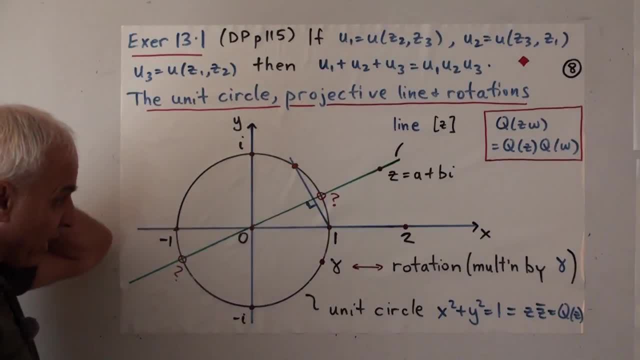 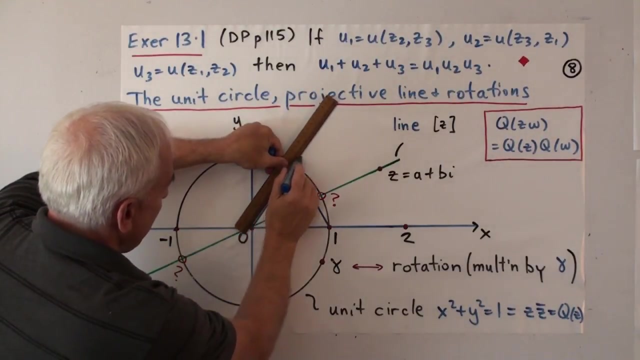 Alright. so what is this point? How can we write it efficiently? Well, it turns out there's a very nice and beautiful way of doing that, And we can see that by drawing this line here and going out a little bit further. Imagine it going out a little bit. 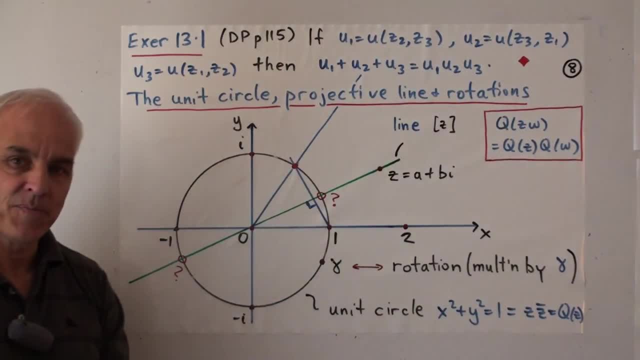 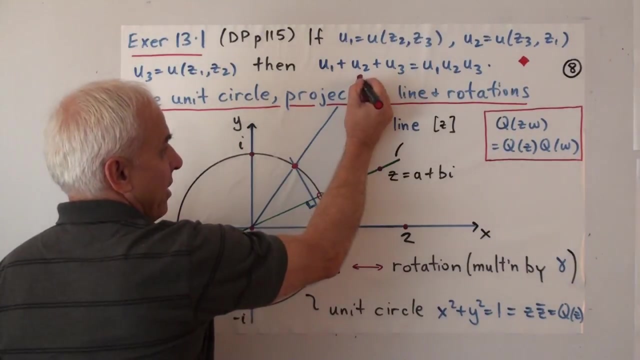 So the trick is to consider this complex number z, and to multiply it by z. Where will that get us? Well, if we multiply this by z, we're going to get z squared. It's going to be up here somewhere. Up here, somewhere is going to be. 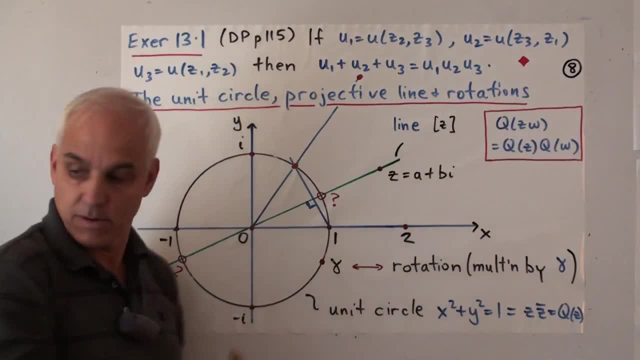 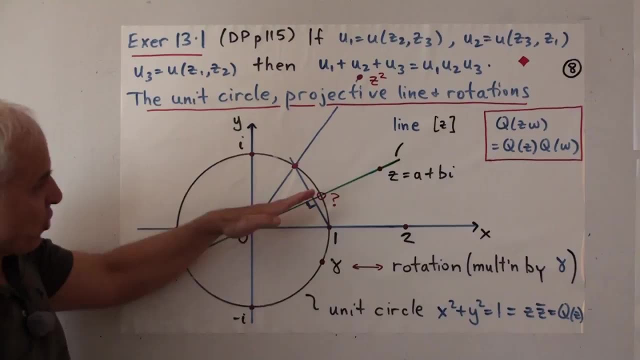 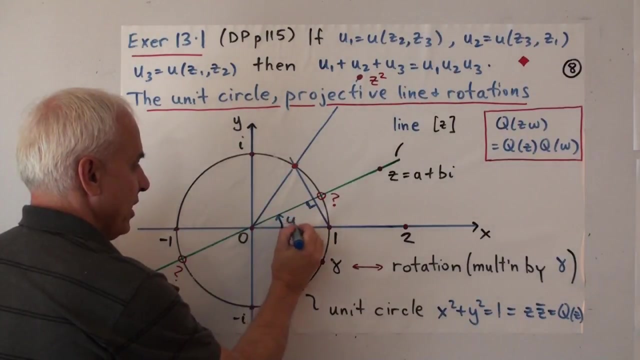 z squared. I'll put it in red so you can see it, And it's going to be up there where this turn and this turn are equal. This turn, say u, and this turn u are equal, Because multiplying by z will take 1. 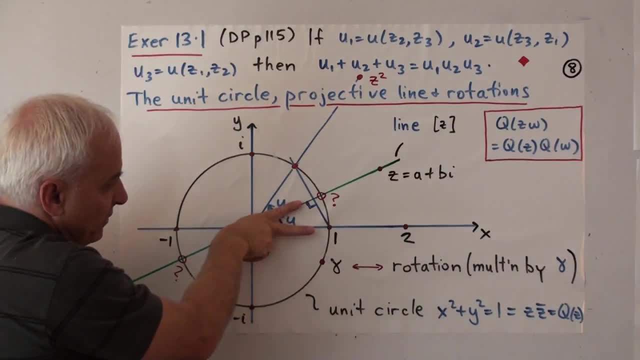 to this and will take this to this. So it preserves the turn here going to the turn there. That's the main theorem about turns. The turn between 1 and z is the same as the turn between z and z squared, And so that line is going to. 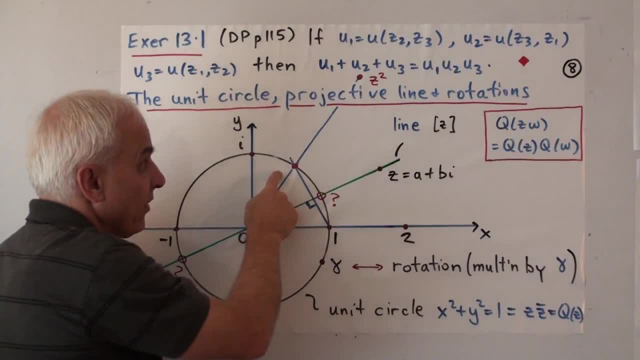 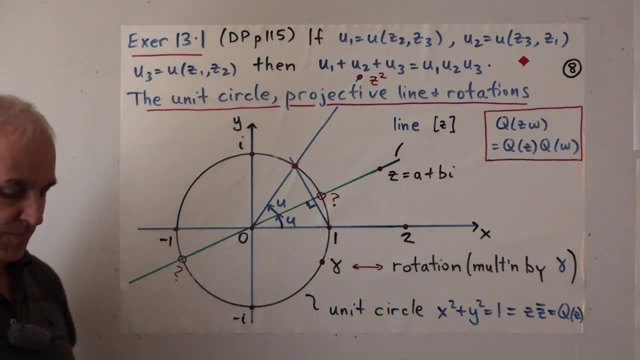 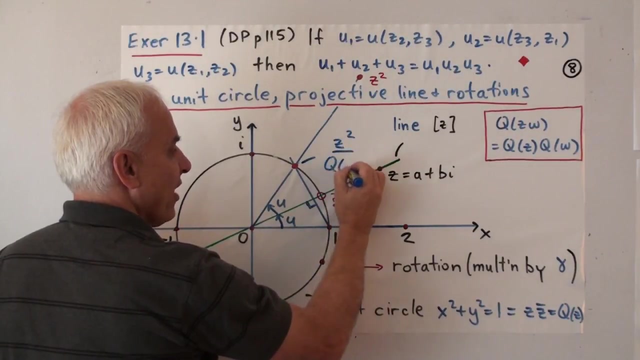 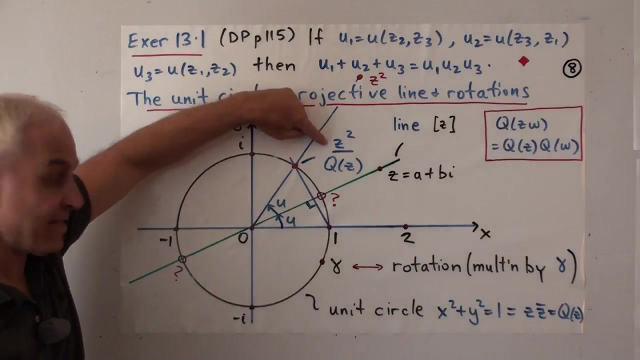 meet that point, And that point is equal to this thing divided by its quadrants. So this point here is actually z squared over the quadrants of z. It's the same kind of thing that we were trying to do here, But because this is z squared the quadrants. 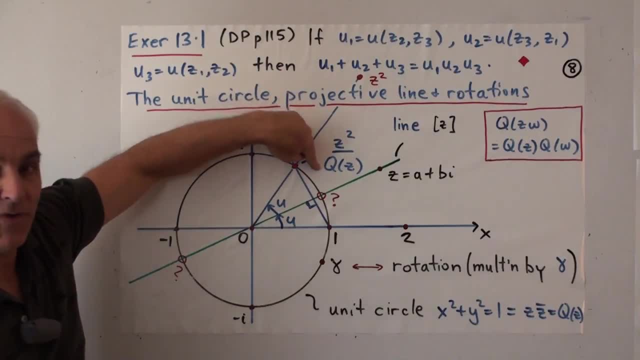 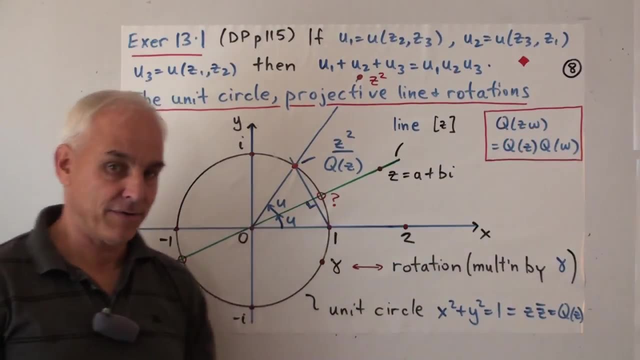 of this is the square of the quadrants of z. That's a property of this thing. here The quadrants of z squared is the quadrants of z all squared. So when we divide z squared by the quadrants of z, we're on the unit circle. 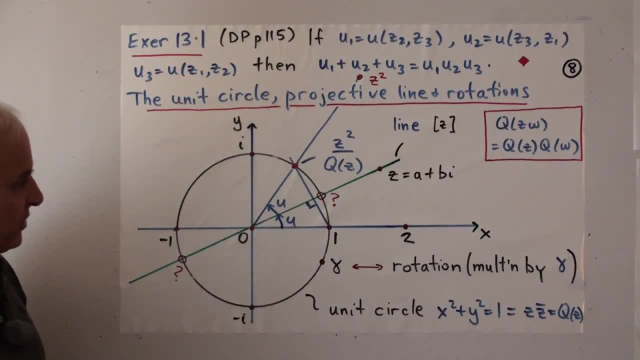 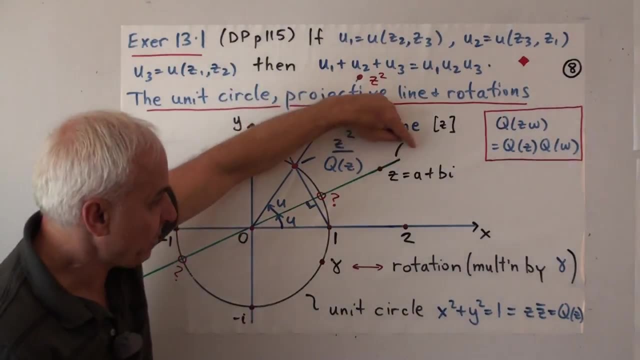 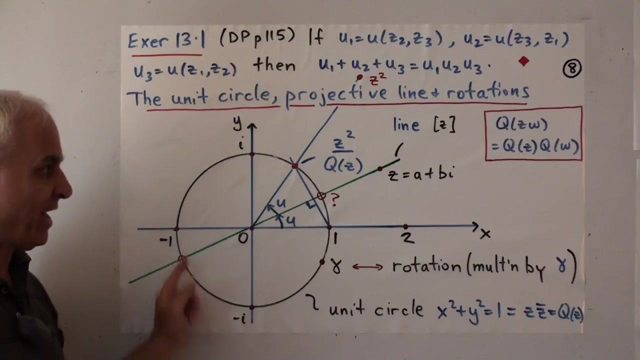 So what a beautiful thing that is. So that's a way of associating to a line a point. And if you change z by multiplying it by a scalar, multiply it by 2, or by 3, or by minus 1, this point is not going to change. 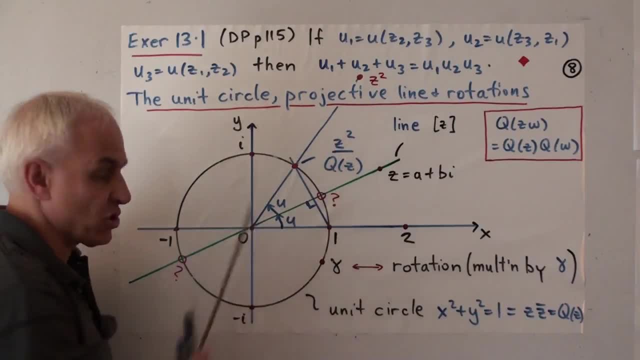 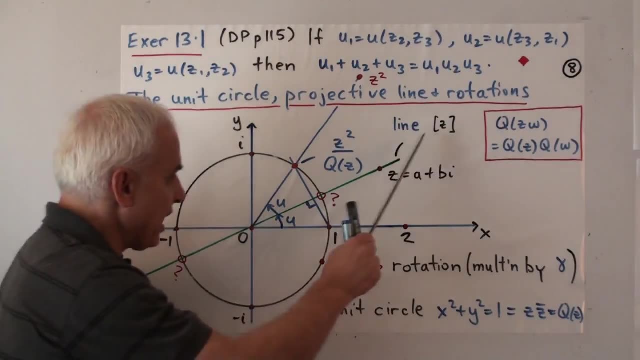 Because you multiply z by lambda, then there's going to be a lambda squared appearing up there and there's going to be a lambda squared appearing down there and they're going to cancel. So it doesn't matter what z you choose on that line. 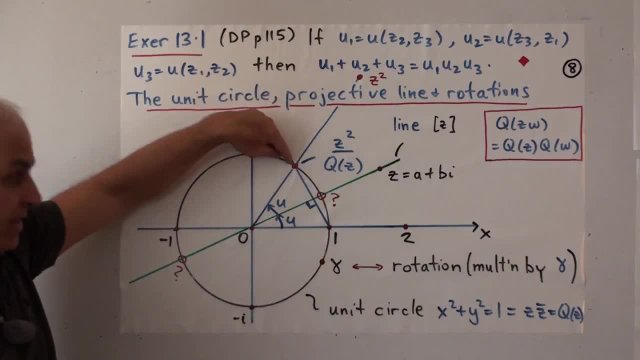 you perform z squared divided by q of z, you're always going to get that point. This is a very important idea. It's somehow at the heart of a certain 2 to 1-ness which appears throughout this subject And it's often considered a feature of the quaternion business. 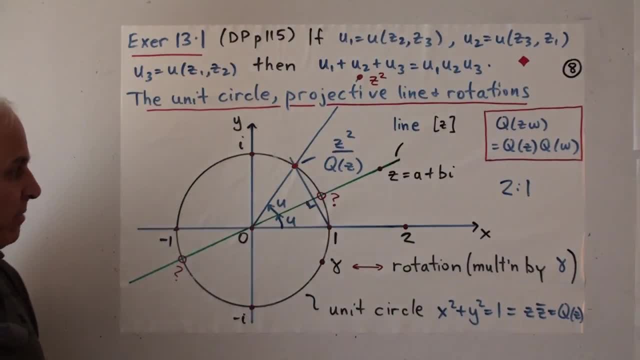 but you should appreciate that it's already existing here in the complex numbers That if we want to associate a rotation to this line, the way to do it is to associate to it the rotation by z squared over q of z. Very good diagram to spend a couple of hours staring at it and to think about it. 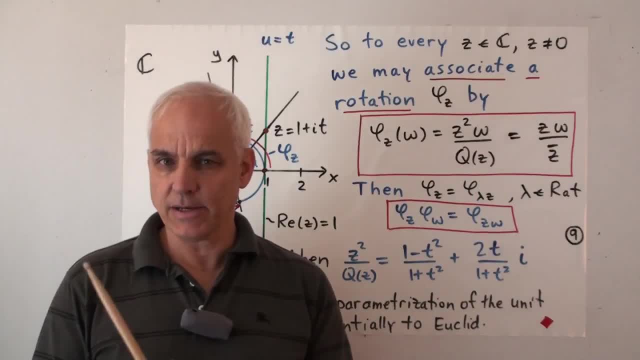 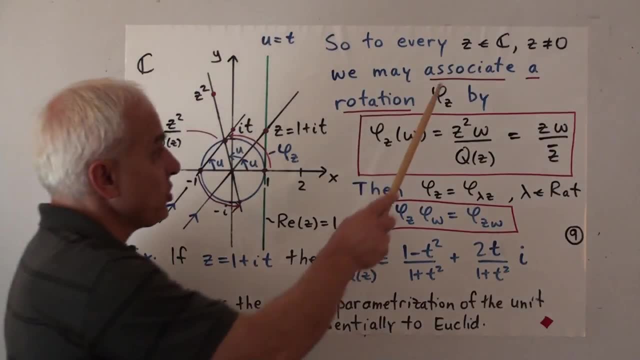 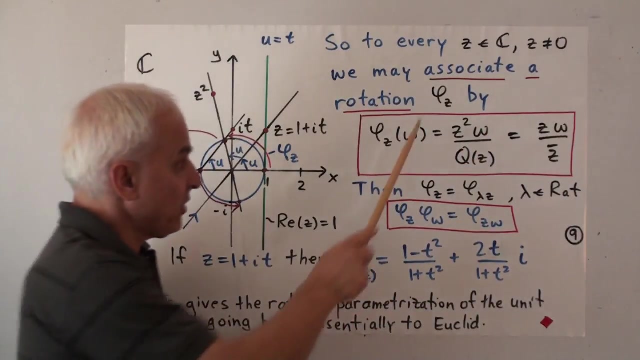 So let's try to understand this structure by looking at a sort of special case. But first let's identify that what we've managed to do is to associate to every complex number z which is non-zero, a rotation. Let's call it phi sub z, where 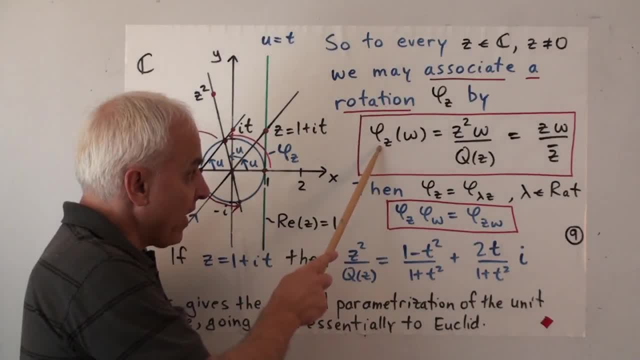 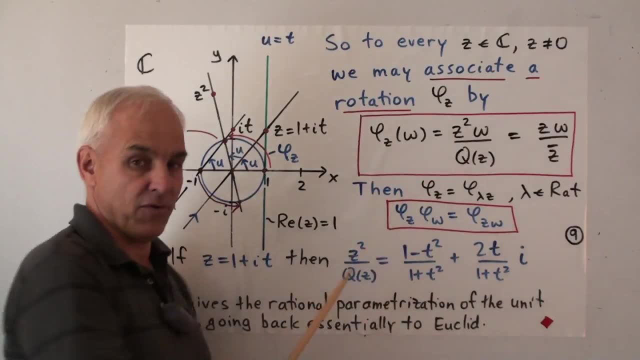 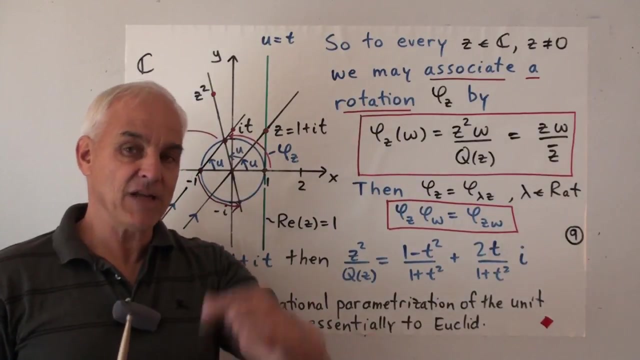 its rotation is defined as follows. It's defined as phi of z acting on a complex number. w is multiplying w by z squared over q of z. Because z squared over q of z is a unit complex number, It lies on the unit circle, And so this is. 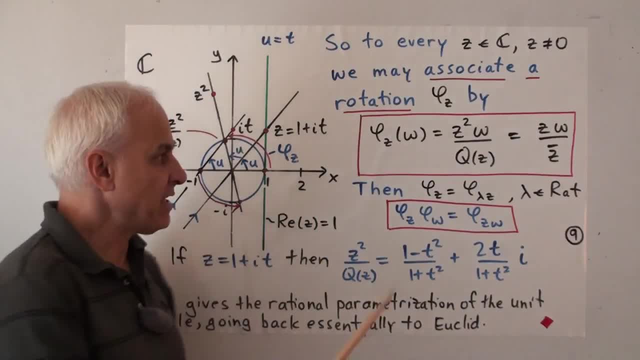 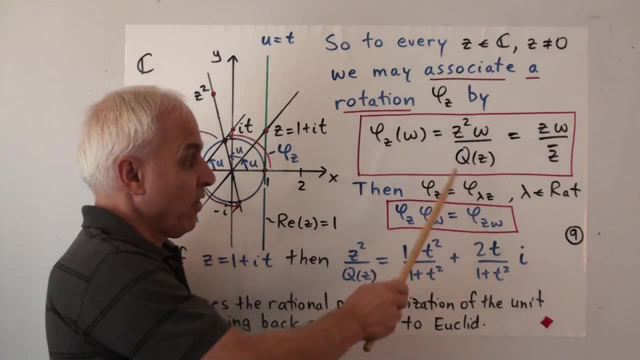 necessarily a rotation That depends on z. I'll just mention that there's another nice way of writing it. Remember that q of z was equal to z times the complex conjugate z bar, And so if we write it that way, then two of the z's on top and bottom. 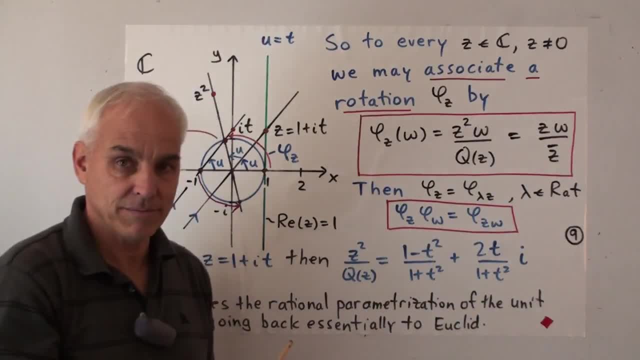 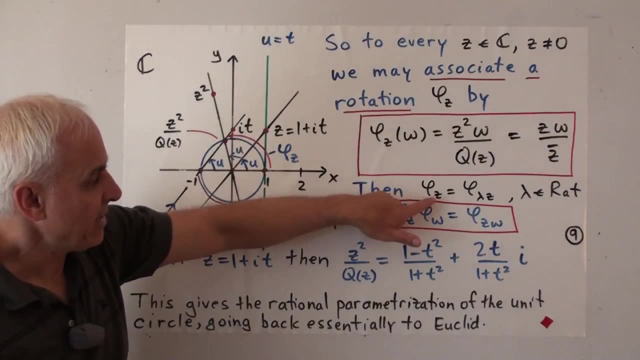 cancel And we can write it as z times w over z bar. That's another way of writing it, So that's quite nice. and it has the property that if you multiply z by a rational number, then the rotation doesn't change. So the rotation. 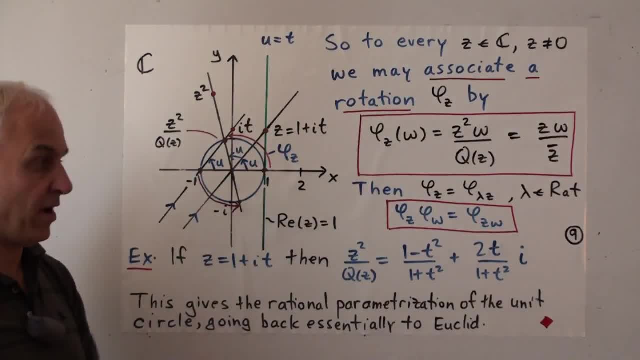 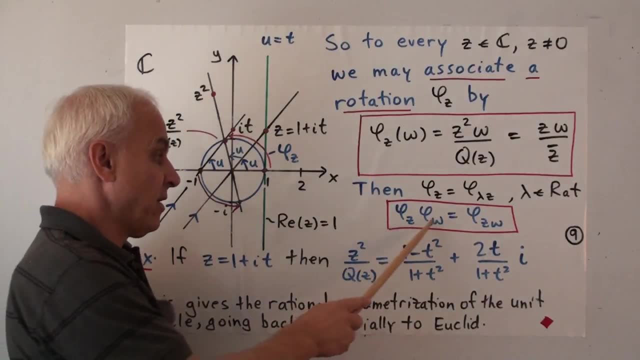 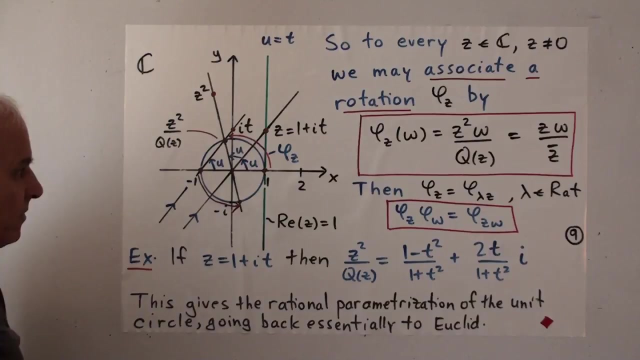 only depends on the line, through the origin, through z, And you can also check as a nice exercise that if you compose two rotations, phi of z, phi of w, that's the same as phi of z times w. Now I want to connect that. 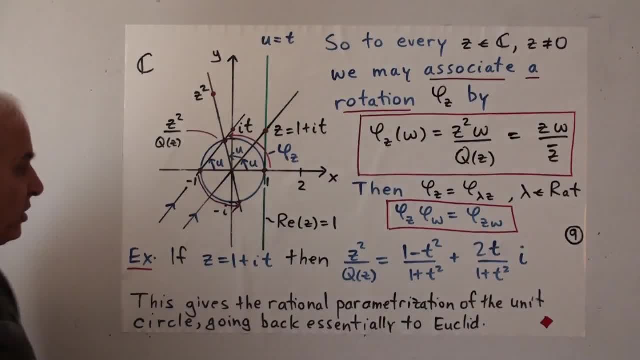 circle of ideas with a very classical subject which is close to my heart, which I've mentioned in quite a few of my videos. It's a very important thing that all undergraduates should be well aware of, And that's the rational parameterization of the circle. 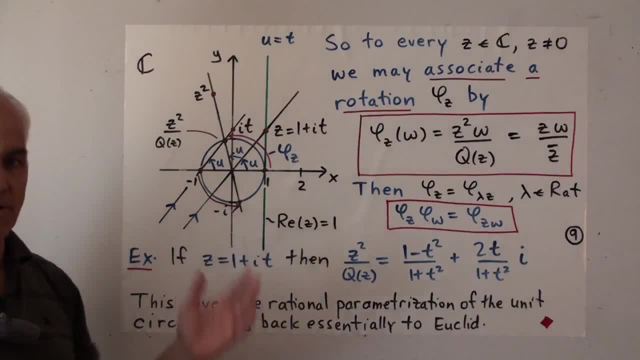 And in fact that really drops out from looking at what we've just done. So a bit of complex analysis allows us to rethink this rational parameterization in a very pleasant way, And the idea is that, well, let's say we're interested in. 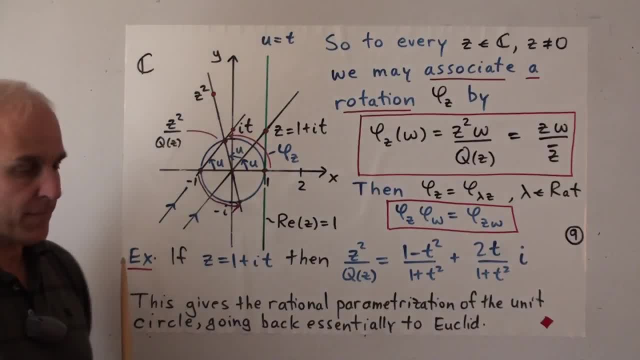 lines through the origin. The space of lines through the origin can be described as essentially a line plus a point at infinity. So if I take this line here, this green line which has equation real part of z equals 1.. So all the complex numbers on 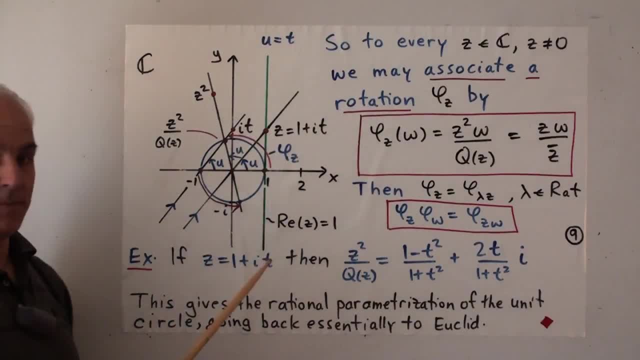 here are of the form: z equals 1 plus i, t, where t is some number. If we take any one like this, then the point on it join it to the origin, we get a line, And all lines through the origin are of that form. 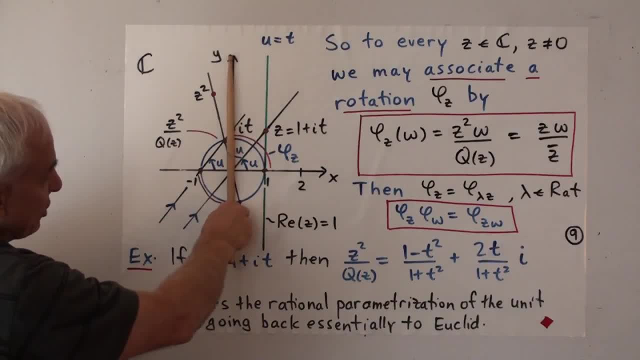 for some t, except for the sort of special case where we're just looking at this parallel one, which is sort of the case when t is infinite, But otherwise all lines meet this green line in exactly one point. Let's call it 1 plus i t. Alright, now that's a rather interesting point. 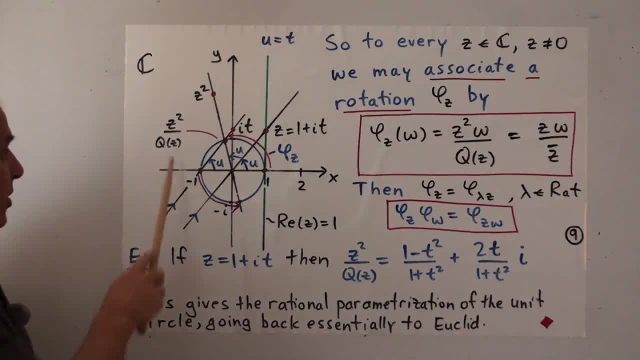 Let's have a look at what happens if we do this construction that we talked about, where we calculate z squared over q of z, When z happens to be the special complex number 1 plus i t. So if z is equal to 1 plus i t, then z squared over q of z. 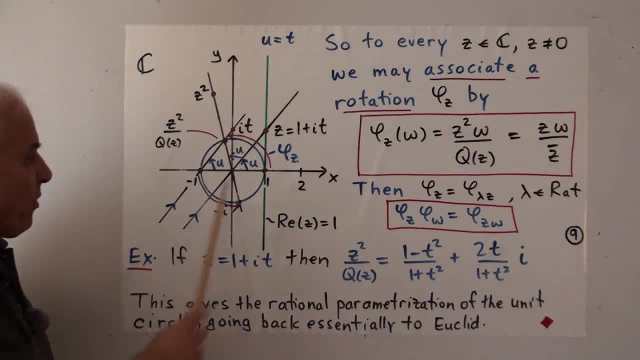 What is it? Well, first of all, what is z squared? z squared will be 1 minus t squared plus i times 2t, 1 minus t squared plus 2t times i. But we have to divide by q of z. 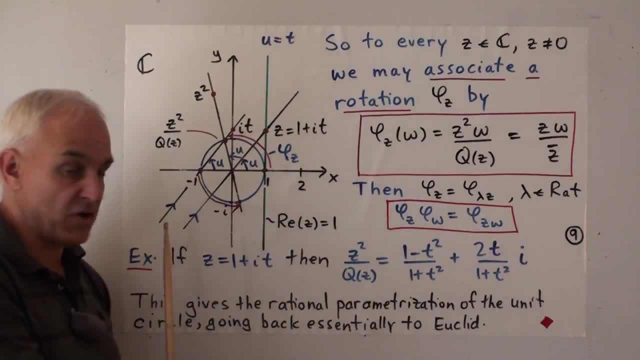 What's q of z? It's the sum of the squares of the coefficient, So it's 1 plus t squared. So we get 1 minus t squared over 1 plus t squared, plus 2t over 1 plus t squared i. 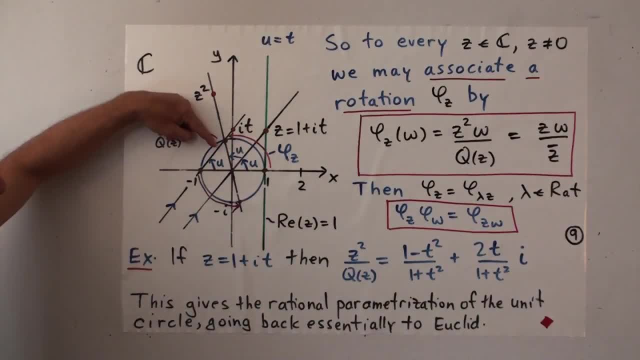 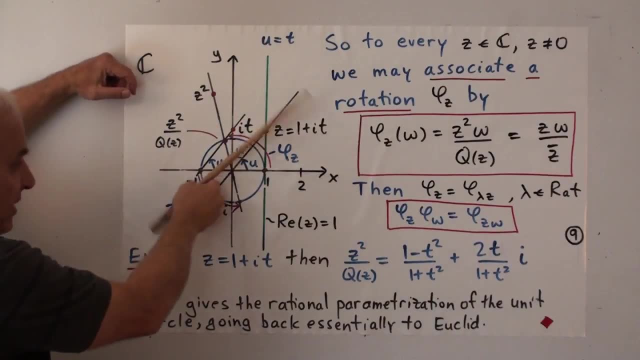 And we know that that's a point on the unit circle. And, moreover, it's exactly the point that we get by doubling this angle, if you like, or taking this turn and applying an equal turn to it. There, it is right there. So, while z squared is up here, 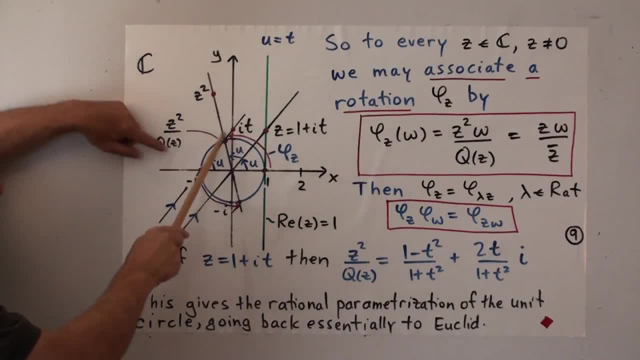 generally, then dividing by q of z, scales it down so that it gets on the unit circle, And this point is also the reflection of the point 1 in this line. Now, this is the familiar rational parameterization of the unit circle that goes back essentially. 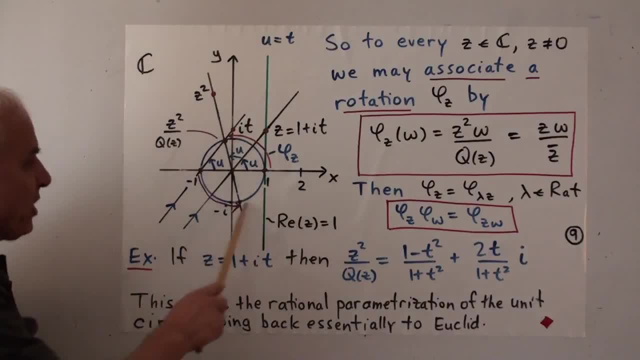 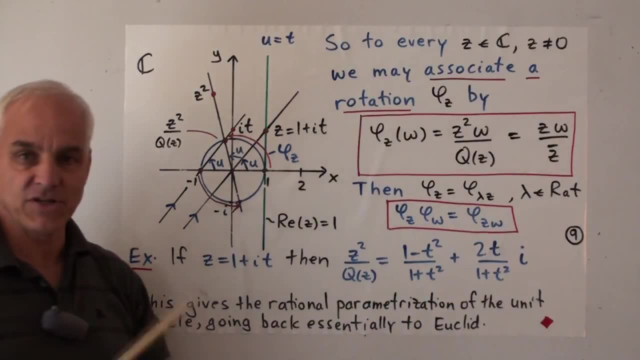 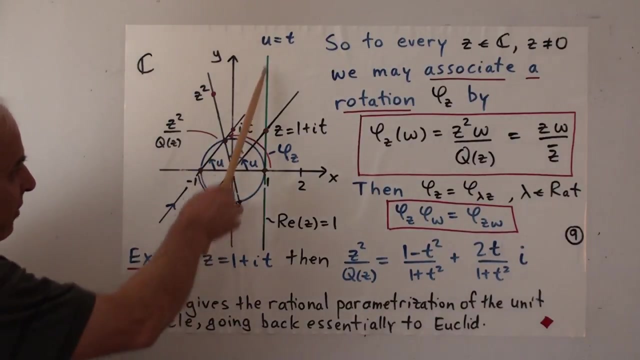 to Euclid. Every rational point on the unit circle is exactly of this form. That's the x coordinate, That's the y coordinate For some rational number t, Except for the special case when you have minus 1, which sort of corresponds to t equals. 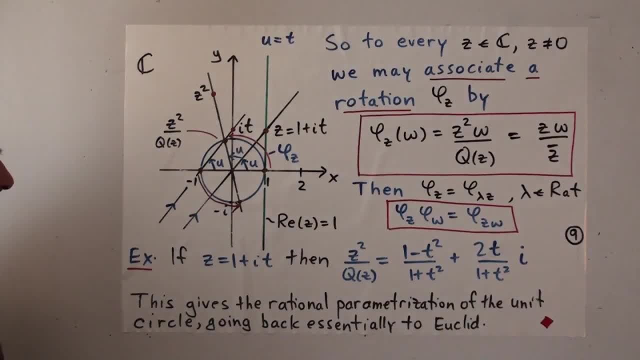 infinity. There's a few other things I would just like to mention about this which are interesting too. The other property is that if you take the line from minus 1 to this point, z squared over q of z, that that's actually parallel to the line that we started with. 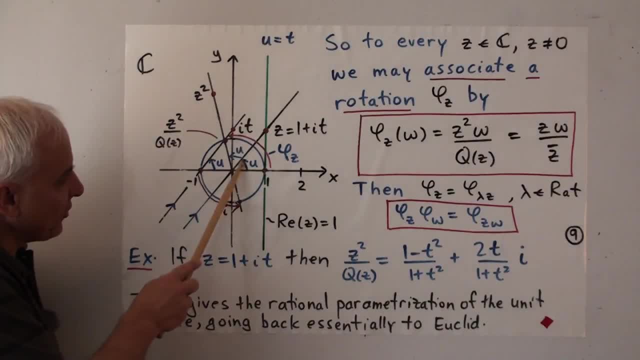 Why is that? Well, it's because here you see, that's u, That's a turn of u and that's a turn of u, And so this turn subtended by this chord at the center is related to this turn subtended by that same chord at the circumference. 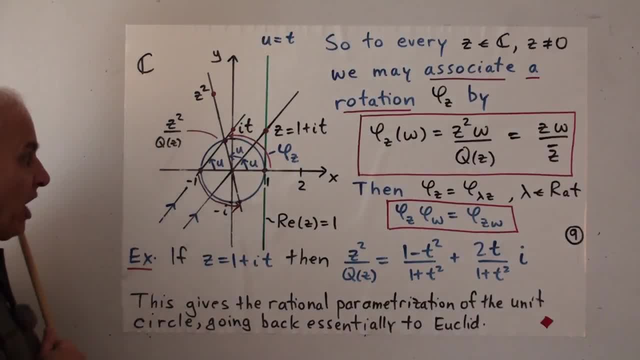 That's going to be a turn of u as well. Elementary geometry of the circle. So this line is actually parallel to this line, And if we just move everything over by 1, then the point 1 plus i, t, if we translate it over by 1, it just becomes: 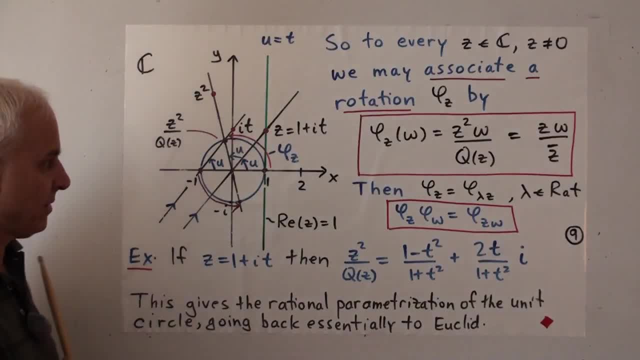 the point i, t, And so the meaning of t- if you like you can think of it here- is: it's the point on the y axis that you need to choose and then connect it to minus 1, and then that line. 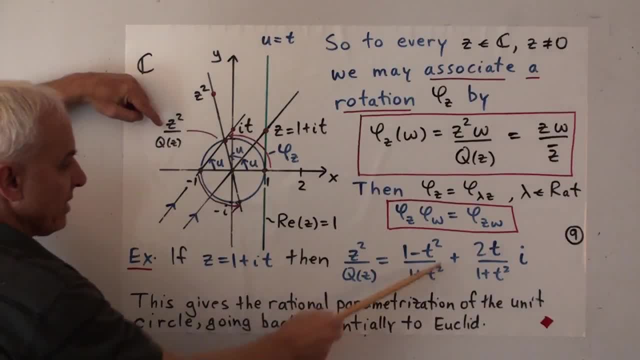 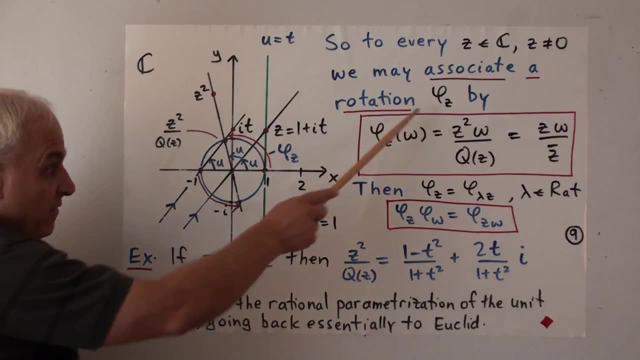 will meet the unit circle at this point: 1 minus t squared over 1 plus t squared, 2t over 1 plus t squared, And then connecting things with the rotation phi of z. once we have this point on the unit circle, associated to that is the rotation. 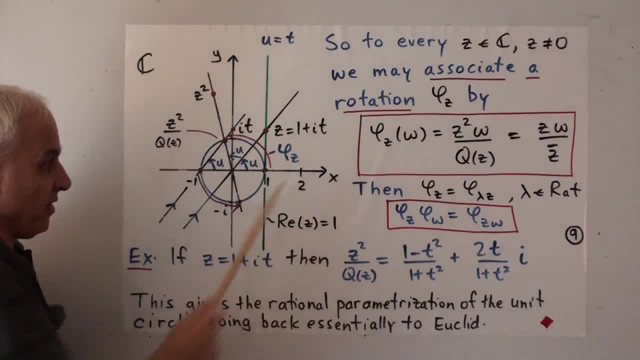 multiplication by that point. That's what we're calling phi of z And that's the rotation that physically takes point 1 and rotates it to that point there, Takes this point and rotates it to there, So it's rotation like that. That's the rotation phi. 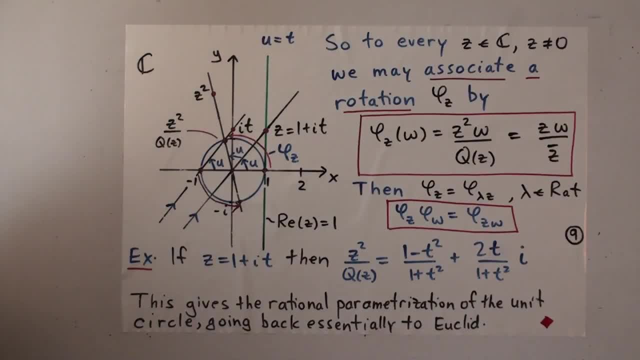 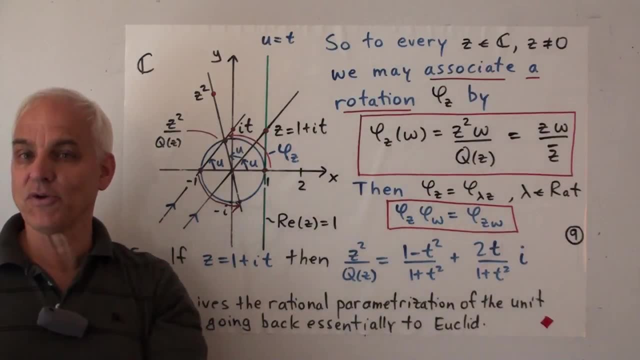 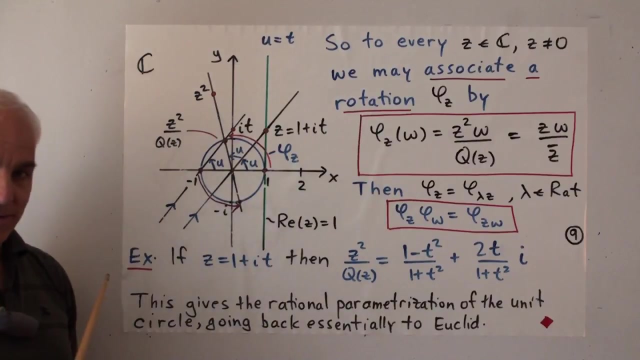 of z And, for future reference, I'd like to also remind you that that rotation can also be thought of as a product of two reflections. Alright, so there's this line here, and then there's this line here that we're considering If we take the product of the reflection. 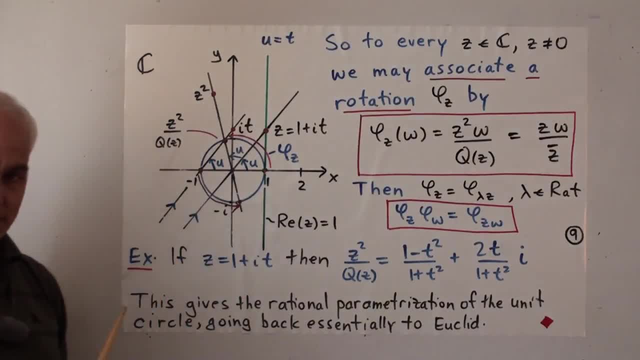 in this line, followed by the reflection in this line. what do we get? Choose some point here and you reflect it first in the x axis and then you reflect it in this line here. you're going to get a point here which is the same as the. 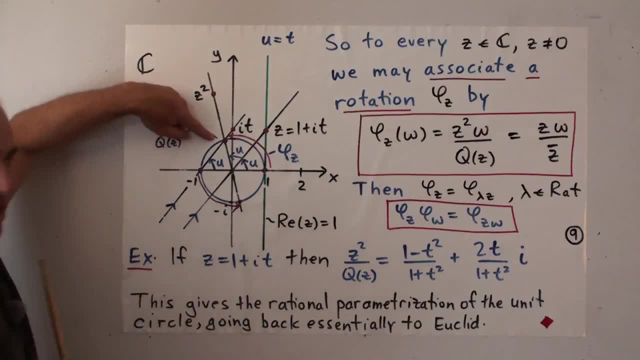 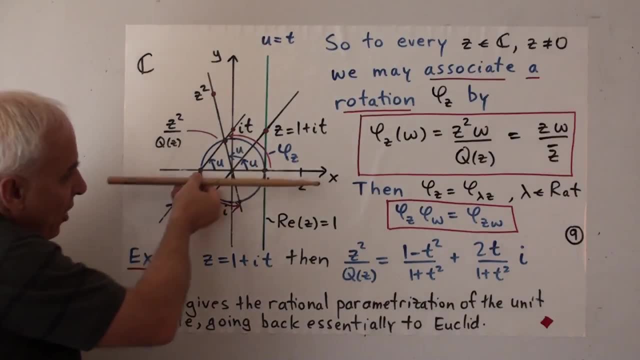 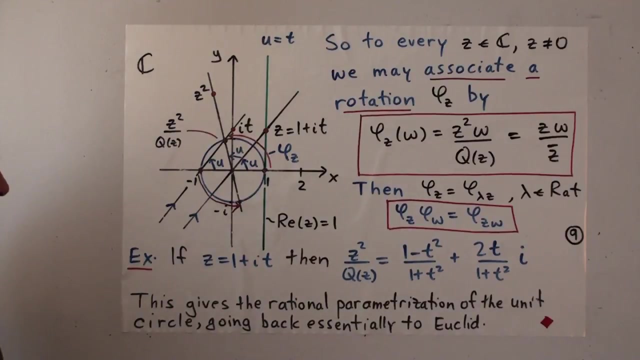 rotation of the original point phi of z. So this rotation determined by this unit circle is also associated to this line in another way. That is basically the product of this reflection times, this reflection Alright, so there's quite a lot of material. If you haven't seen complex numbers before, of course it will probably. 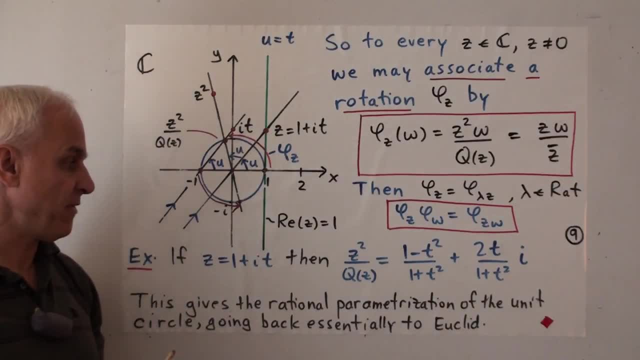 be overwhelming to you If you have seen some complex numbers before. I hope this provides a somewhat different view on things And this 2 to 1 aspect is going to be very important for us when we try to understand quaternions, So this is a very good thing to try to understand. 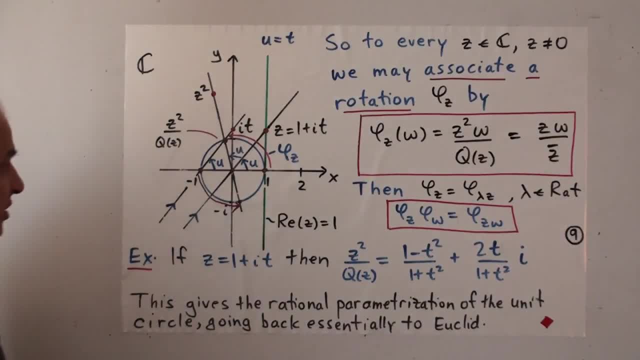 first, It makes understanding quaternions so much easier. As good practice for you, you might like to calculate the turn associated to the vector, say, and this unit vector that we found here. So in other words, the turn u, this turn here is t, because that's t and that's 1.. 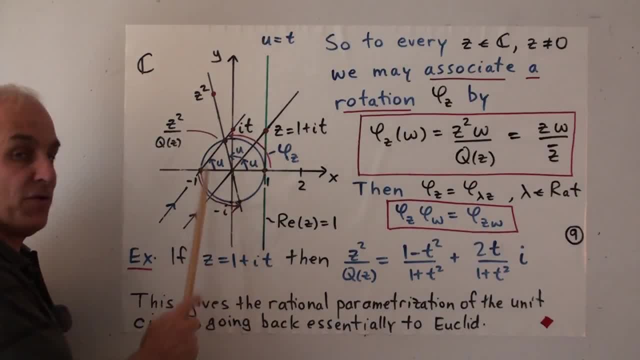 So the slope is t. So if that's a turn of u and that's a turn of u, then what's the combined turn from here to here? In fact, you can think about what happens if you combine more turns of u's: 3 turns of u, 4 turns of u. 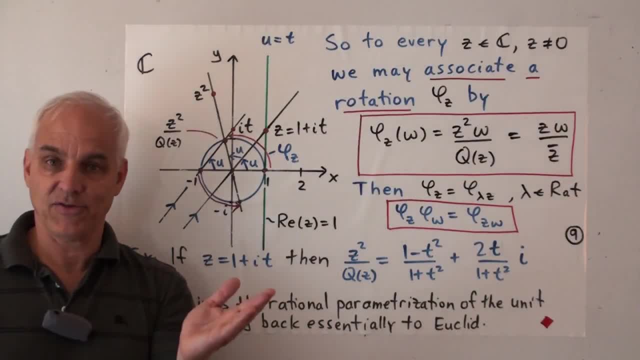 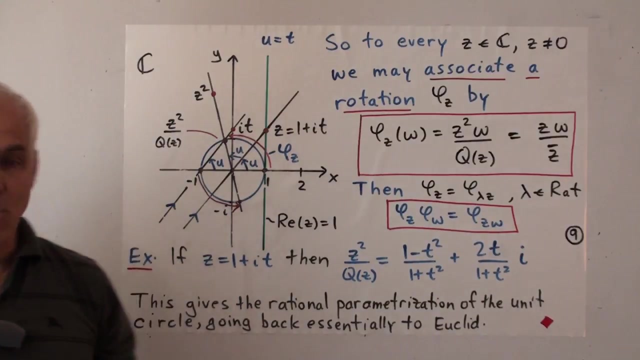 and so on. What is the turn of the composite turn? It's a very nice little formula And of course we all want to do that without any transcendental functions, no circular functions, no mention of angles. So in our next video we're now going to go up to 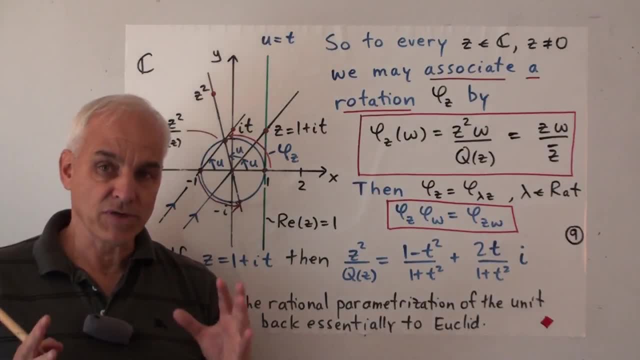 3-dimensional space and start discussing rotations, The problem of rotations. How do we describe rotations in 3-dimensional space And, in particular, how do we compose rotations? I hope you'll join me for that. I'm Norman Wahlberger. Thanks for listening.